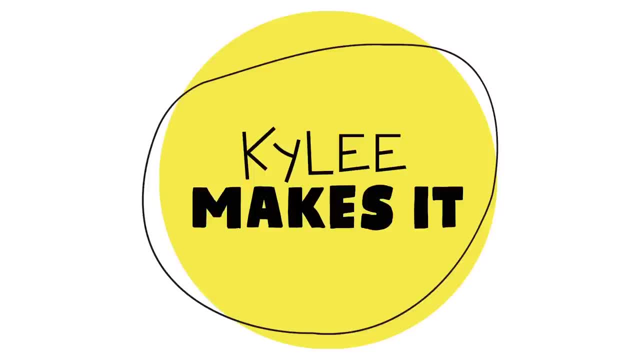 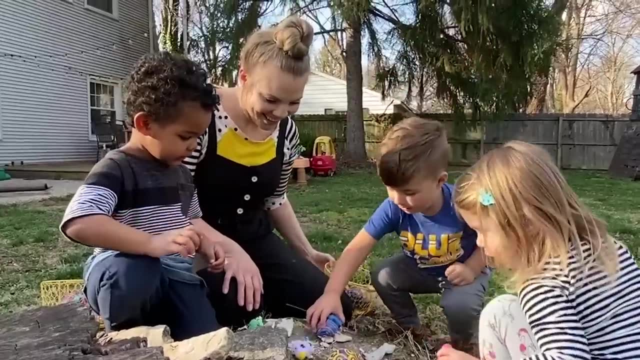 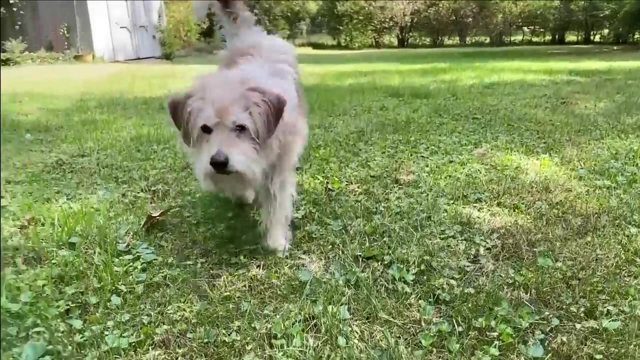 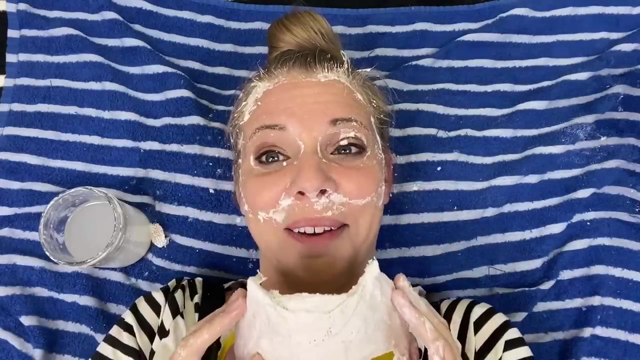 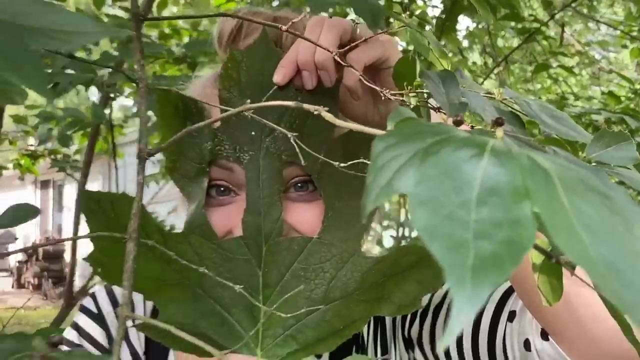 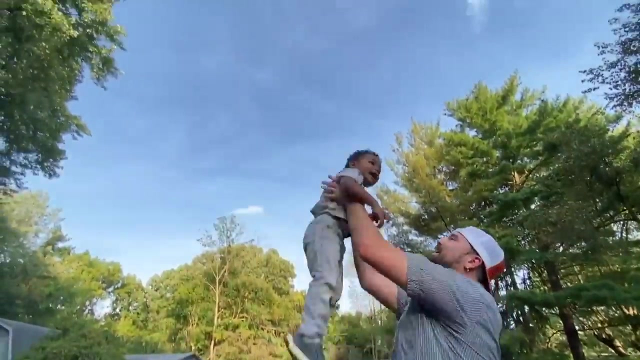 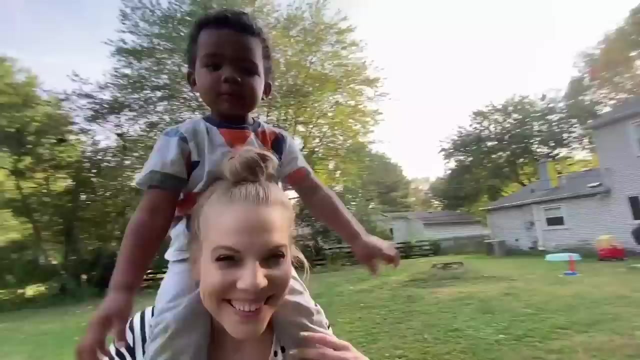 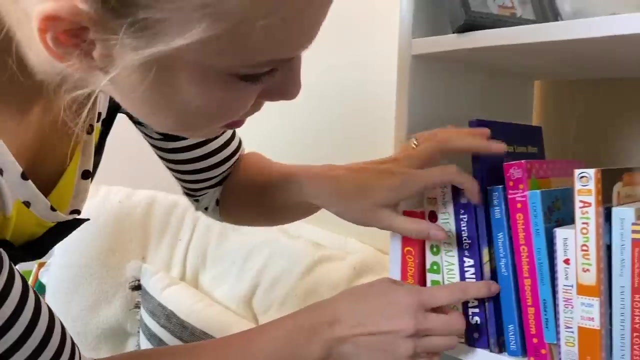 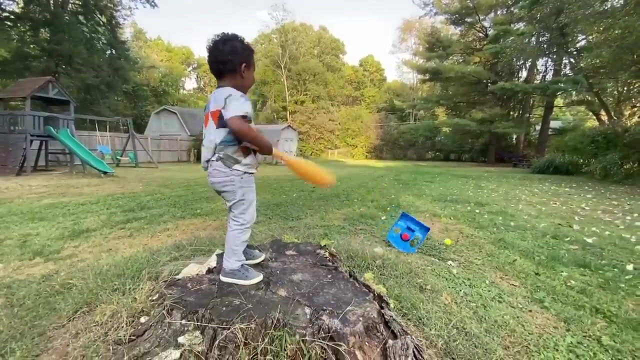 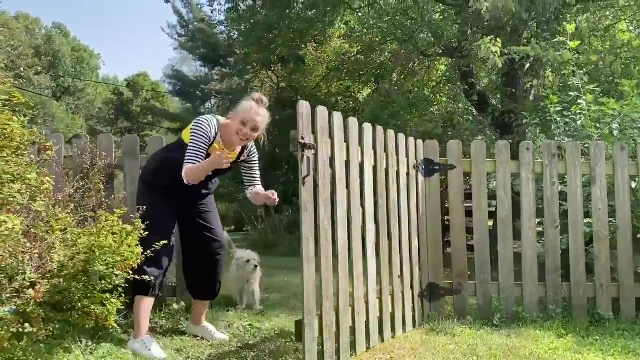 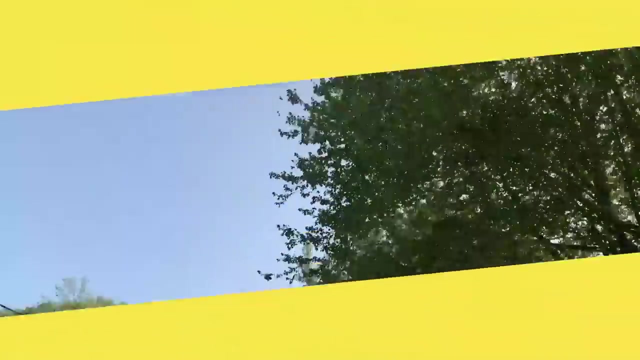 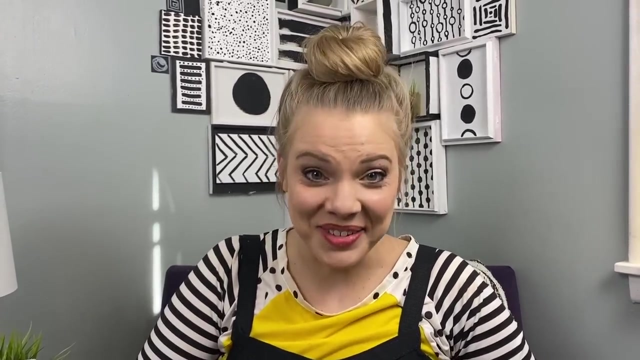 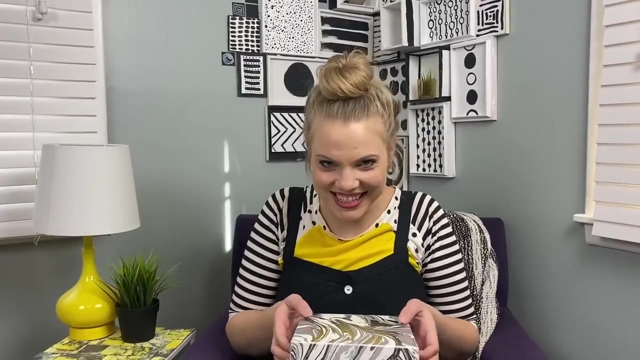 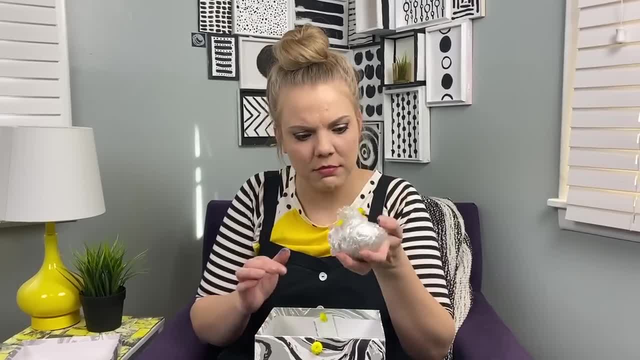 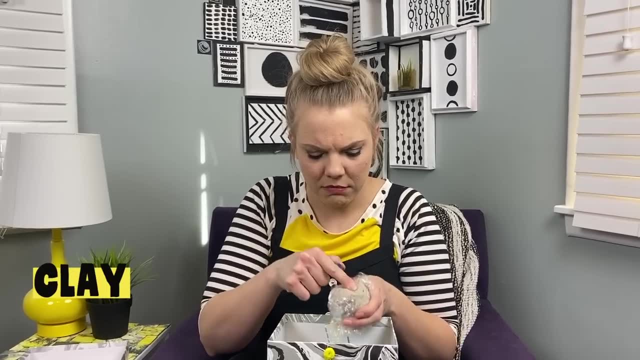 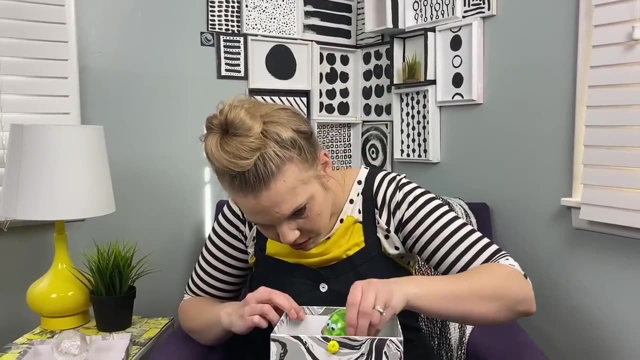 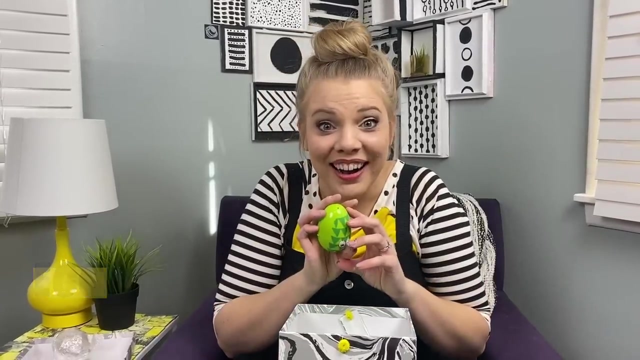 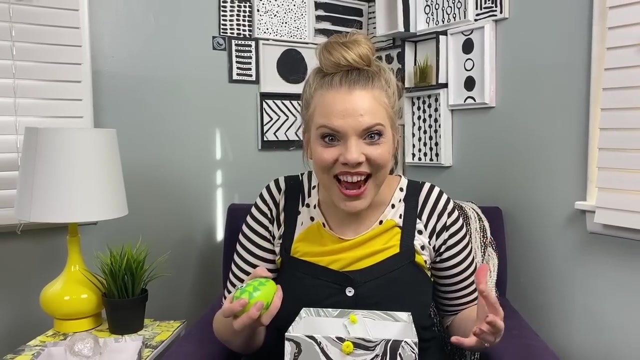 Coming up on Kylie Makes It surprise eggs So fun to make, so fun to break. Coming up on Kylie Makes It surprise eggs So fun to make, so fun to break. People hide them outside and when you open them up there's all sorts of surprises in there. 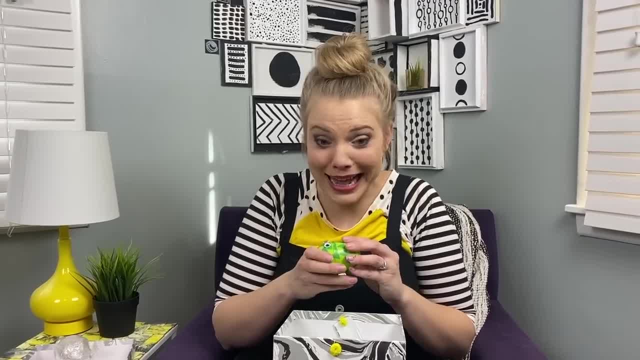 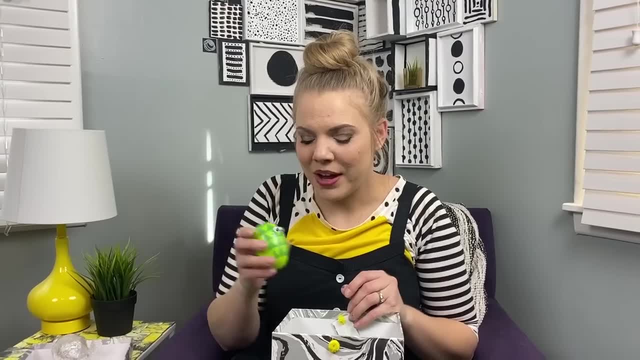 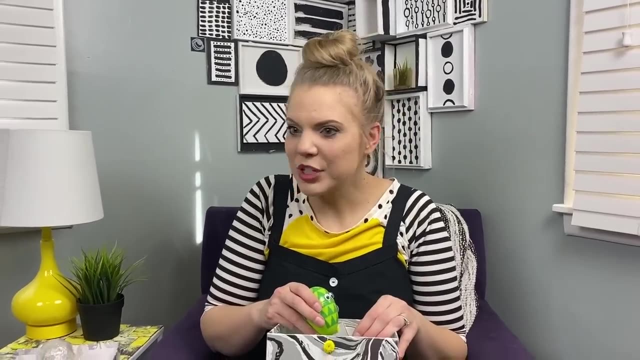 It could be candy, toys, stickers, money, anything I love. surprise eggs. I don't know what that clay is about, but, um, you want to go on an egg hunt with me? Let's do it. I wish there was a basket or something around. 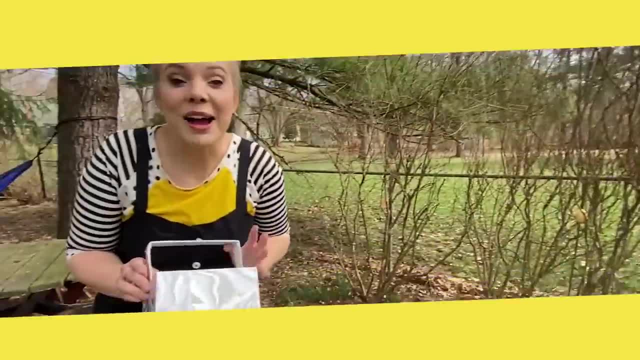 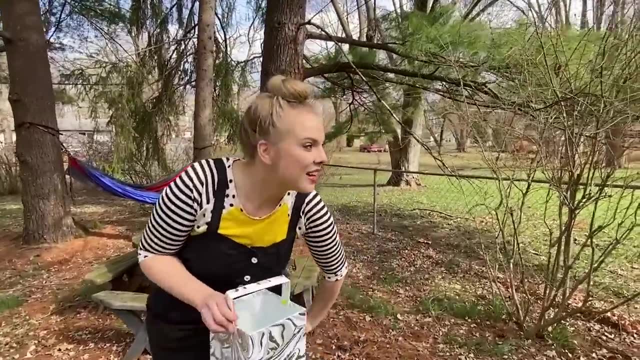 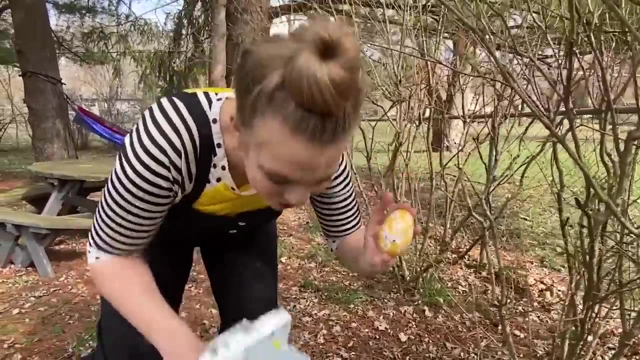 Perfect, Let's go. I'm so excited to find some eggs. Do you have your looking eyes ready? Me too. Let's do it. Oh, Oh Oh. We found our first egg. It's yellow. Should we wait or open it up now? 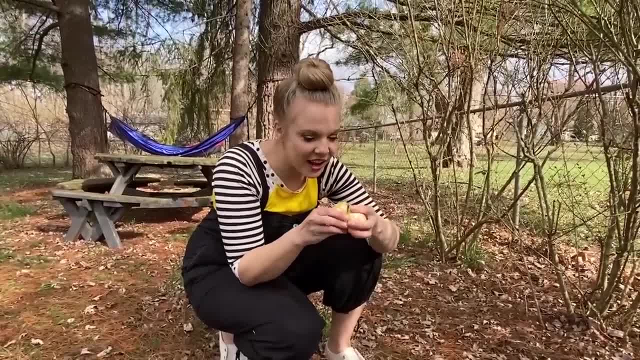 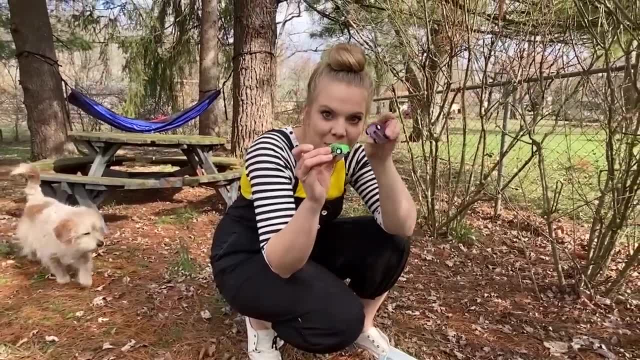 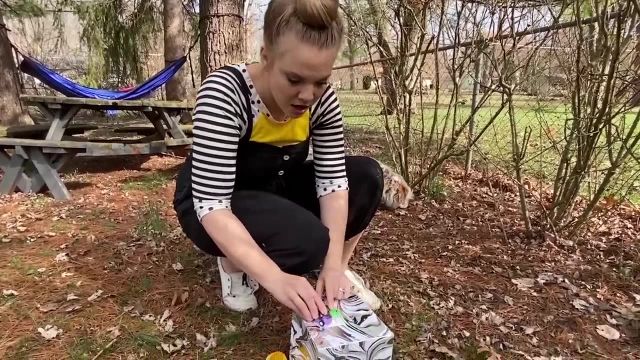 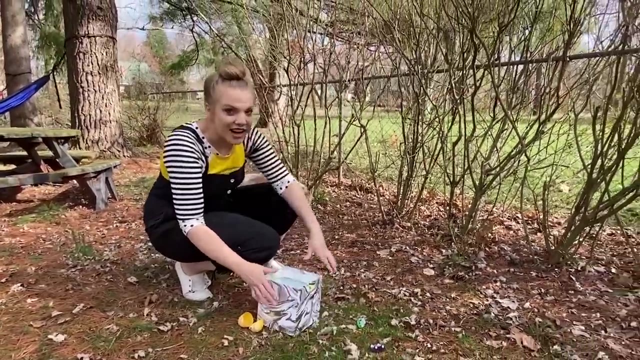 Now right, Alright, It's two cars. It's a green car And a purple car. Let's have a race. Who do you think's gonna win? I think it was green. I think it was green. We'll have to try it again in the studio. 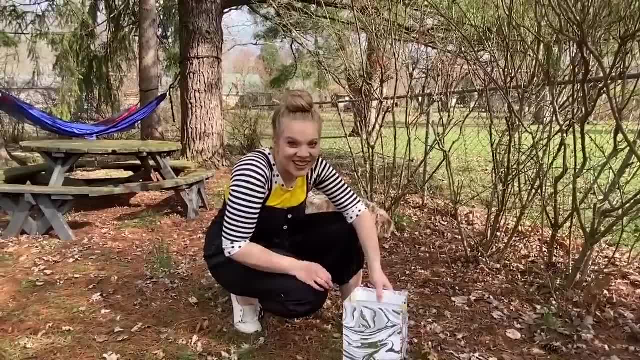 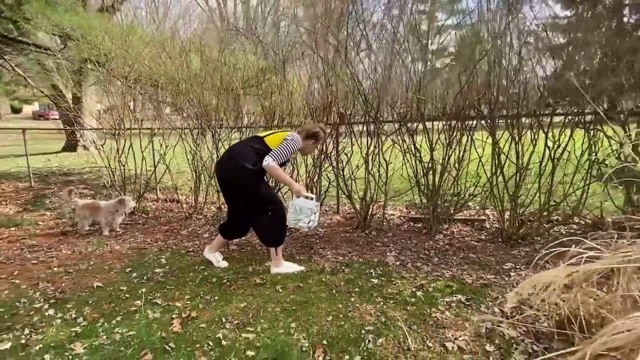 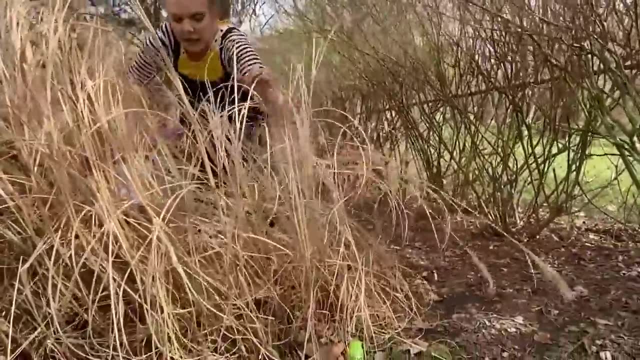 Awesome. I bet there's more. Let's keep going. Eggs, You gotta look up high and look down low. I'm so excited, I'm so excited, I'm so excited. Oh Oh, Oh, Oh, This green one. 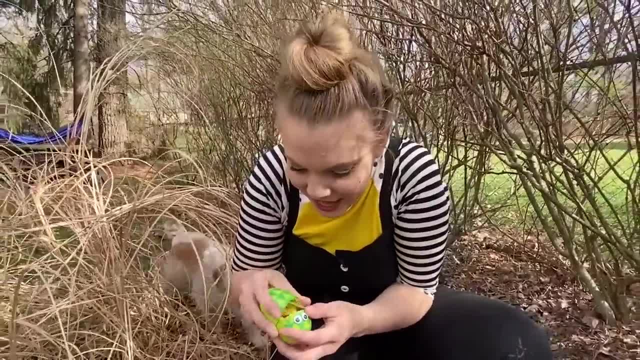 It looks like an alligator. What's inside? What? It looks like beads for a bracelet. Should we make it? There's different colors and letters. Oh, I know what this spells. I'm going to have to look at it. 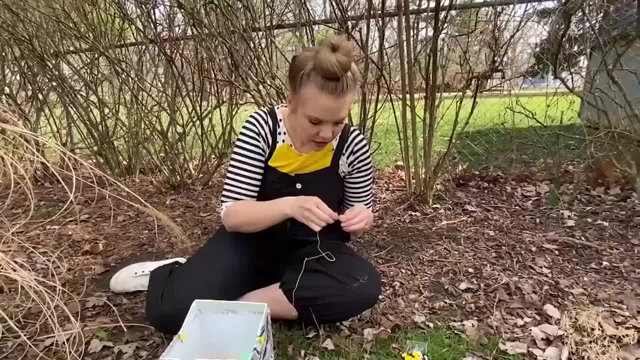 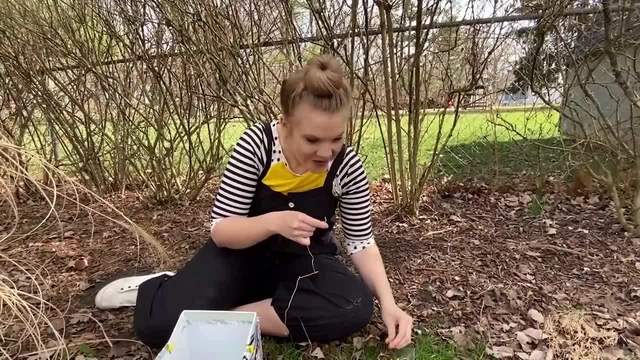 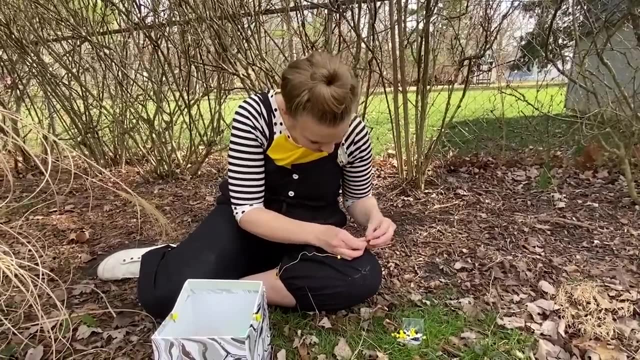 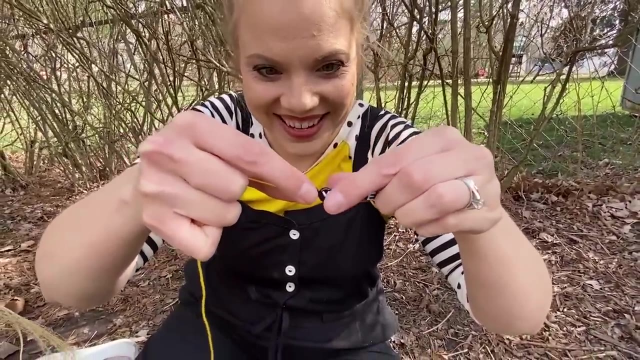 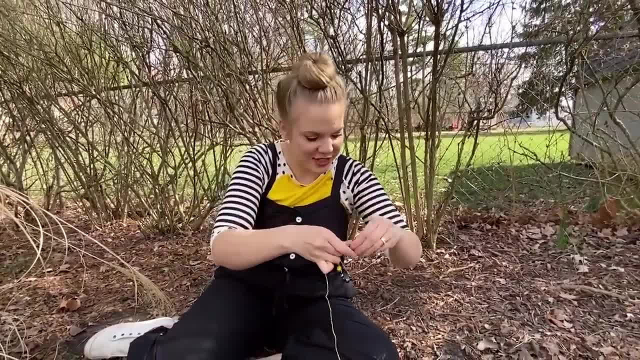 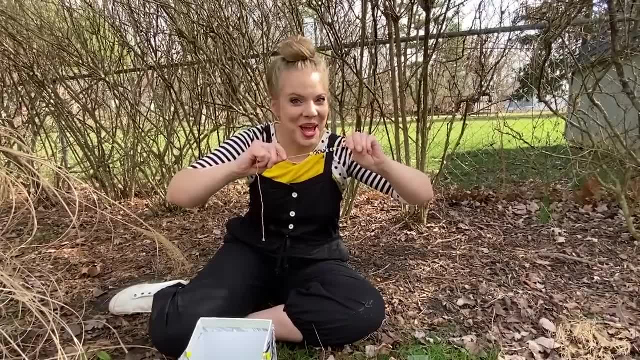 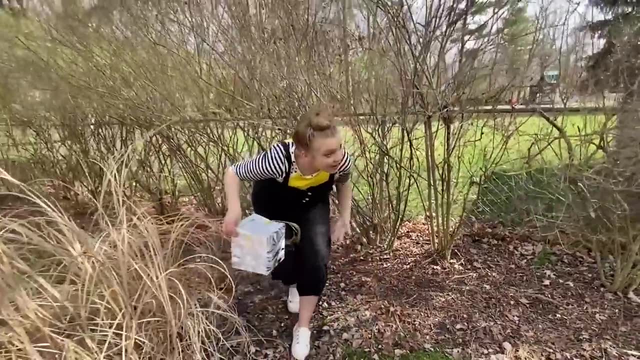 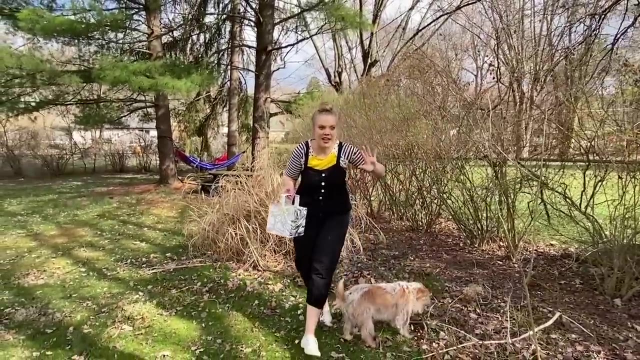 Kiley, That's me. I made a special bracelet just for me and I cannot wait to wear it. What letters do your names start with? Mine starts with K. Oh, Let's keep going. Sometimes different color eggs can blend in. 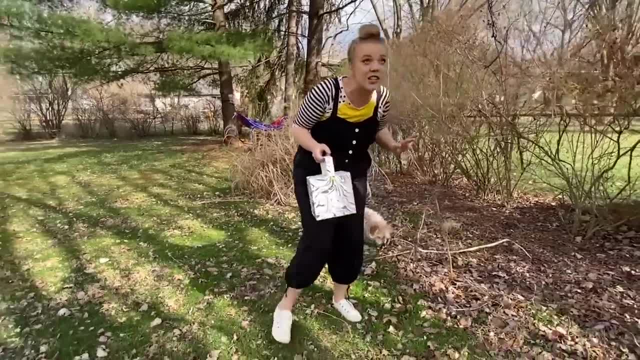 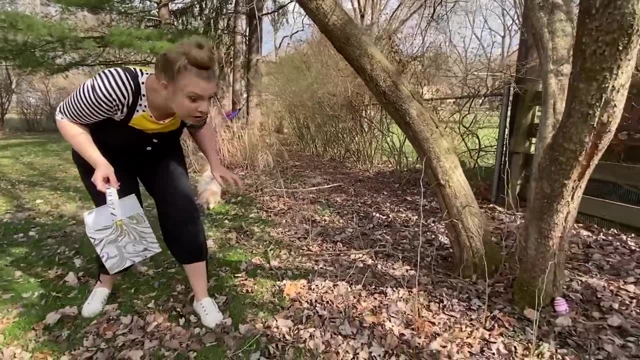 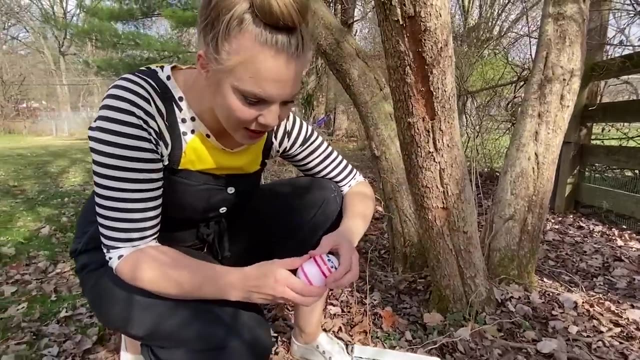 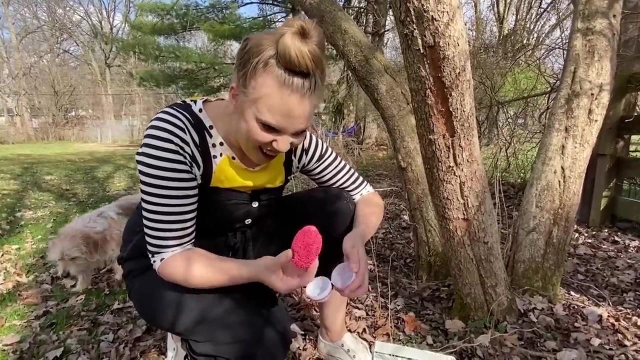 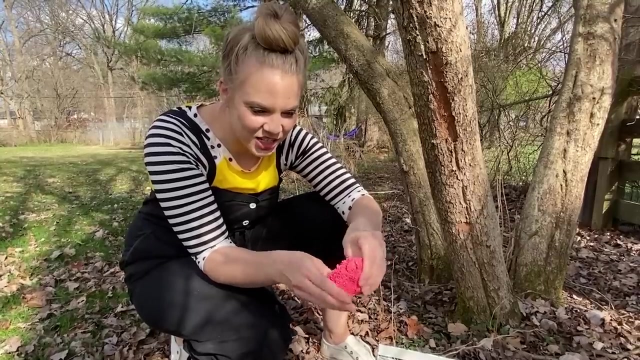 with the background. So you have to look very carefully for those camouflage eggs, What You see, one over here. Oh hi, little stripey. What's in here? What? We can mold this into whatever shape we want. Ooh, it feels good and squishy. 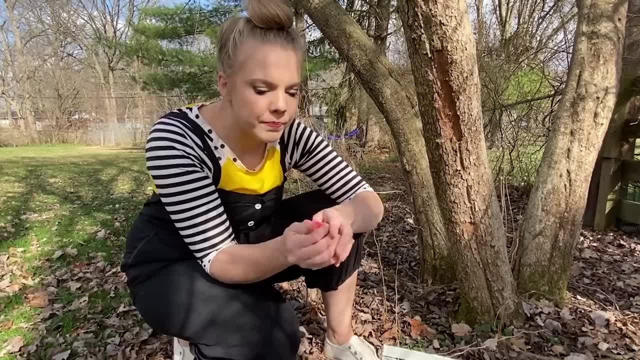 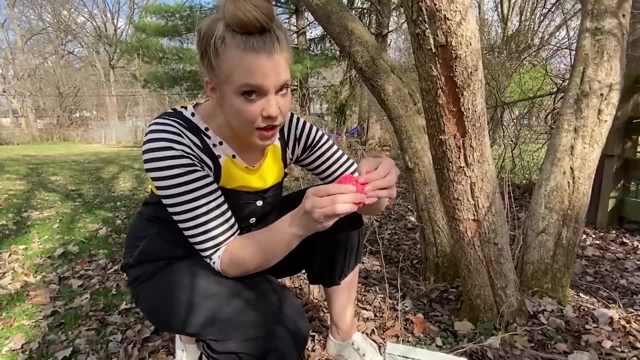 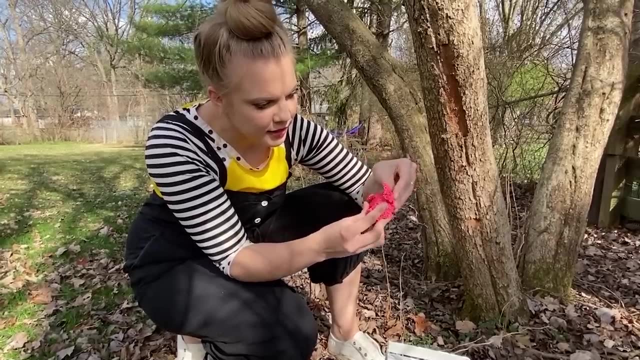 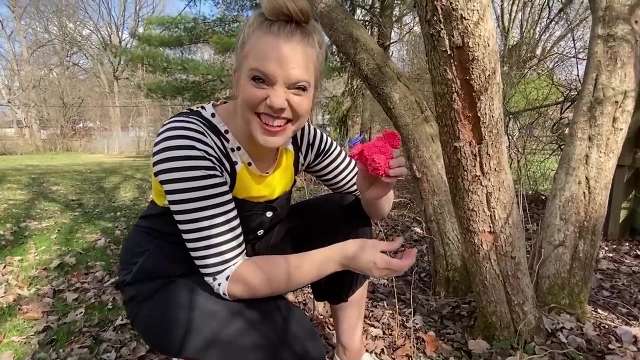 I'm going to make, hmm, maybe a dog Ball for his head. Gonna have floppy ears like Hashbrown the dog And, ooh, a cute little nose. Does it look like a dog to you? Thanks, Let's keep going. 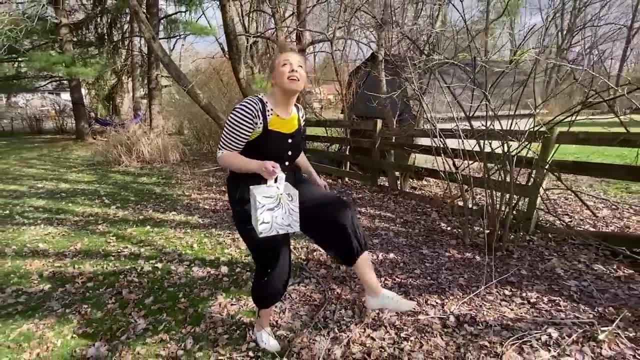 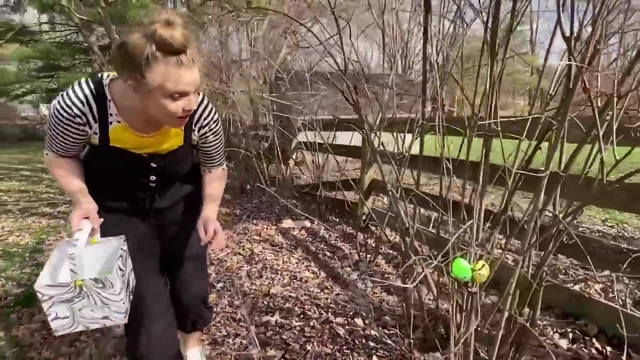 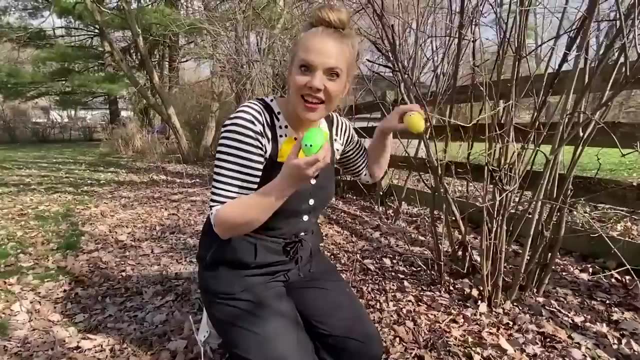 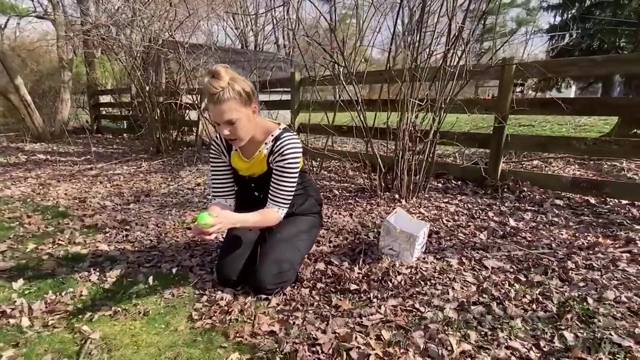 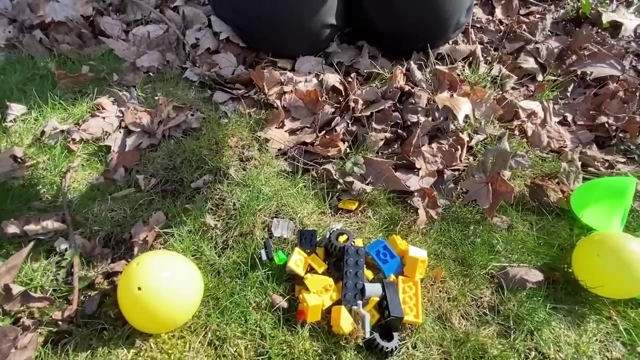 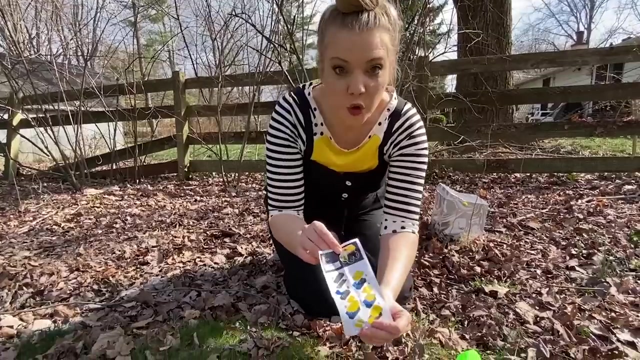 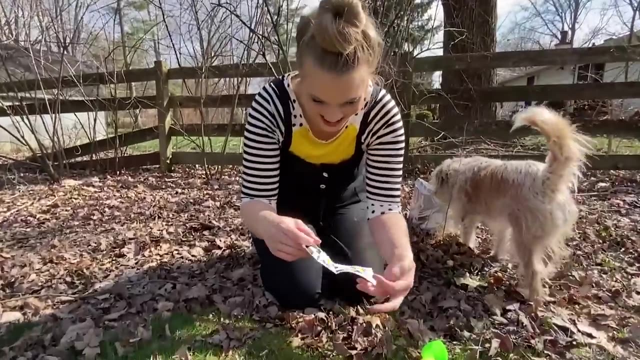 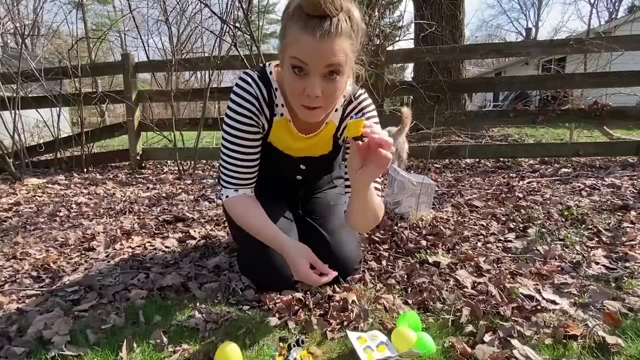 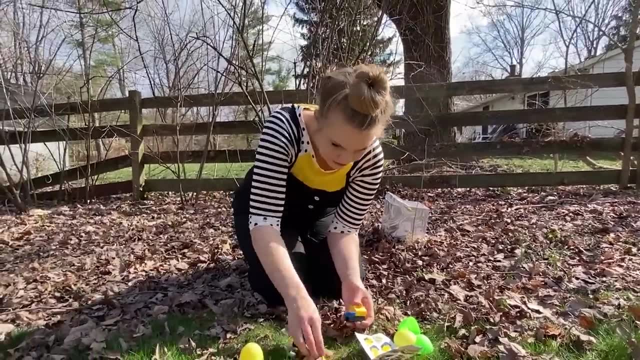 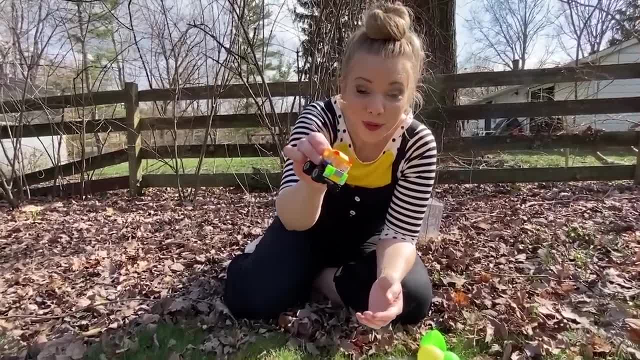 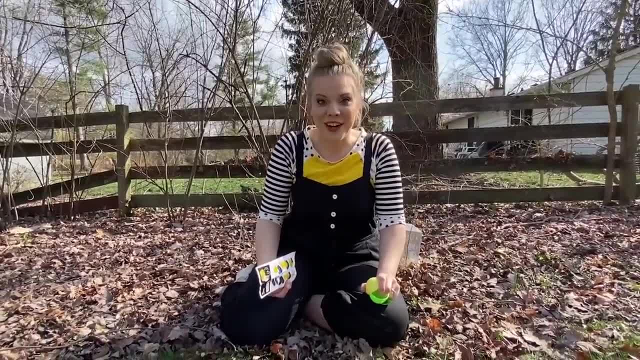 Hmm, Whoa, Two right next to each other, Green and yellow. I wonder what these have inside What. And there's instructions on how to build. Oh, This really cool truck. Should we do it? All right, amazing, that was fun. do you think there's more out here? 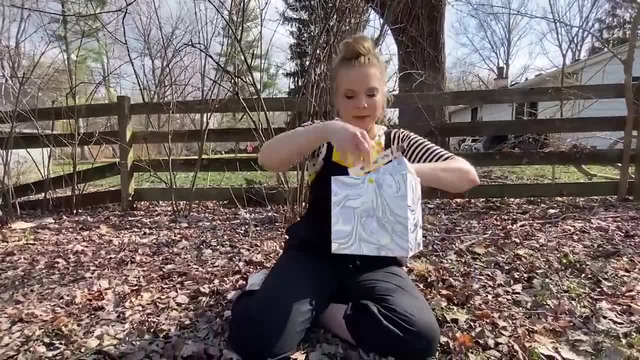 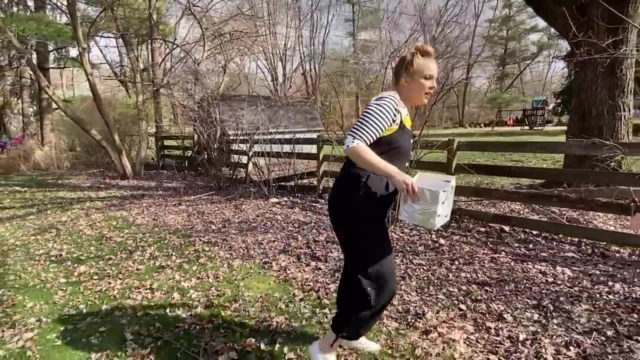 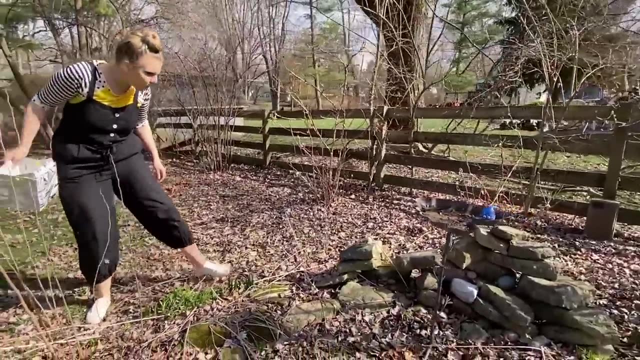 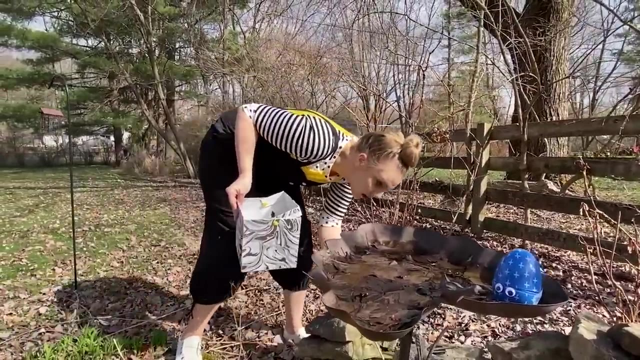 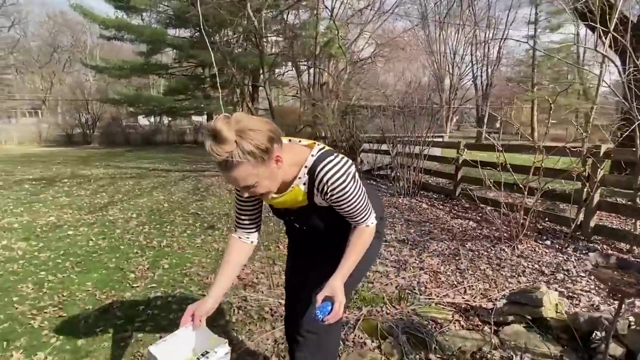 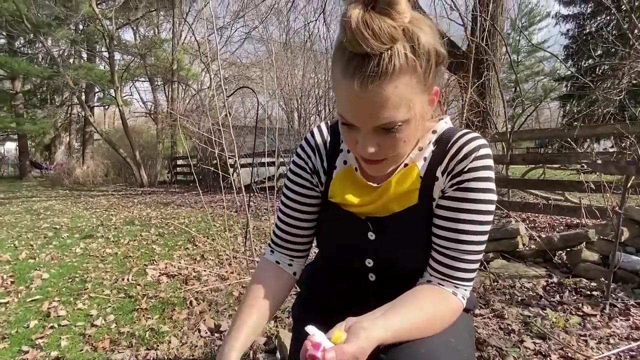 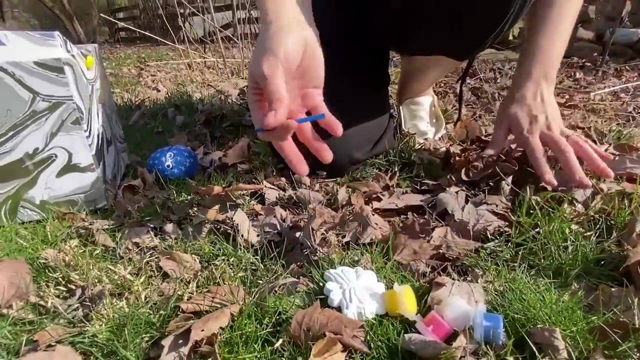 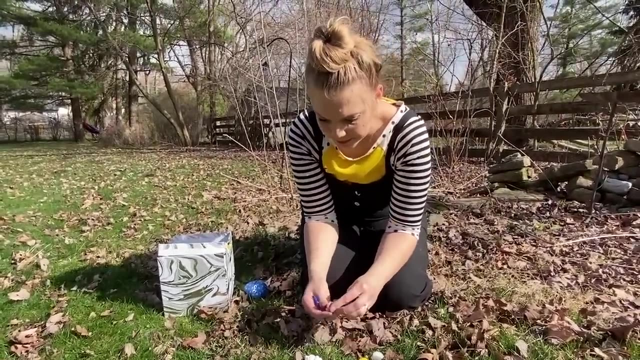 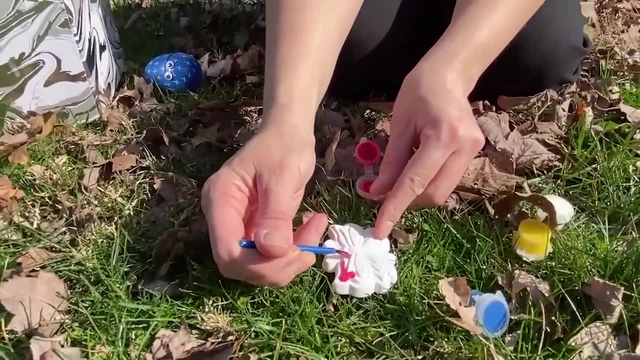 this is awesome. come on, this would be a good place to hide an egg. I see you, this is an amazing surprise egg. it's a little butterfly and a tiny, tiny paintbrush and paints to paint it with. let's do it. this is an amazing surprise egg. it's a little butterfly and a tiny, tiny paintbrush and paints. 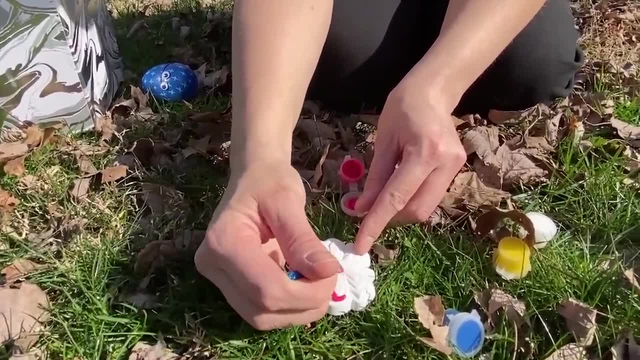 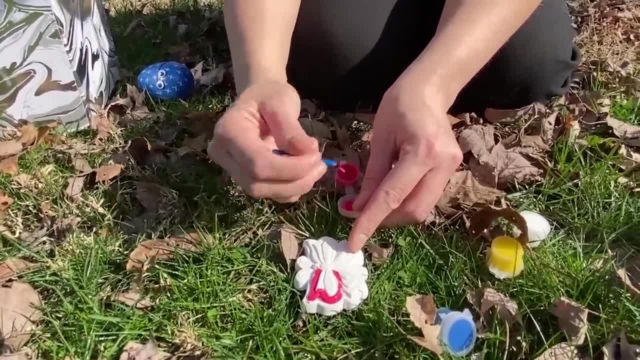 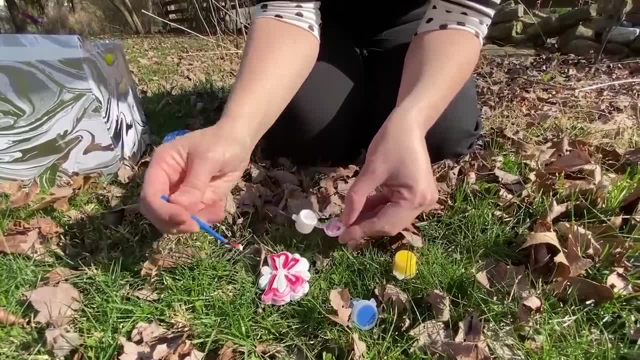 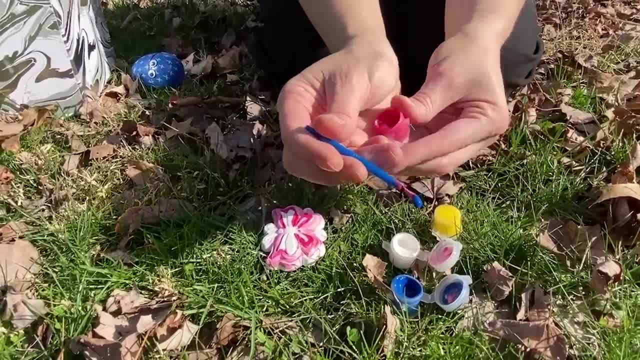 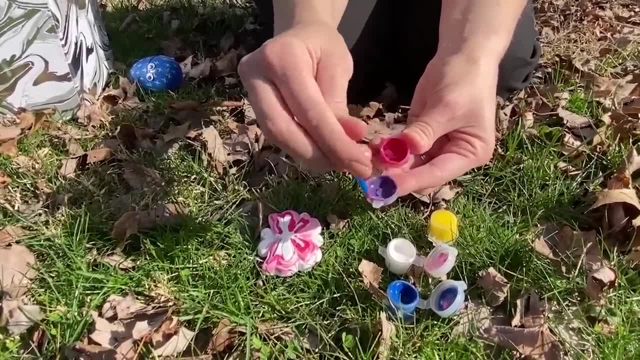 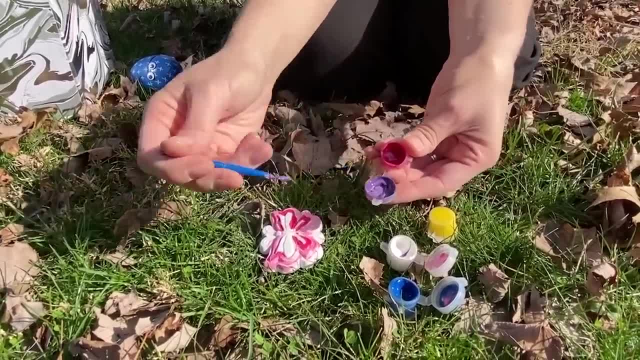 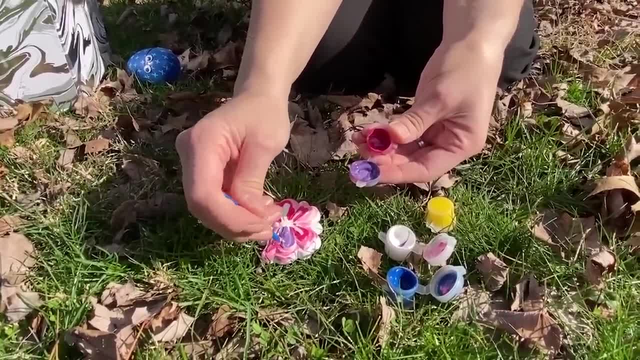 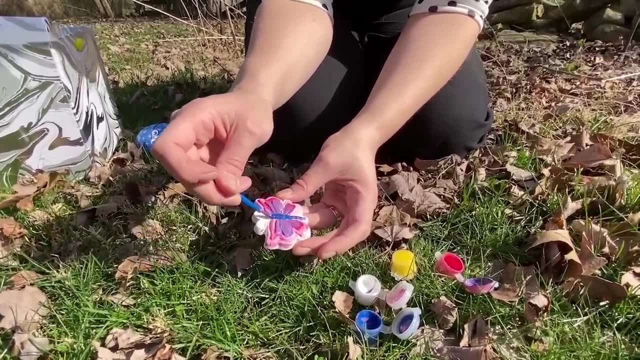 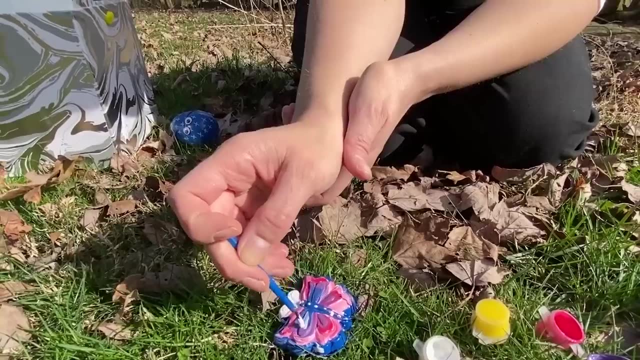 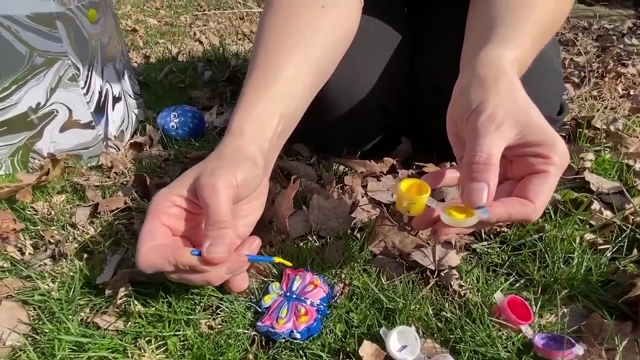 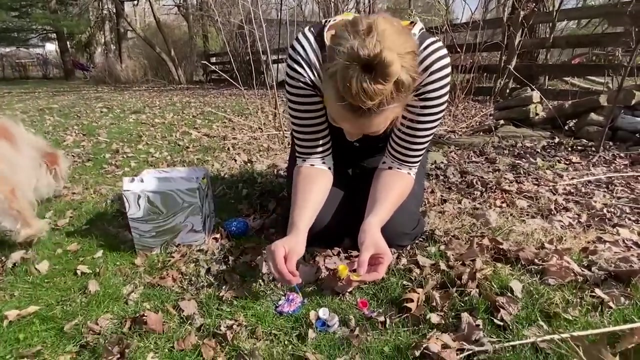 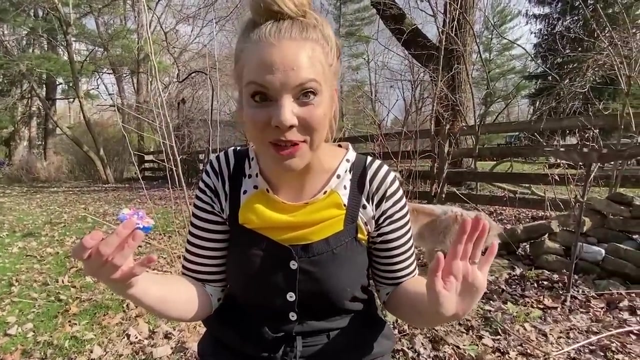 to paint it with. let's do it. this is an amazing surprise egg. it's a little butterfly and a tiny, tiny paintbrush and paints to paint it with. let's do it. Excuse you, I think this is the happiest little butterfly. I can't wait for it to dry so that I can display my piece of art in my house. 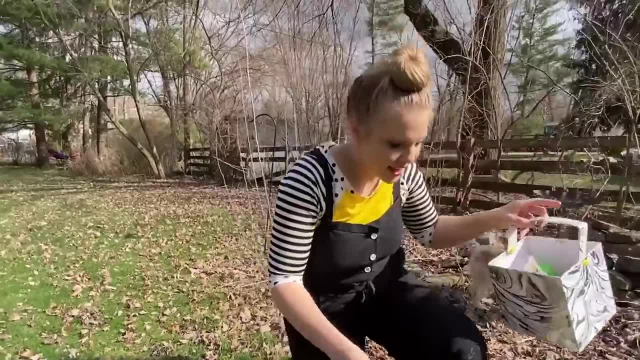 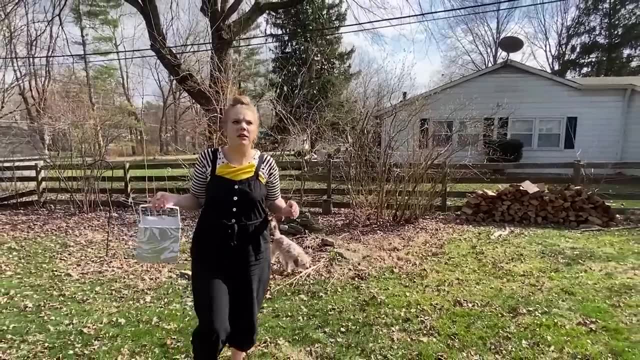 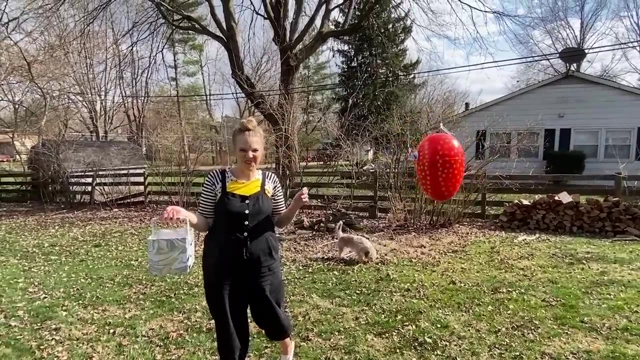 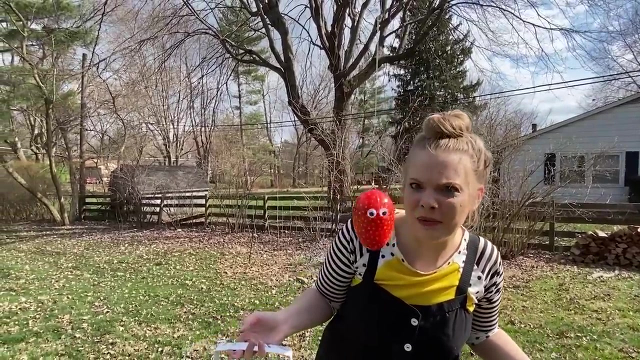 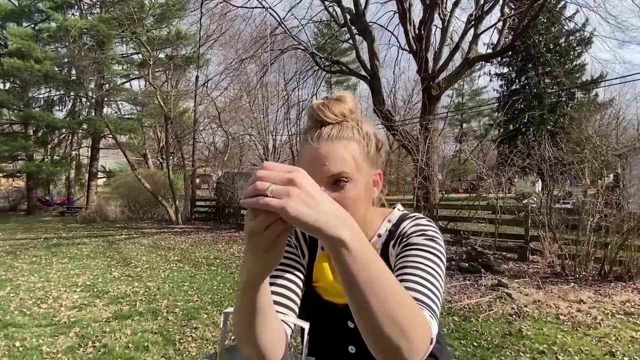 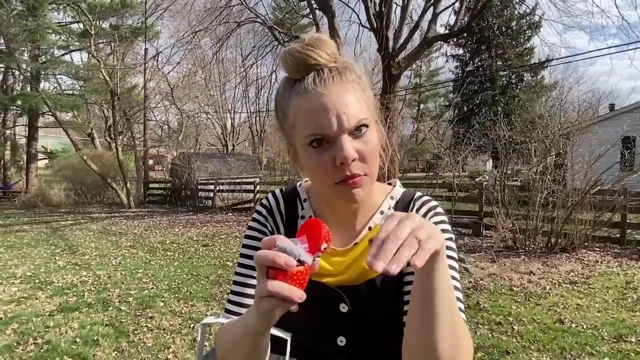 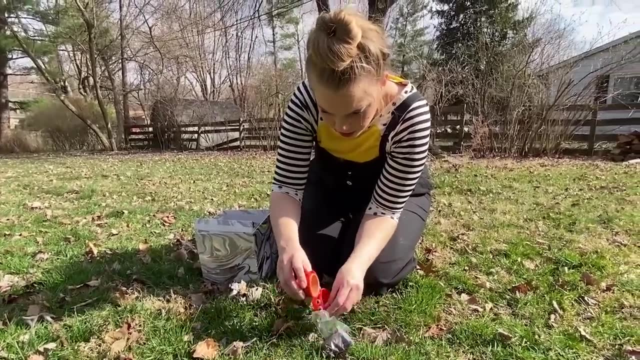 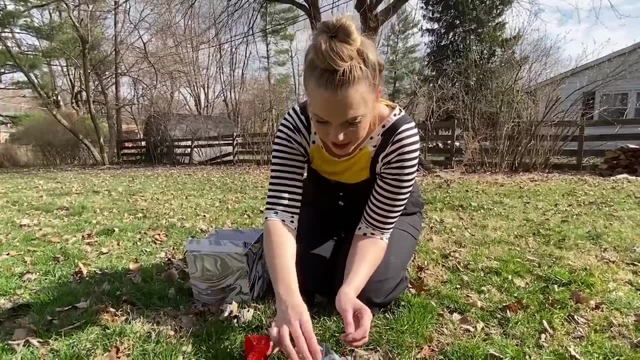 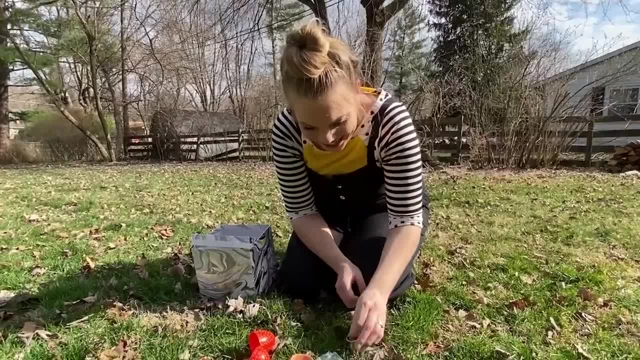 Let's keep going. What? How did this get here? And what is inside? Only one way to find out What? Come on down here. What I know what this is? It's a little flower pot soil, a tiny seed and a little bucket and a little trowel to plant it with. 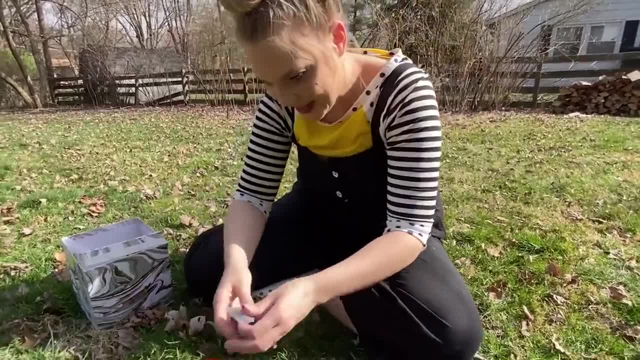 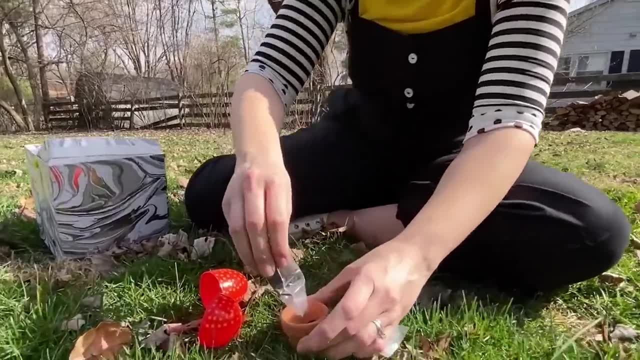 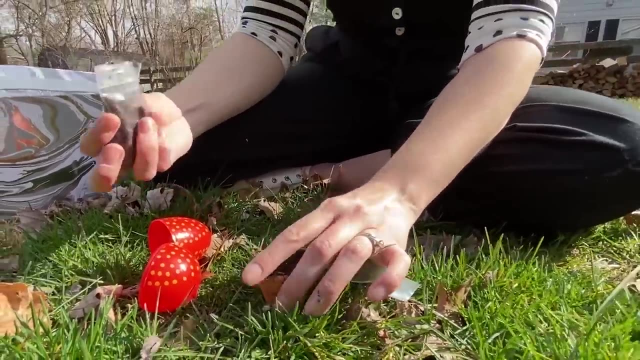 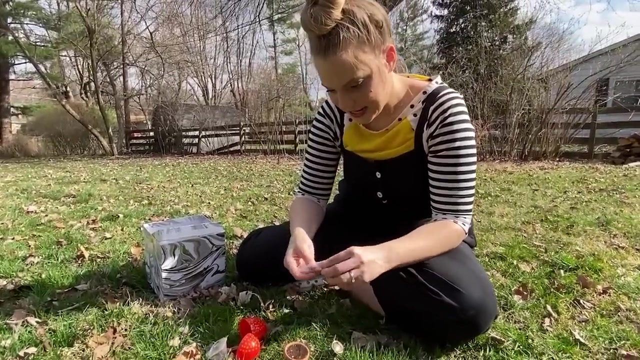 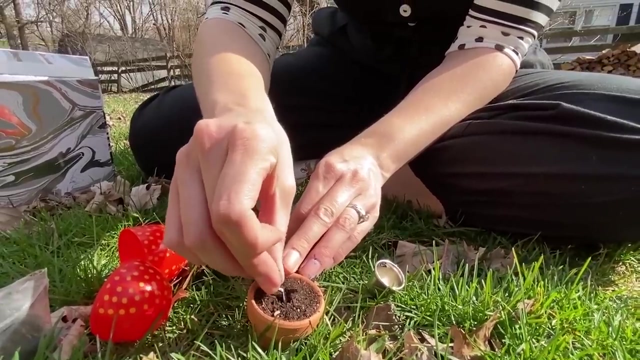 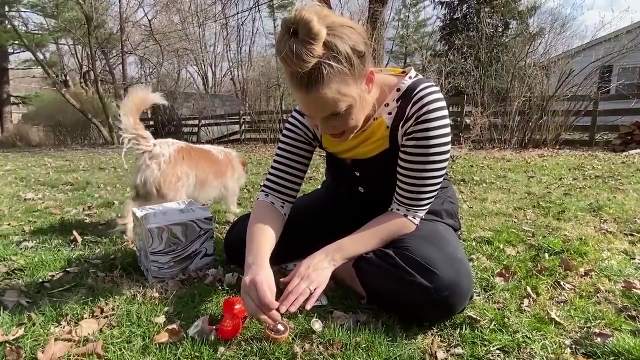 That is so fun. Let's do it. First the soil: Fill up our pot. That looks like enough. Now let's get out our seed. We'll dig a little hole And plant it, Cover it up, Press it down a little bit. 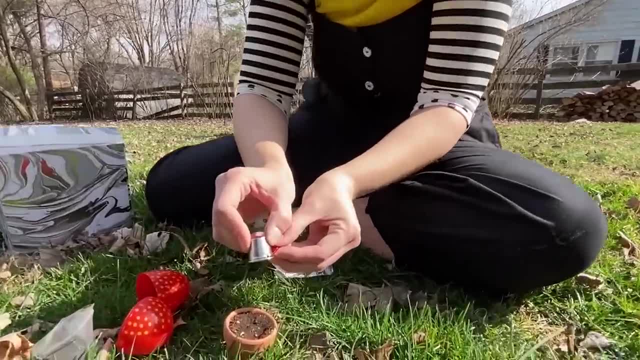 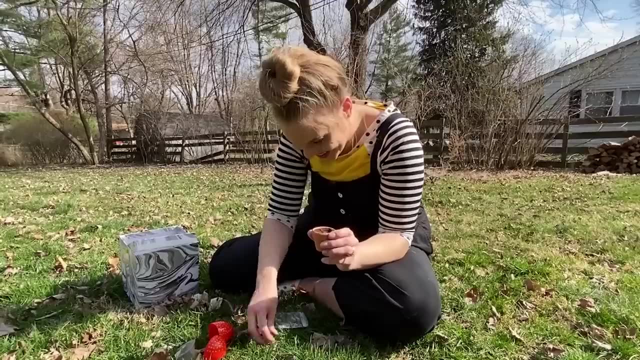 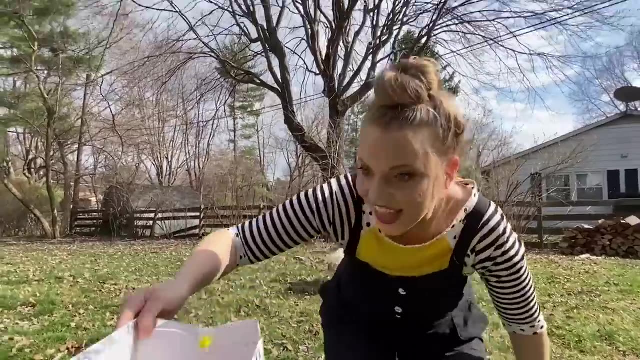 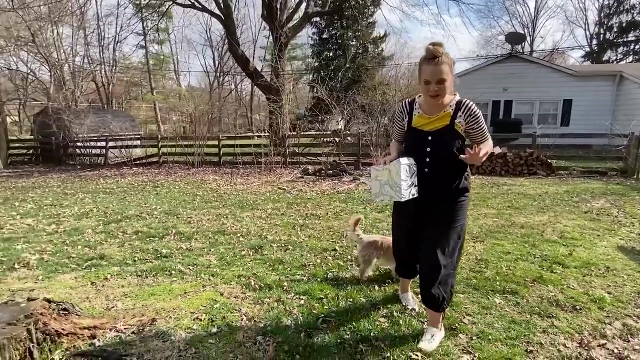 And then water it. I'll have to put real water on it later. I can't wait to see what this grows into. Cool, Wow, I have a feeling that there's one more. The stump is always a good place to look for things. 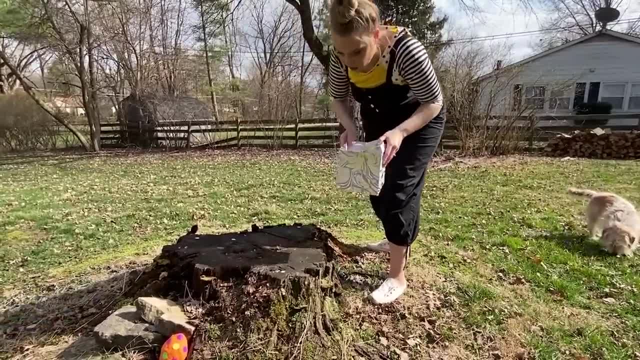 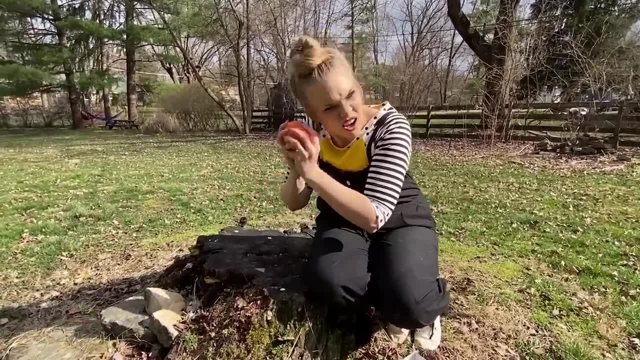 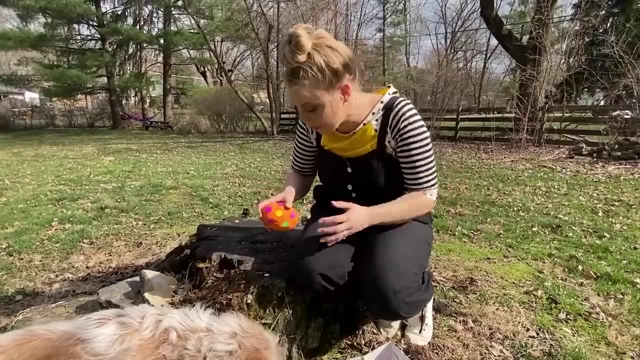 Let's check it out. Whoa, What Do you hear? that There's something inside. This is a surprise egg with a toy inside, just like the other ones that we just found. How do we get it out? Have you ever broken open a real egg? 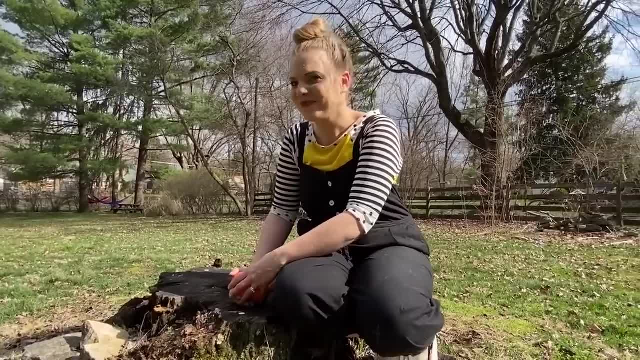 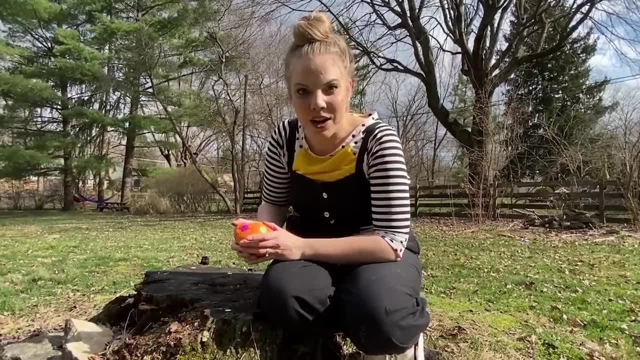 Like when you're helping bake a cake or cook. You have to crack the shell, don't you? I wonder if, to get the surprise out of this surprise egg, we have to crack the clay open. Should we try it Okay? 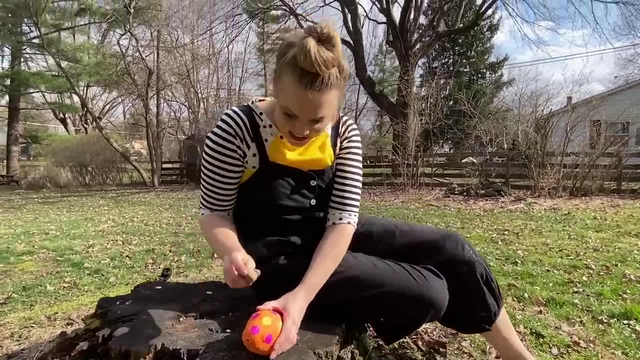 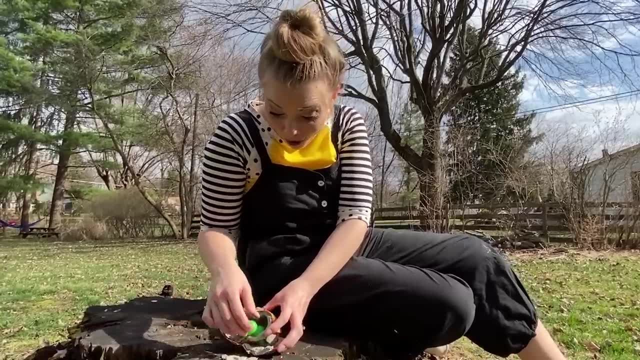 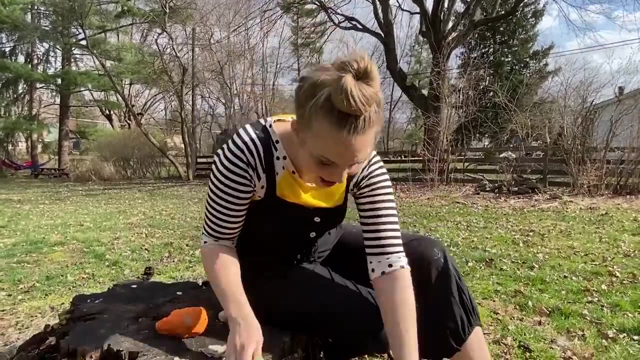 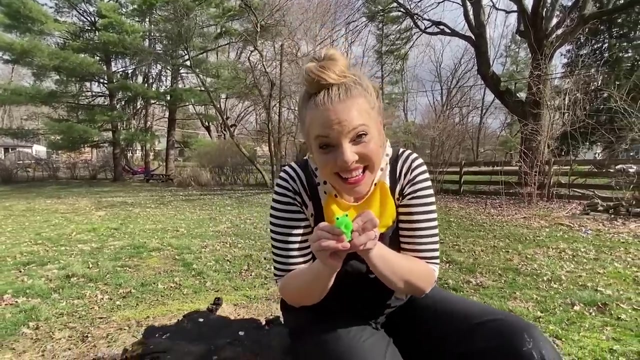 Ready? Alright? One, Two, Three, What is? I know what this is. This is watch. Put the little ball in his mouth and, Sorry, I shot you with a ball. That is so fun. Throw it back. 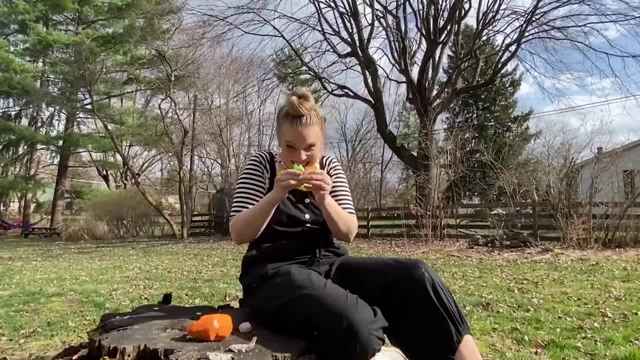 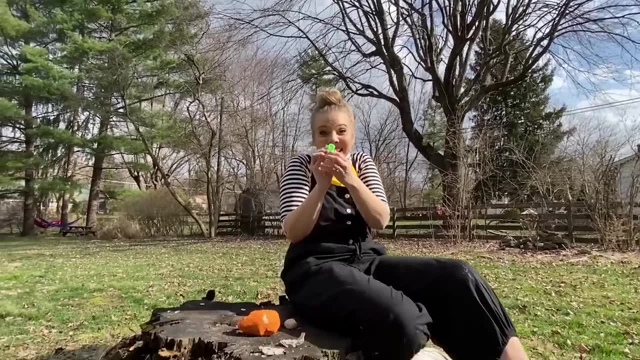 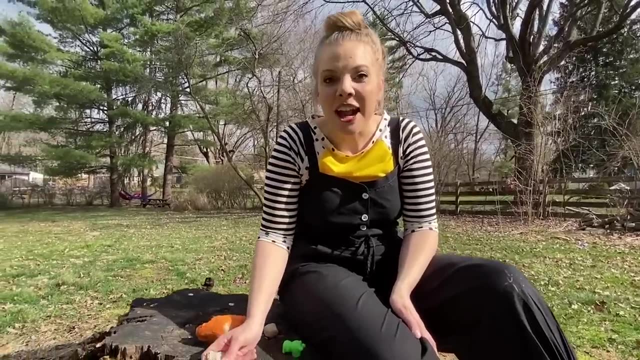 Nice, Alright, catch You ready. Okay, Oh, Oh. This is so fun, And this has given me a great idea On how to use the supplies that we found in the MakerBox earlier. You want to go do it now. 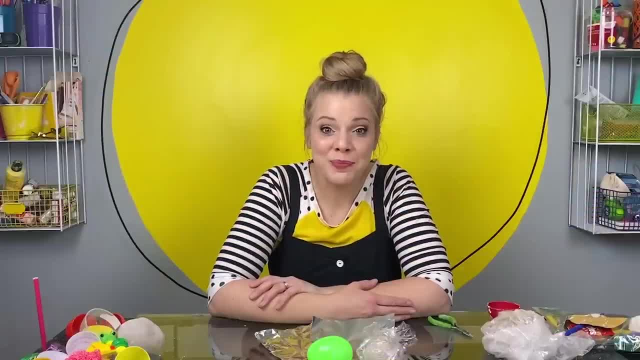 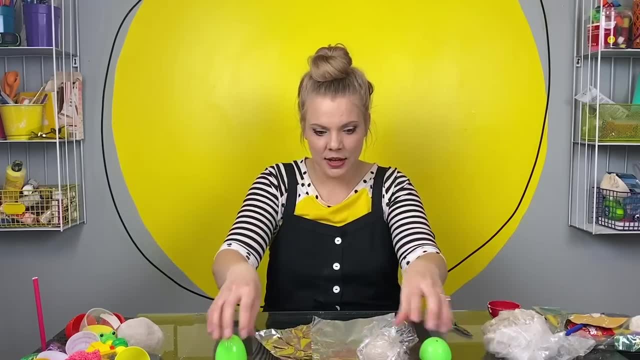 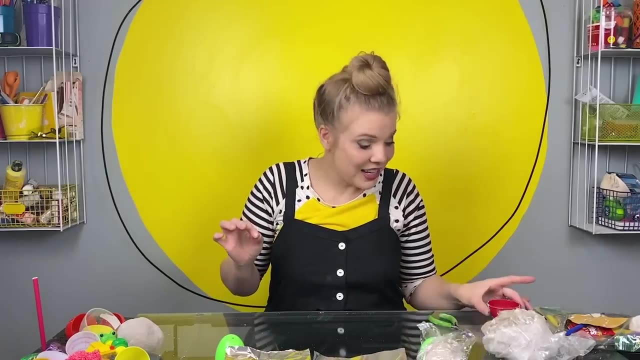 To the studio To make your very own surprise clay egg. here's the things that you're gonna need: A plastic egg that comes apart in two pieces, Some air-dried clay, Two small pieces of tin foil, A little cup of water. 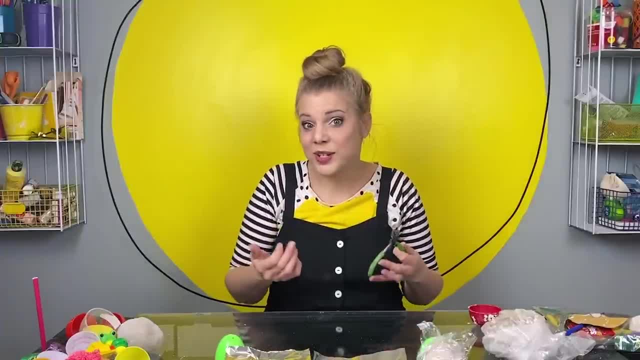 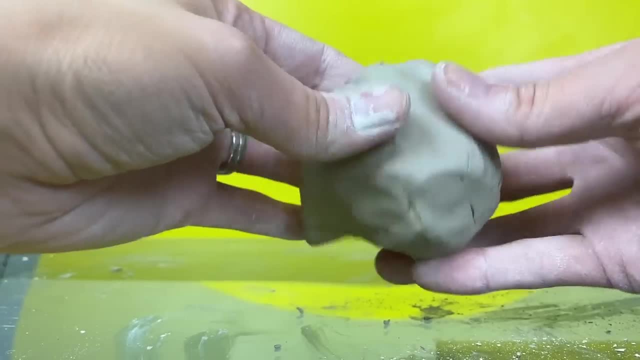 The first thing you're gonna do is cover the two halves of your eggs in tin foil. The first thing you're gonna do is cover the two halves of your eggs in tin foil. side of the egg. If you want to make it a little bit smoother, you can dip your finger or your. 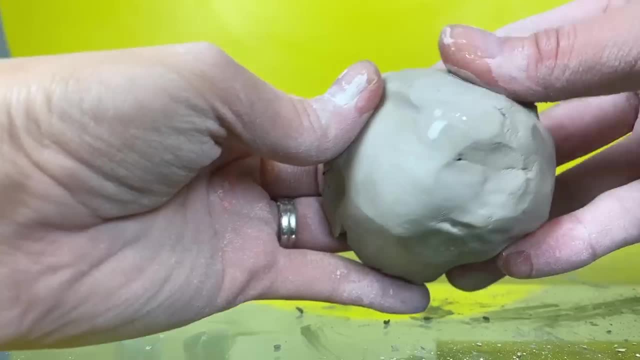 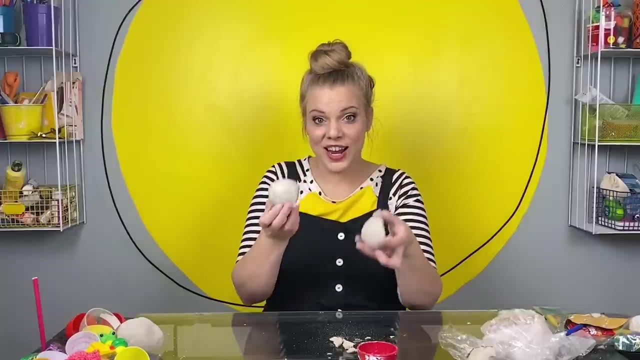 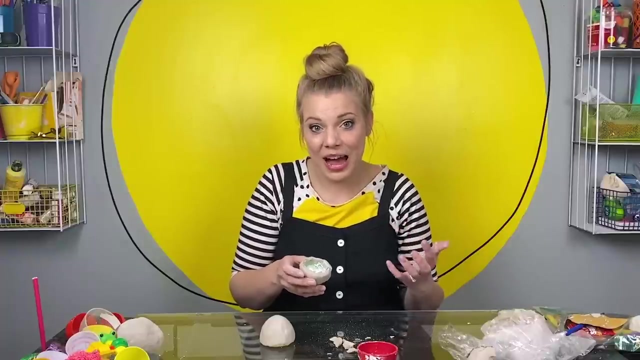 thumb in some water and smooth out any fingerprints or cracks or lines that you have. Repeat that with the other side. Both of the halves of our eggs are covered now, So the next thing we need to do is to get the plastic egg out. How we're going to get the plastic egg out so that the clay can dry without? 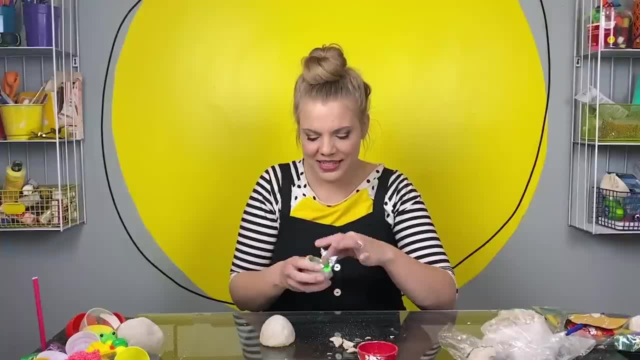 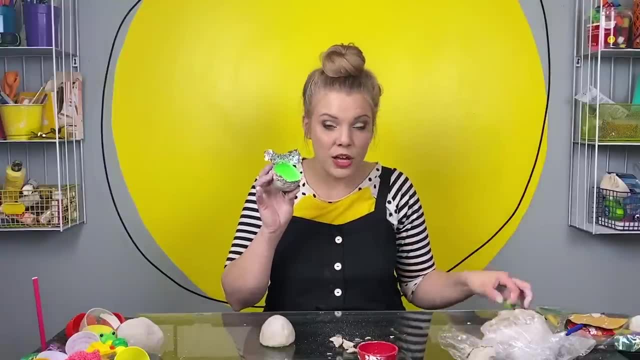 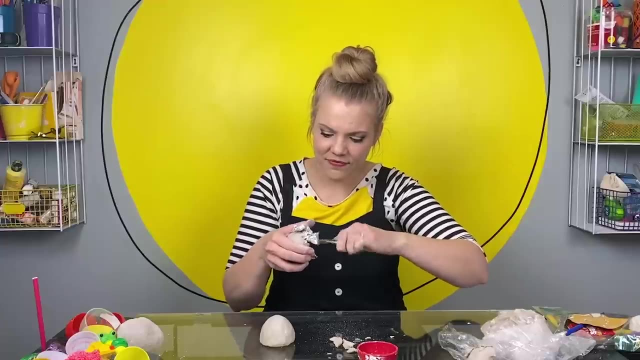 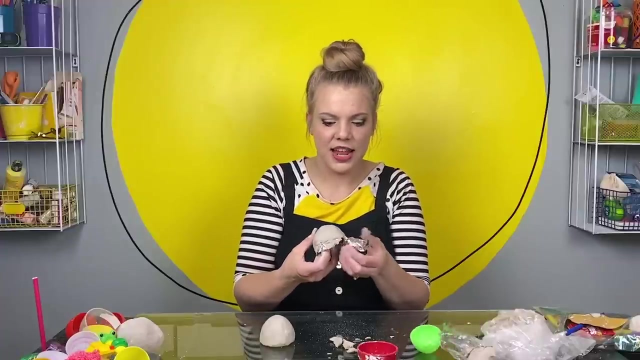 it in there is to start peeling back our tinfoil from inside the egg. Once you've peeled the tinfoil back, you can use your fingers or a pliers or tweezers to grab onto the edge of the plastic egg and just pull it right out Like that. This leaves an egg-shaped clay ball that's hollow inside. 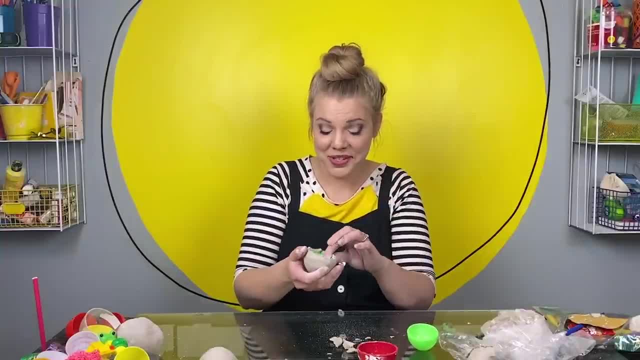 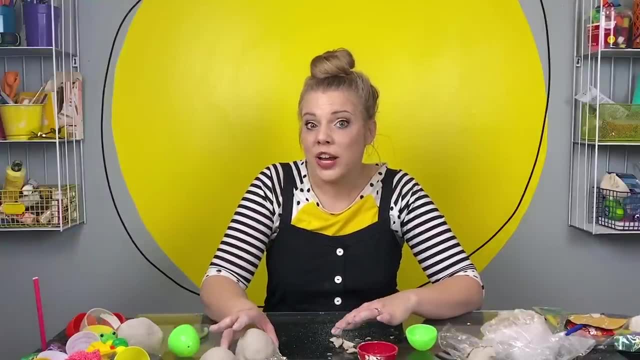 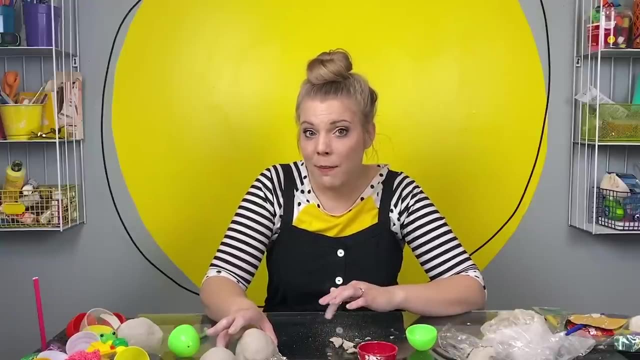 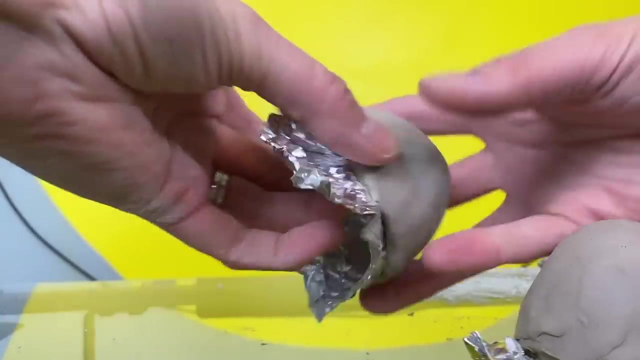 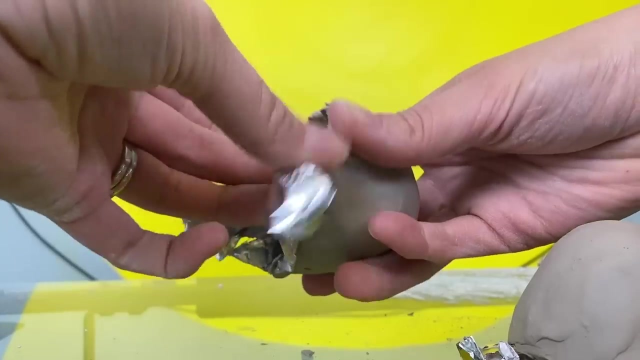 with the tinfoil still in. Do that for both sides. Now we want to let these dry for a little bit with the tinfoil still inside. You want to make sure that they don't air dry all the way until we're done with the next part. You want the clay to be a little bit moist for this part but still be able to hold its shape when you take the tinfoil out of the inside. I'm going to start peeling away the tinfoil on the inside. If these are dry enough, that'll come right out. It's going to be a little bit more. 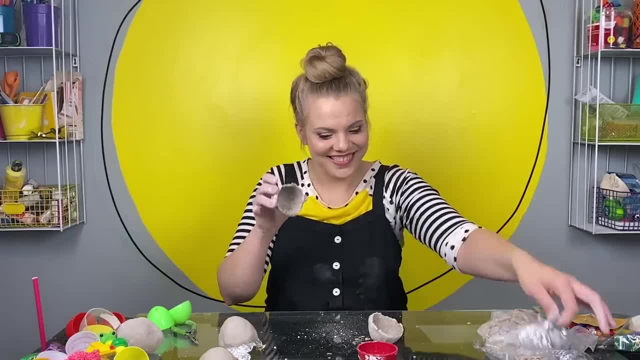 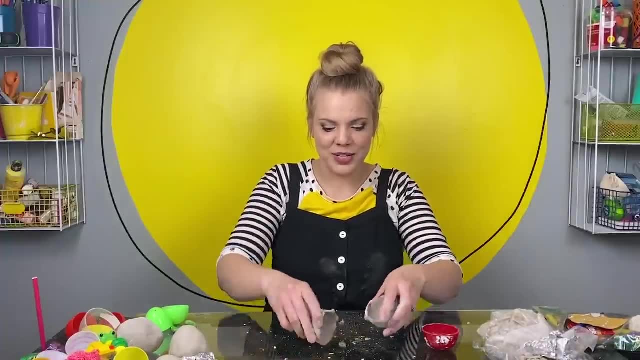 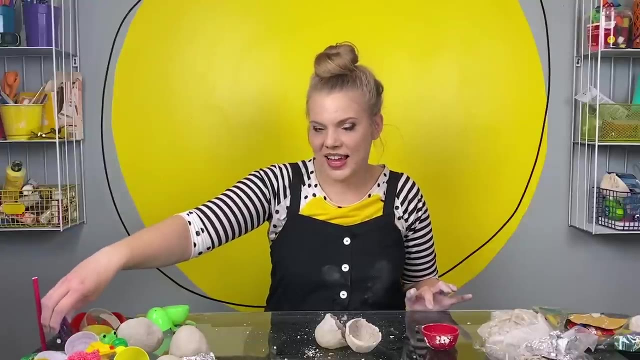 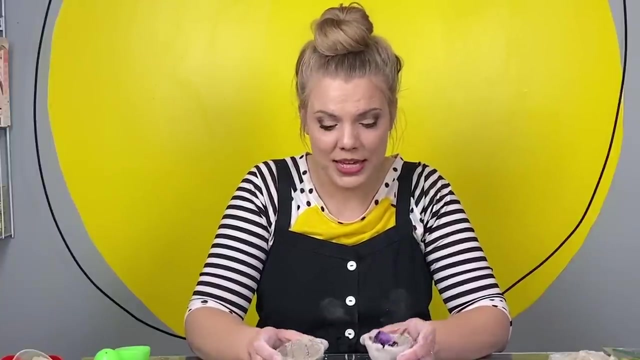 wrinkly on the inside, but that's okay. Next comes the super fun part. We get to decide what surprise we're going to put into our surprise egg. I think I'm going to put a car into this one. Now it's time to seal it up so that it's all one piece. The reason that we still want this to be a little bit wet when we do this is so that the new 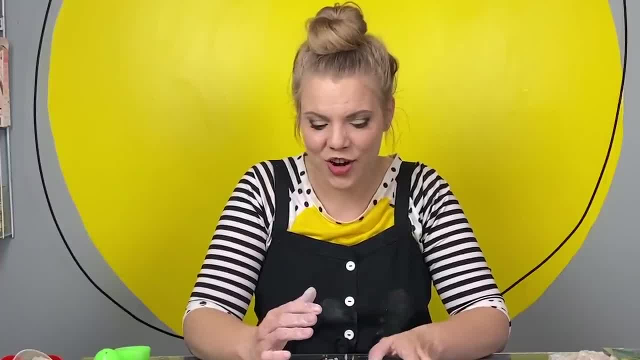 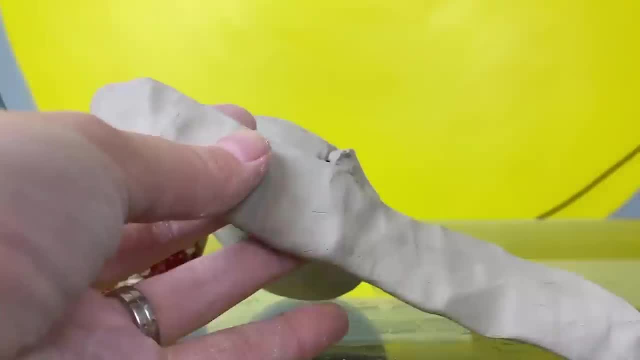 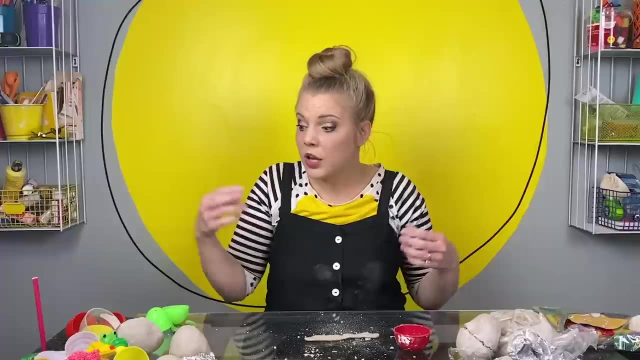 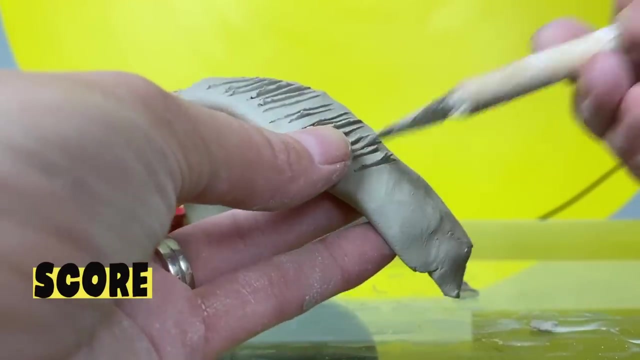 clay sticks to this clay and doesn't crack away from it when it starts to dry. I'm going to roll this piece of clay into a coil and kind of flatten it out a little bit like this. Once I've done that, I'm going to use a clay tool. If you don't have one, you could use a toothpick or a knife or a pencil, And I'm going to score the clay, which is what's going to help it grab on and stick together. Scoring the clay just means I'm going to draw a bunch of lines in it like this Kind of like scratching. 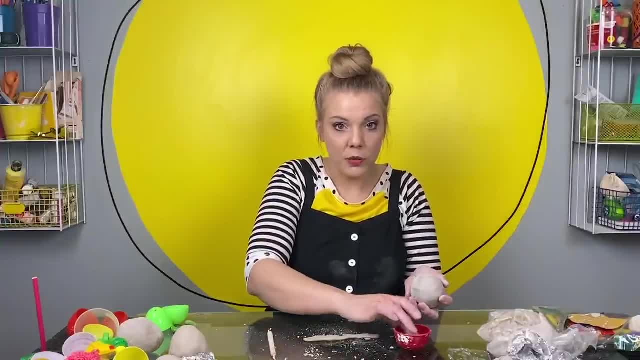 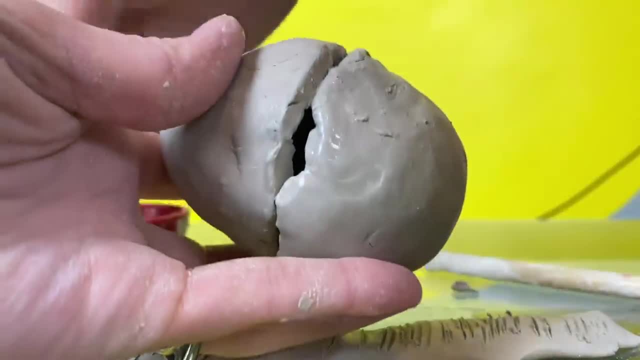 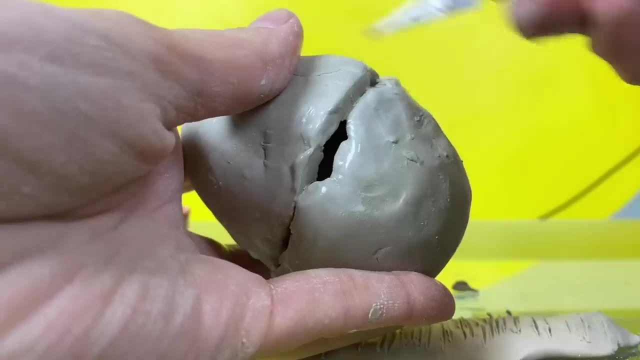 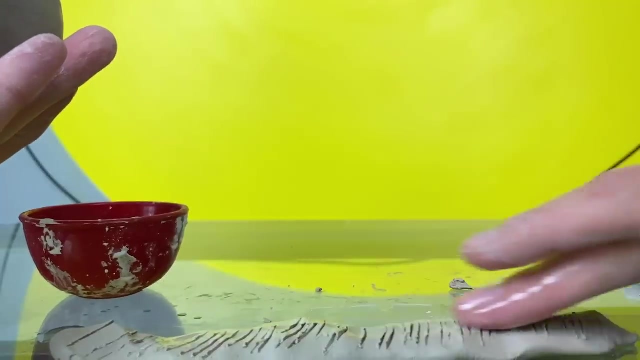 Great, Now I'm going to go all the way around the seam of my egg and just get this clay wet again, Just like that. Now I'm going to score the outside of this egg all around the seam, Scratch it up. Now I'm just going to put a little bit of water around everywhere I scored- even on my new clay, and lay it over. 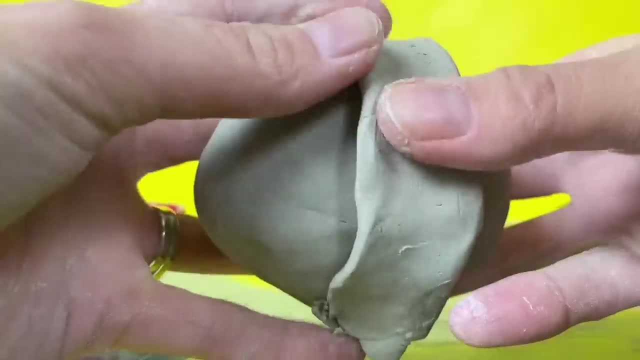 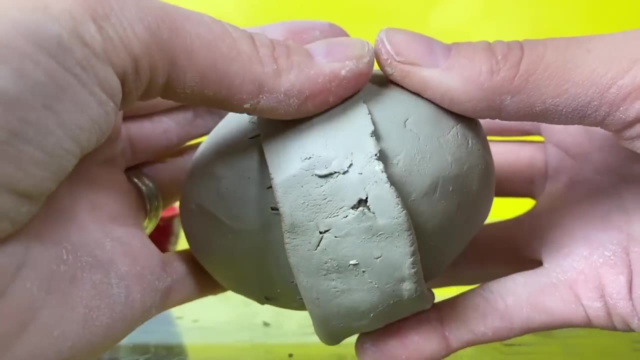 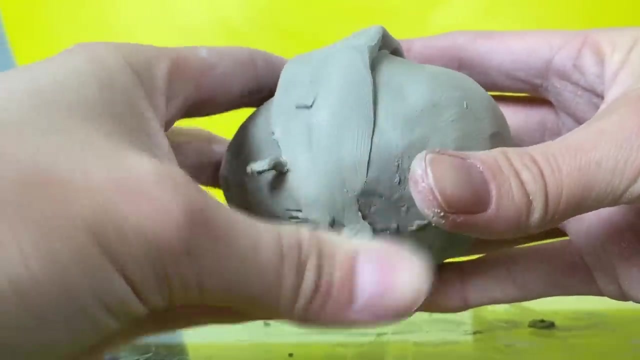 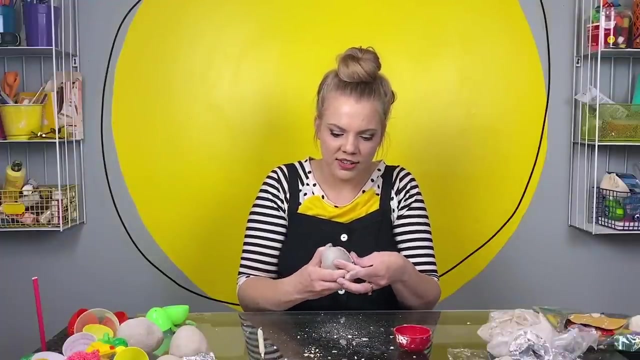 the middle. I'm then going to use water and my fingers to just smush it and blend it in. We're never going to push too hard because, remember, this clay is still wet so it still will squish a little bit. So just gently and carefully go along connecting your coil and smoothing it into the egg. 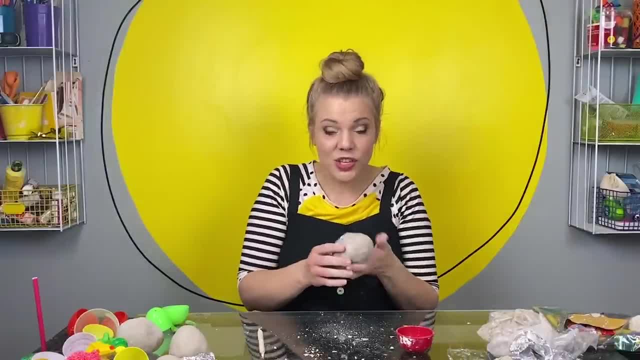 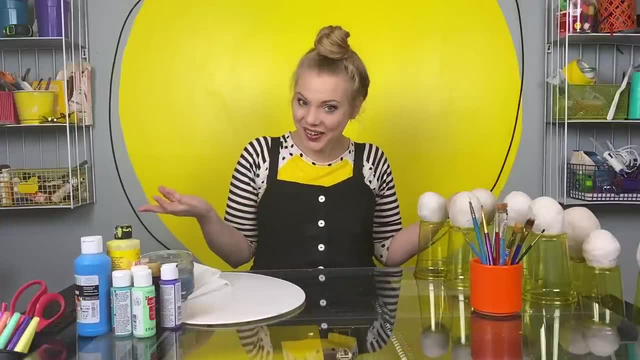 Now the two pieces. It just became one piece. Let this dry overnight, and then the next day you can paint your eggs. The eggs are all dry, which means it's time to decorate them. There's lots of ways to pick the colors that you're going to use. 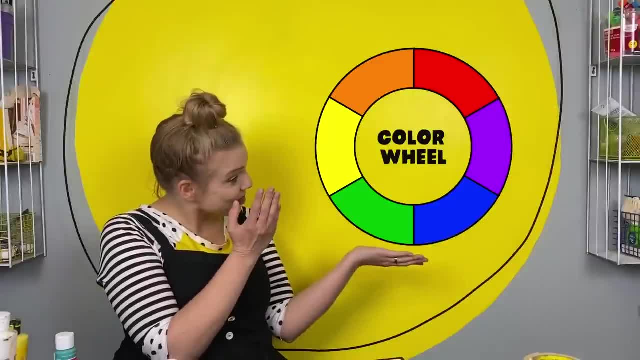 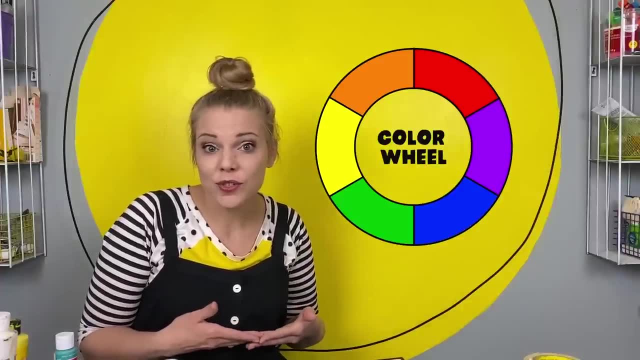 One of the ways that we understand color is by using the color wheel. The color wheel helps us understand the relationship between colors and helps us pick what kind of colors we're going to use. Today I'm going to use complementary colors because when complimentary colors are, 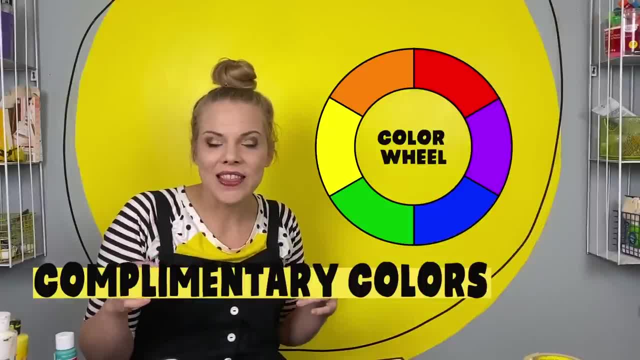 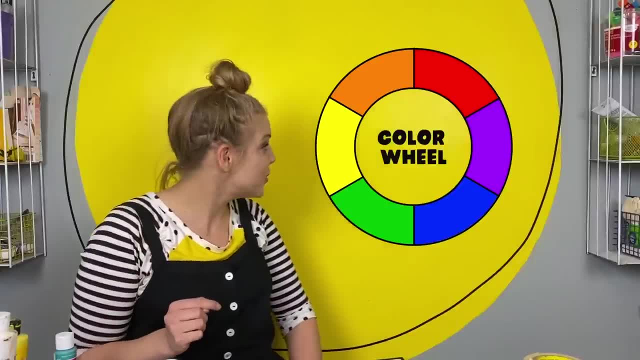 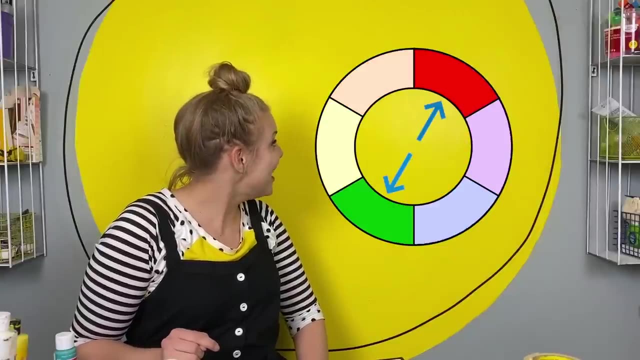 next to each other. they give a lot of energy to whatever you're painting and they make the colors really pop. Complementary colors are colors that are opposite from each other on the color wheel. So we have purple and yellow, orange and blue and red and green. Those are the complementary colors and that's what I'm. 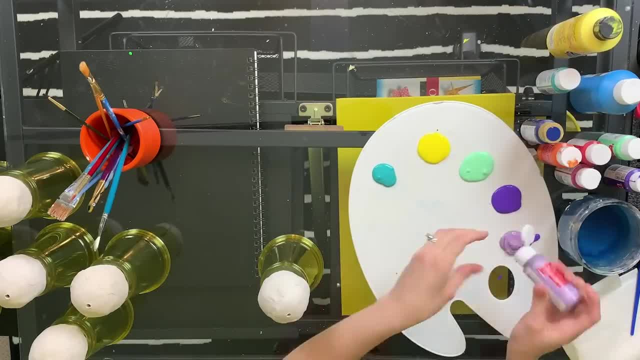 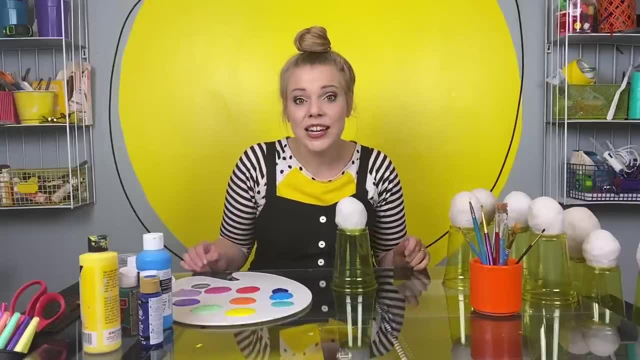 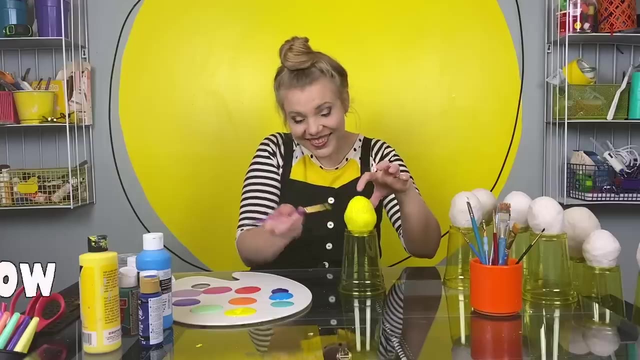 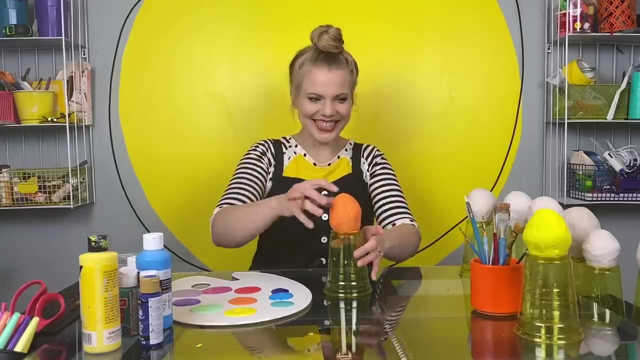 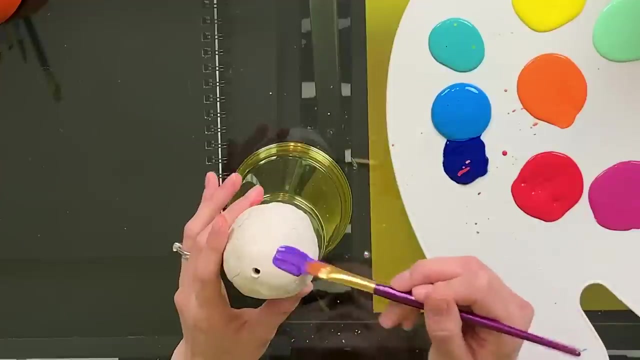 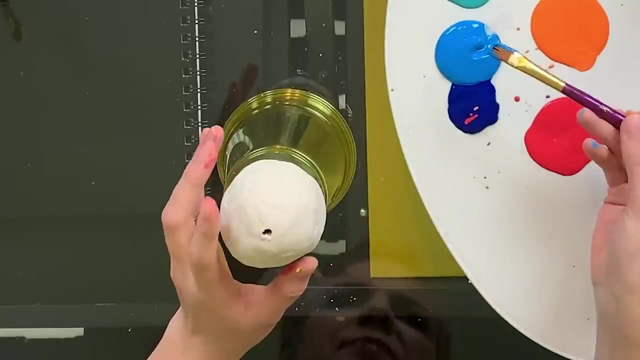 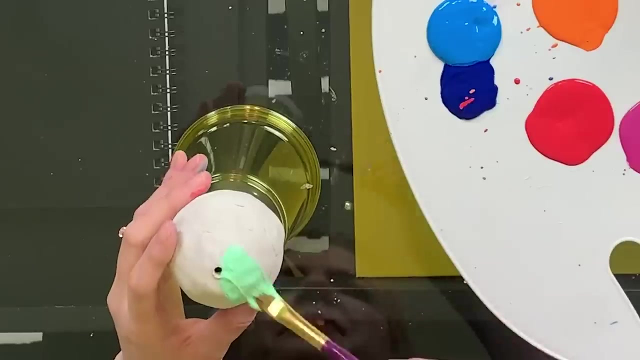 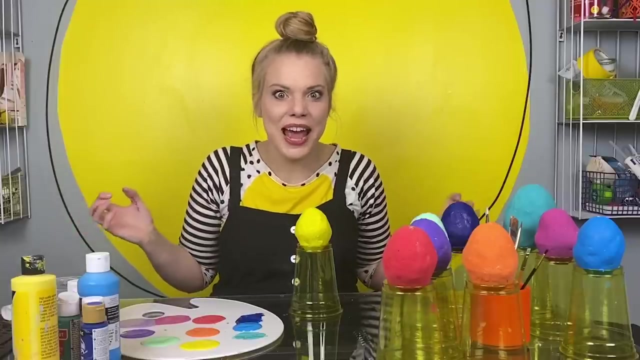 going to use to paint these eggs. I'm gonna start with a base coat on each of my eggs and when that dries I'll add more details. Let's make it Yellow, Orange, Red, Purple, Blue, Light green. Now it's time to add some details. You can do anything you want, and 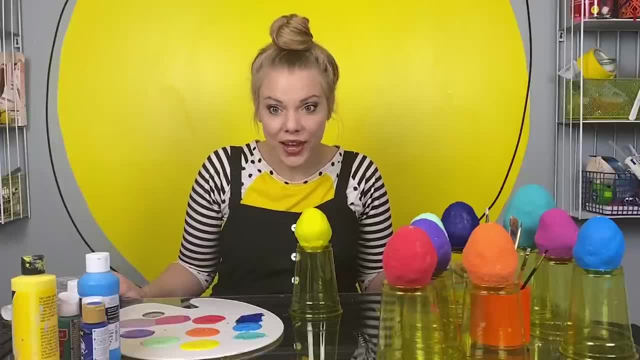 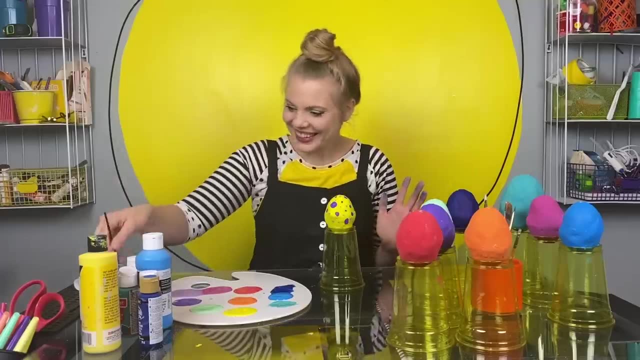 let your imagination go wild on this one. For my yellow egg, I'm going to use purple, because that's the complementary color that I'm going to use to paint this egg. I'm going to use a complementary color to yellow. for my orange egg, I'm going to 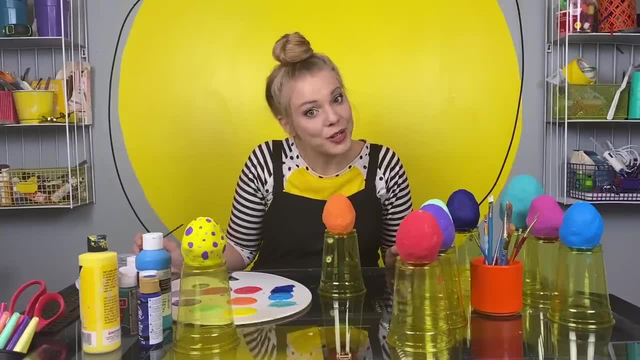 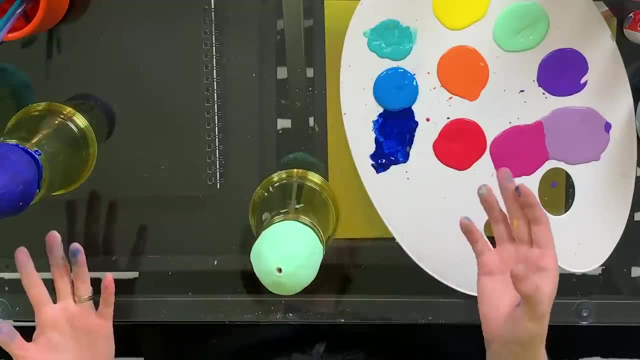 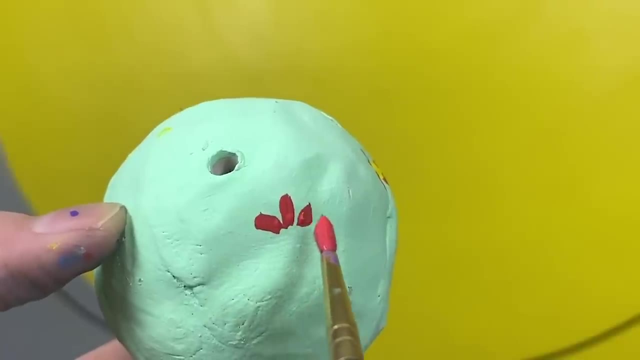 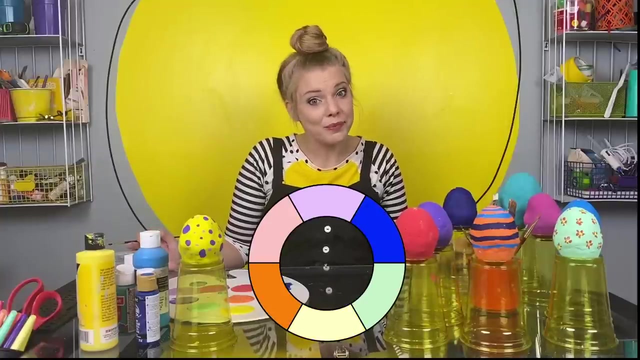 decorate it with blue, because blue is the complementary color to orange. Ta-da, On this green egg, I'm going to use red, because red is a complementary color to green. That's all the complementary colors: Purple and yellow, Orange and blue, Red and green. Let's keep decorating. 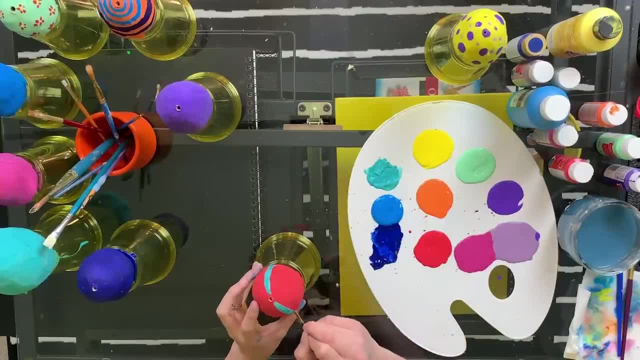 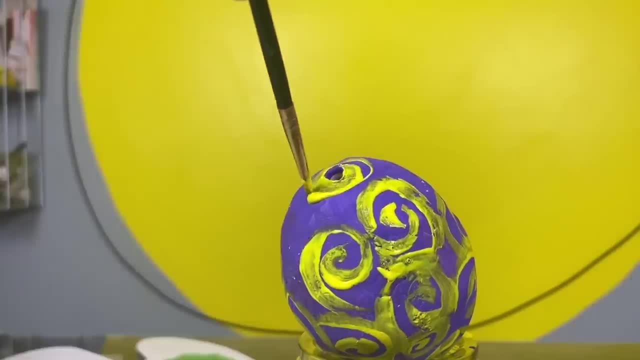 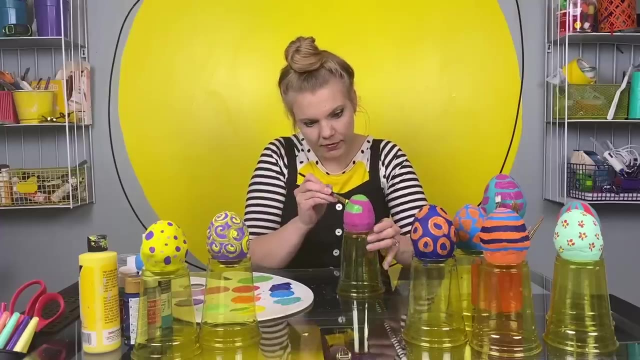 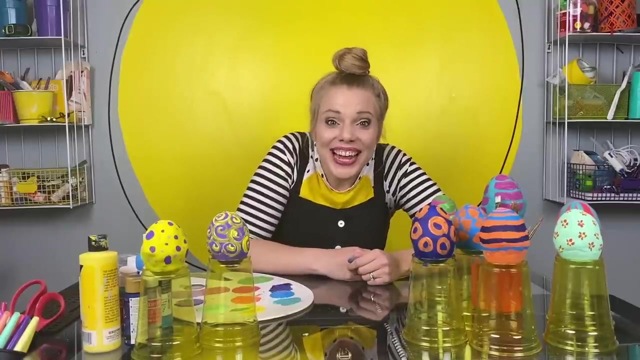 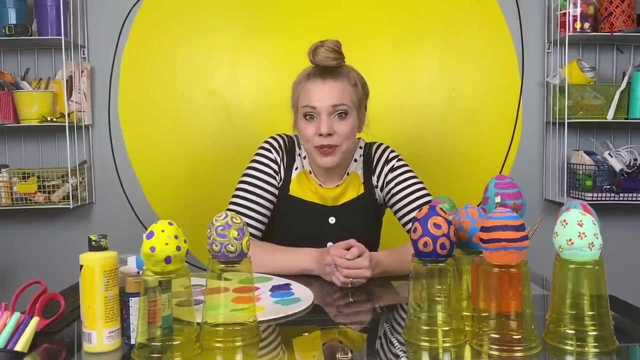 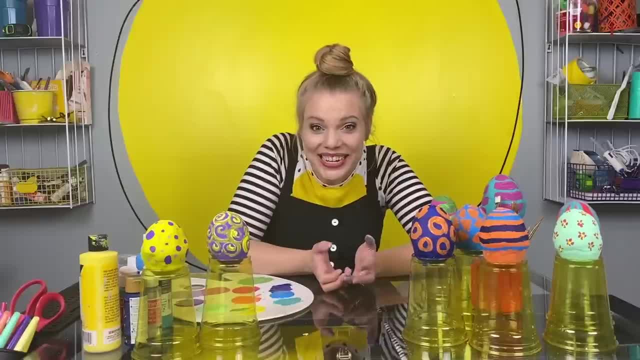 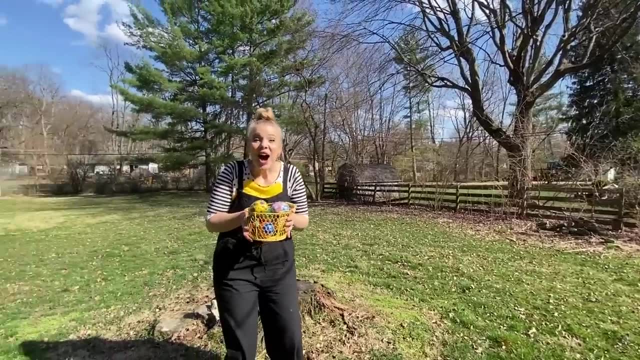 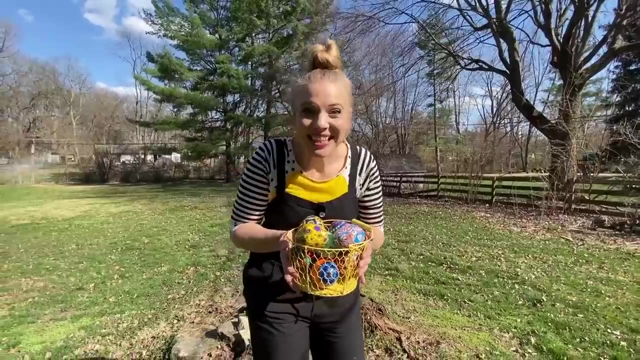 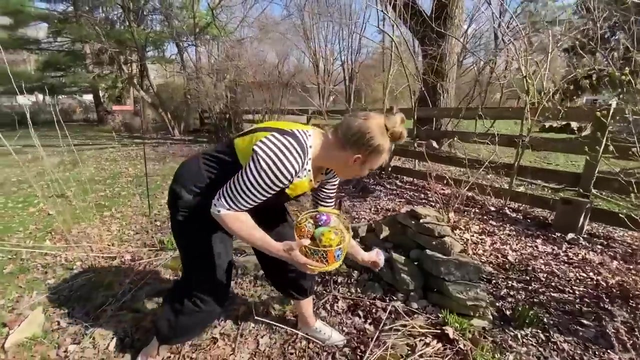 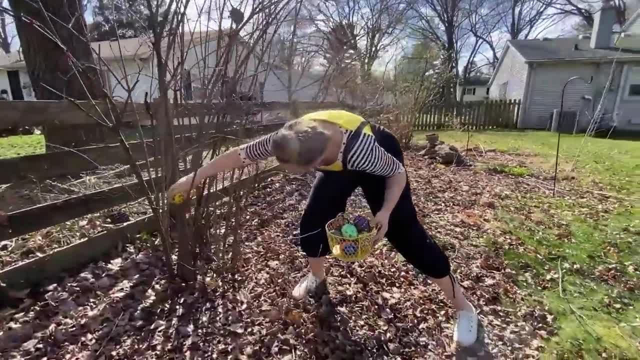 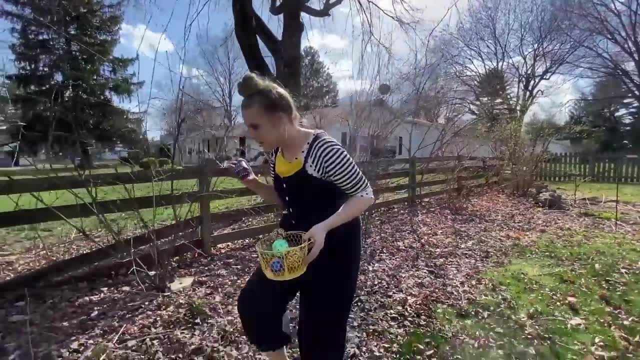 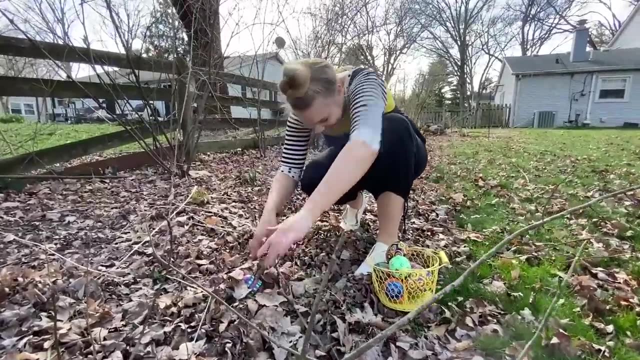 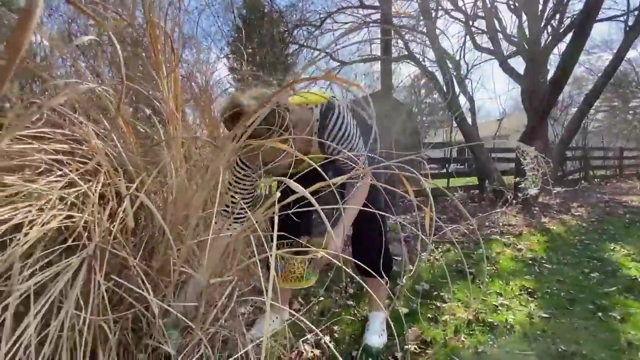 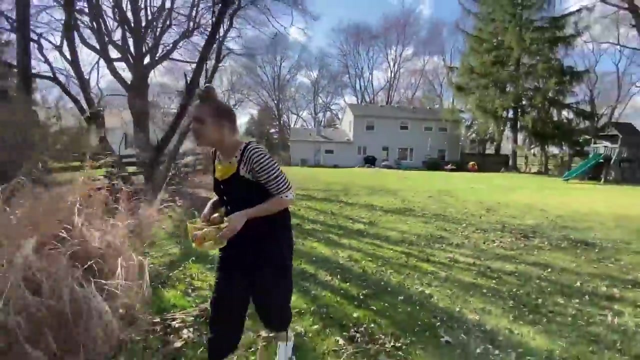 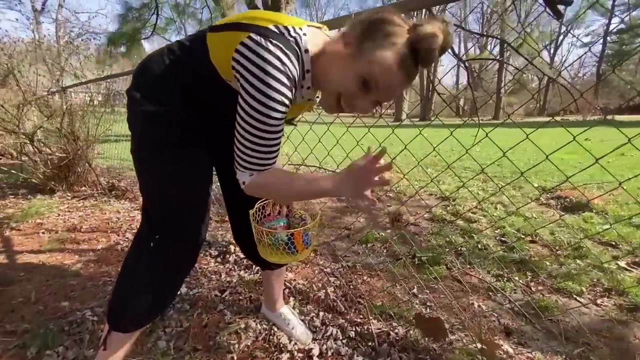 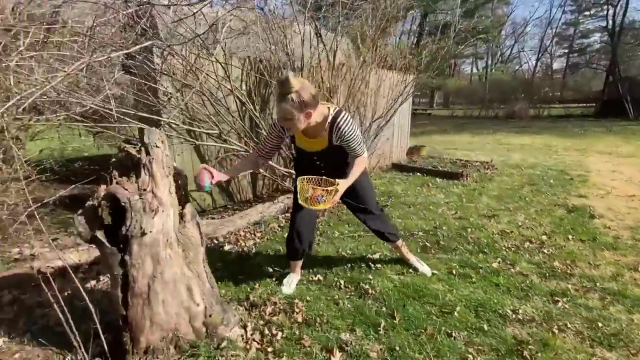 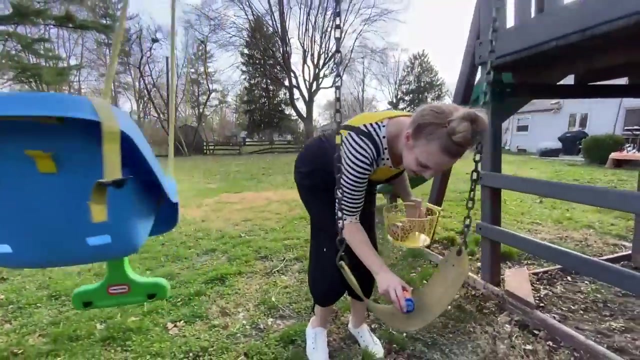 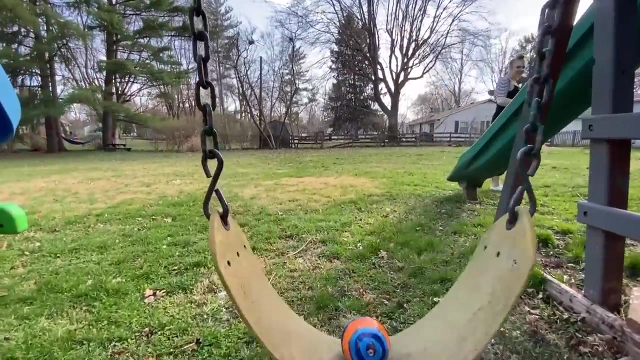 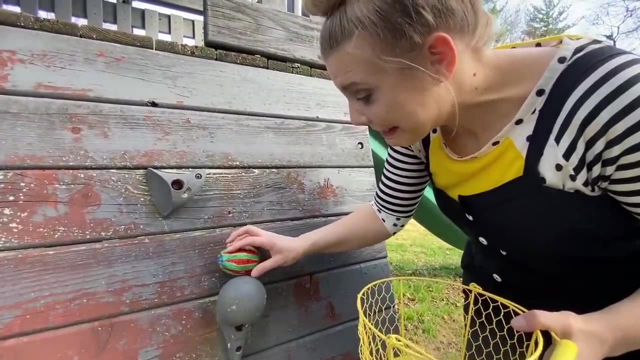 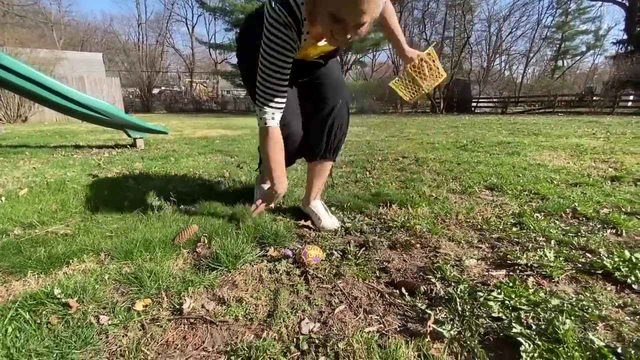 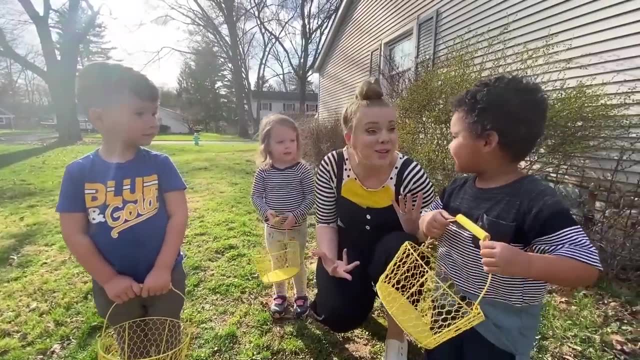 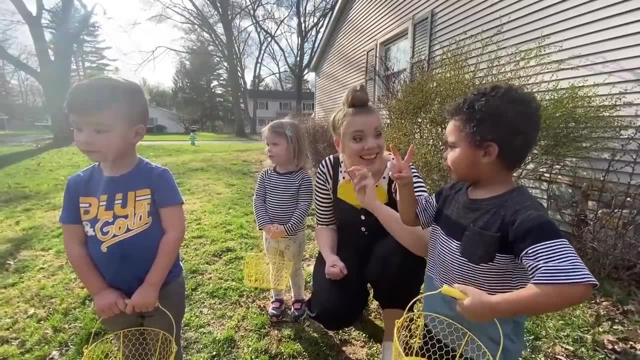 I'll see you guys in the next video. Bye-bye. I'm here with my friends and we are so excited to find some Easter eggs, aren't we? Let's do it Ready. One, two, three, Let's go. 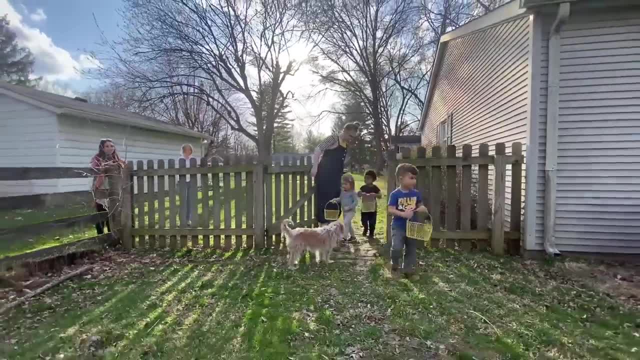 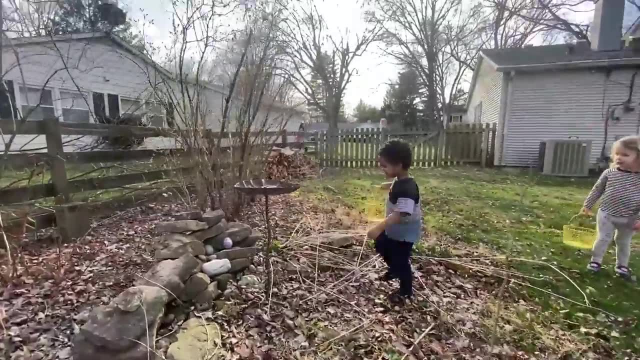 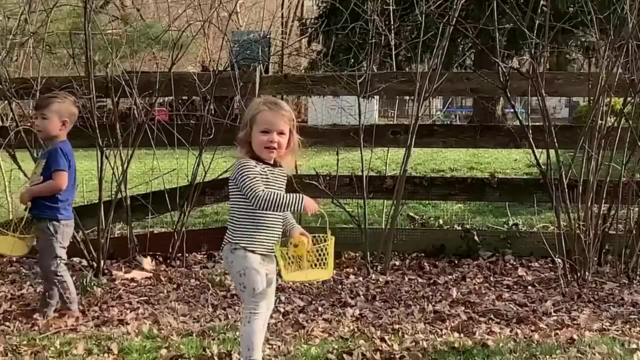 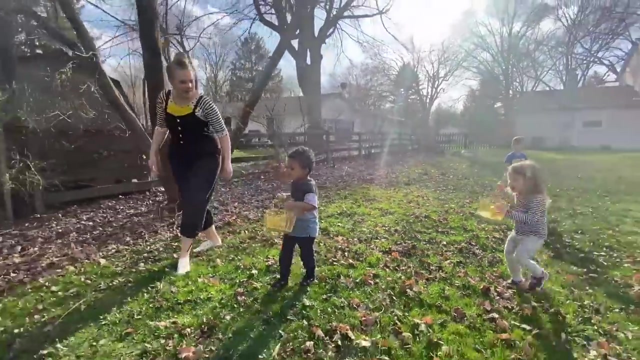 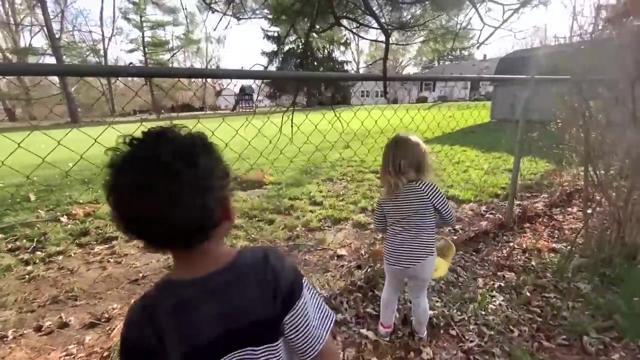 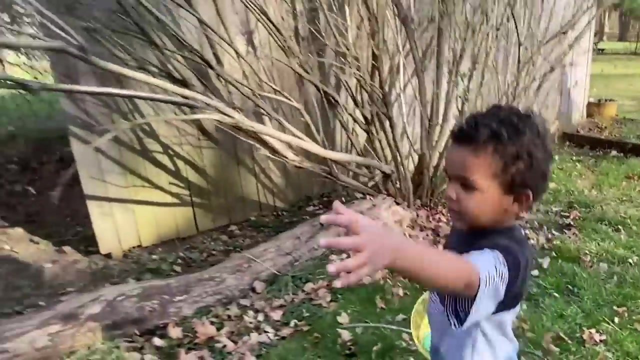 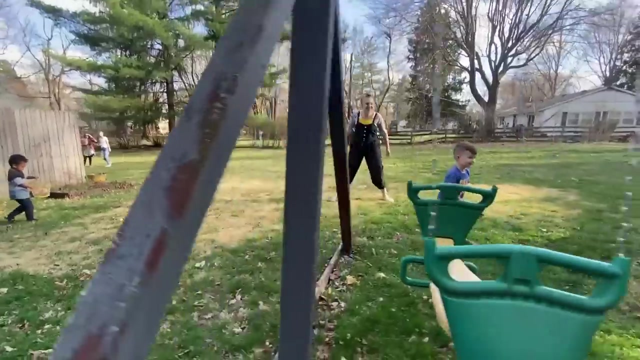 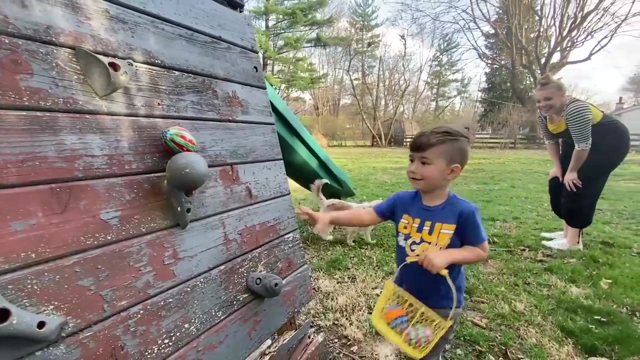 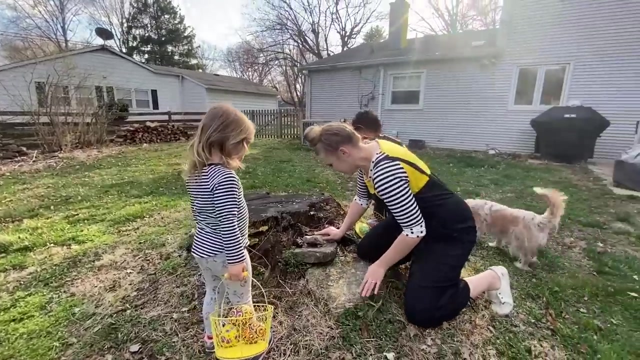 Let's do it Ready. One, two, three, Let's go. Can you see it? Woo, Yes, that's the last one, Come on. This part is very exciting Because we have to smash them to get the toys out. 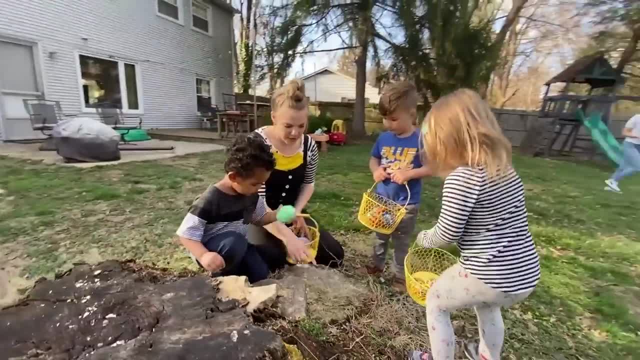 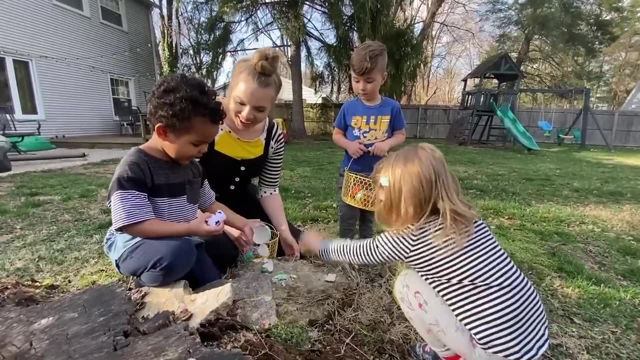 Just smash them. Yep, Which one do you want to open up first? Dax, This one. Okay, put it right here on the rock. Oh yeah, you can smash it that way. What's in there? A cow. 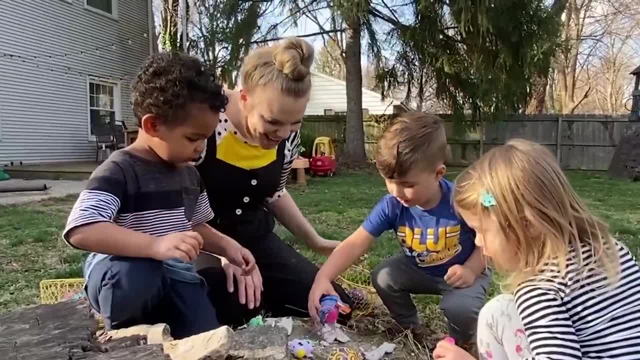 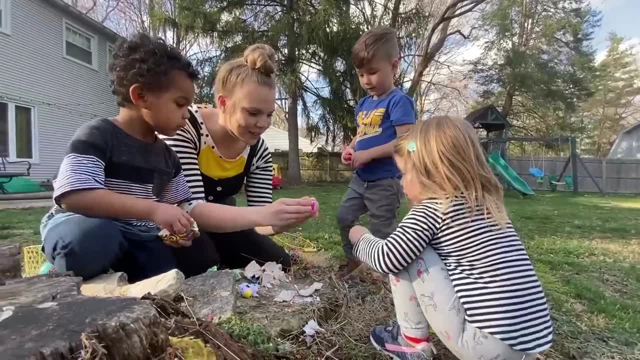 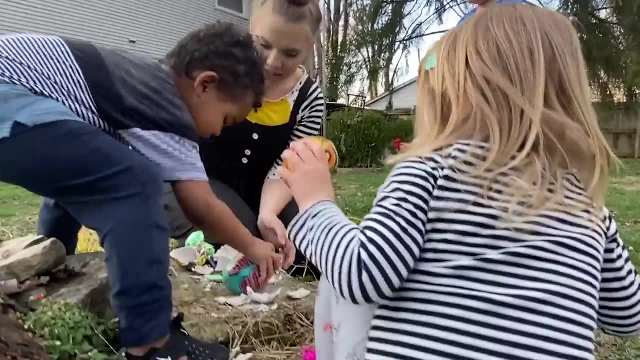 What's in there, Frank? Yeah, what's in there? There's something in that Silly putty. These are like rings that go on your fingers like this: Hello, Hello, Oh nice to meet you, Smash, Smash. 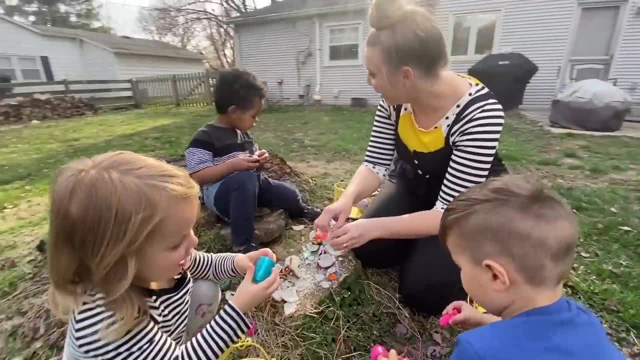 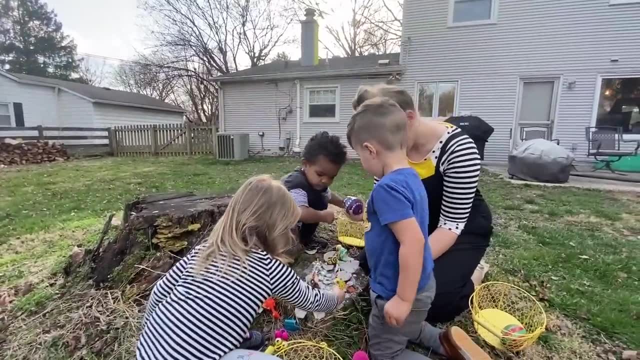 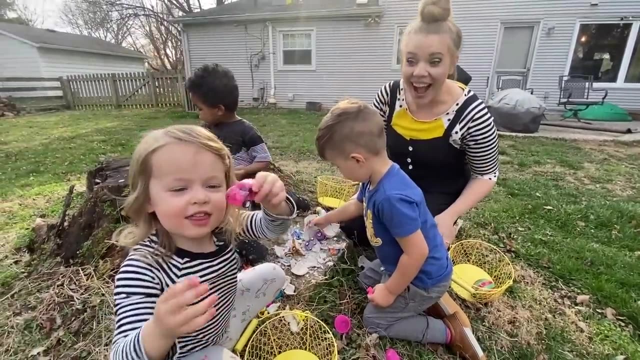 Oh, a slinky. Yeah, Woo, I need to do this one. Look it, Woo. Look what hopped out of your egg, Frank. look A new car. And you got a car too, A purple one. 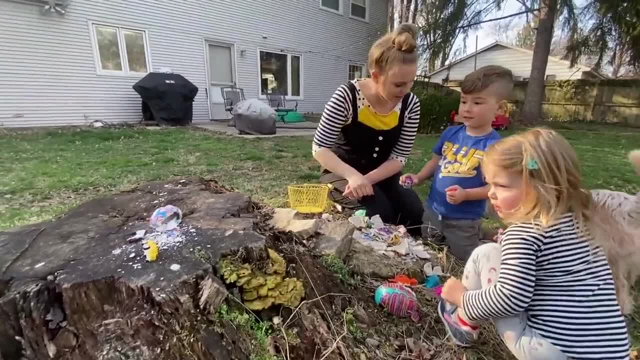 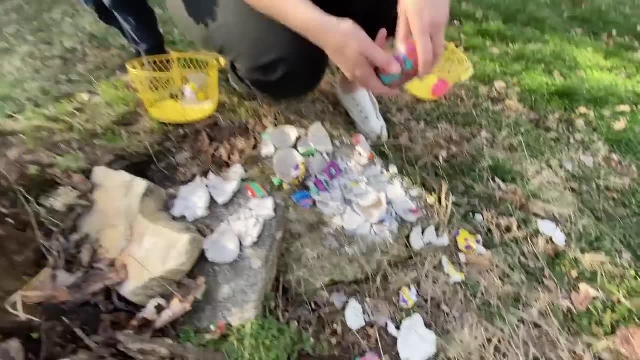 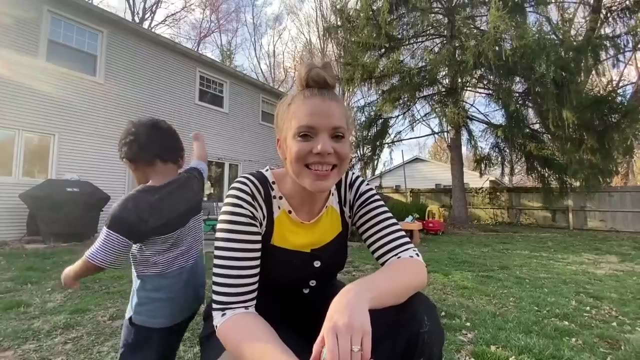 And Dax got a yellow car. You guys should race. Oh perfect, Look A stretchy dinosaur. I got to get JoJo. That was so fun opening up these amazing eggs with our friends And it was so fun making these eggs with you. 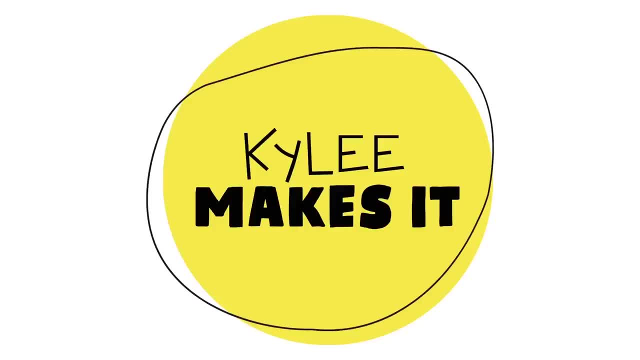 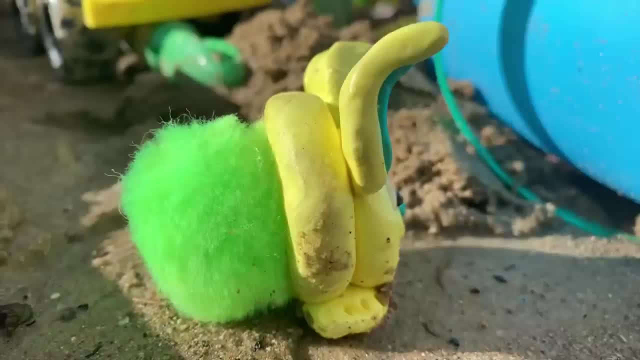 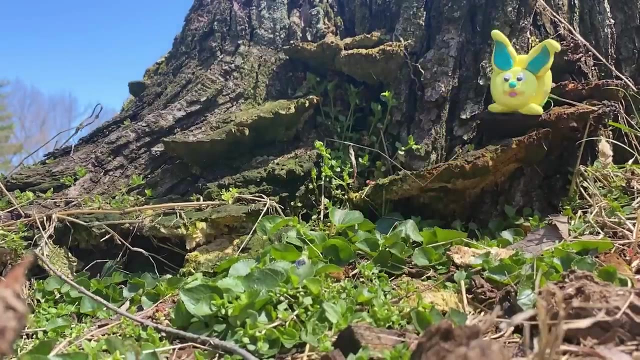 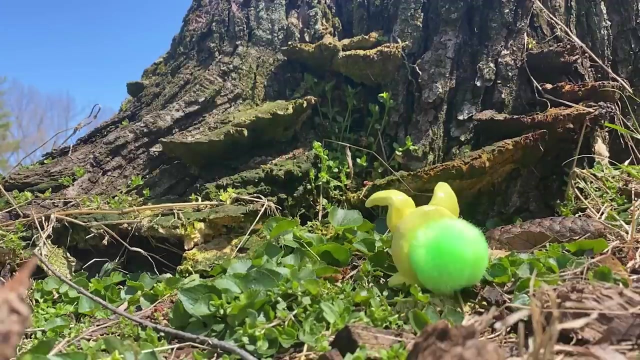 I'll see you next time. Kylie makes it. Hello, I am a bunny And I have journeyed far and wide to find the largest character, The largest carrot on top of the largest mountain. I'm here, Whoa A rope. 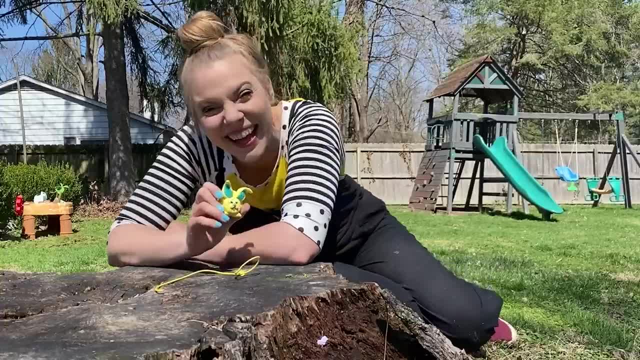 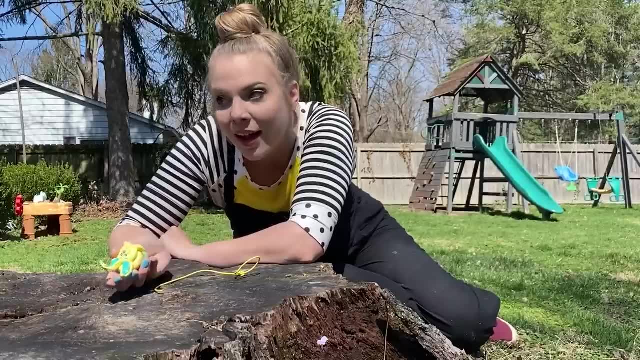 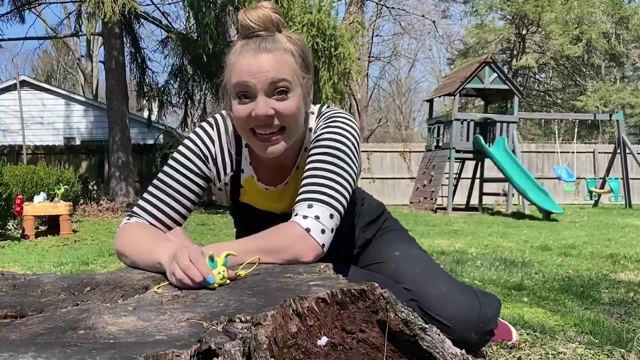 Someone's come to help me. Hi, My name is Kylie And I made this little rabbit today out of polymer clay, So I just had to come outside and try it out, See if it was good to play with. right Turns out it is. 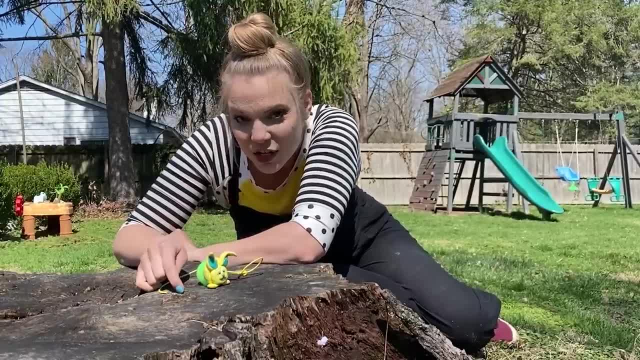 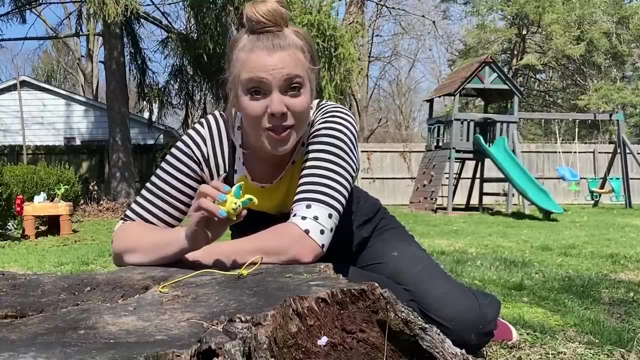 I'll come back and finish this story with you, But first do you want to learn how to make your very own polymer clay rabbit? Let's go to the studio and I'll show you how to make your own rabbit so you can tell your own stories. And then we'll finish this one up. Come on To make your polymer clay bunny. here's the things you're going to need: Polymer clay. If you don't want to use polymer, that's totally fine. You could make this with air-dried clay or Play-Doh or any kind of clay really. 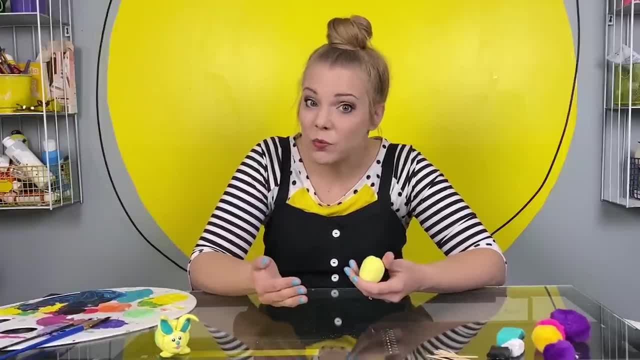 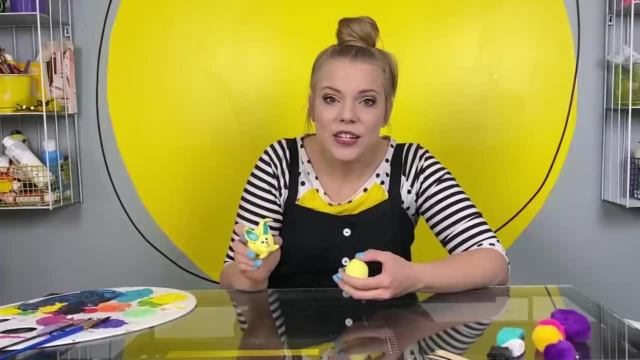 It'll just depend how you finish it and how strong it is once it's done. I chose polymer clay because it's really easy to use and once you bake it it's hard And you can bake it in your oven, So it's really easy. 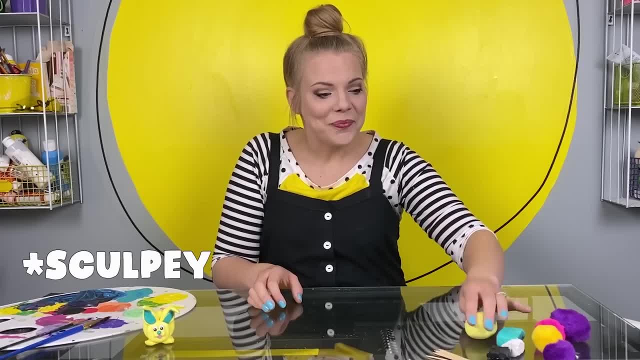 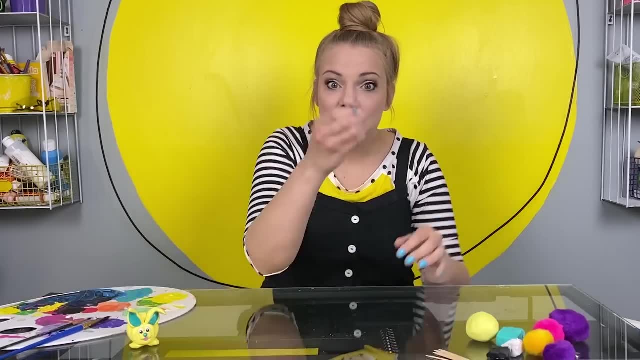 Polymer clay. My favorite brand is Sculpey. If you want to put a puppy tail on your rabbit, you're going to need some pom-poms, Toothpicks, And I used a little bit of paint and a little bit of glass for mine, but you wouldn't need that part. 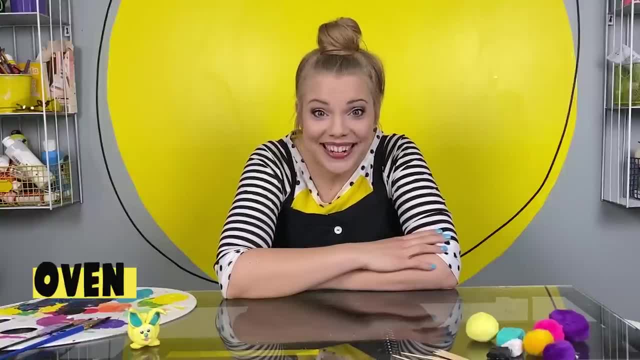 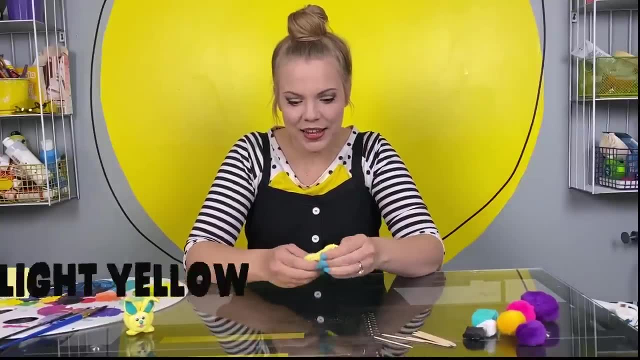 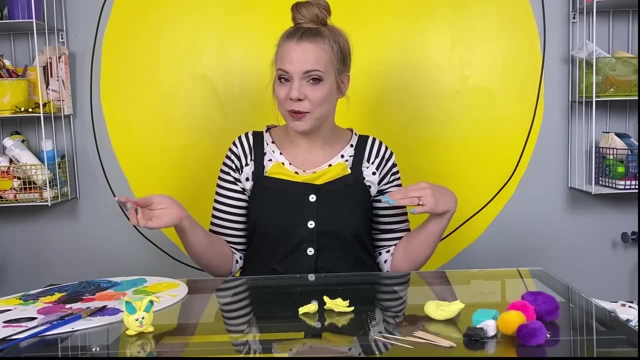 You'll also need an oven. Are you ready to make it? Let's do it. You can make your bunny whatever color you want. I'm going to use this light yellow. Break off two balls of clay, Just like that, One a little bit bigger and one a little bit smaller. 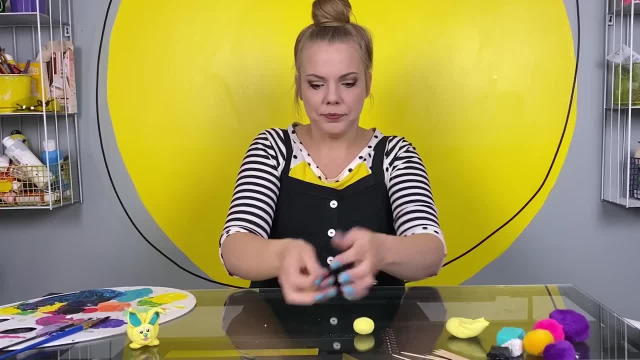 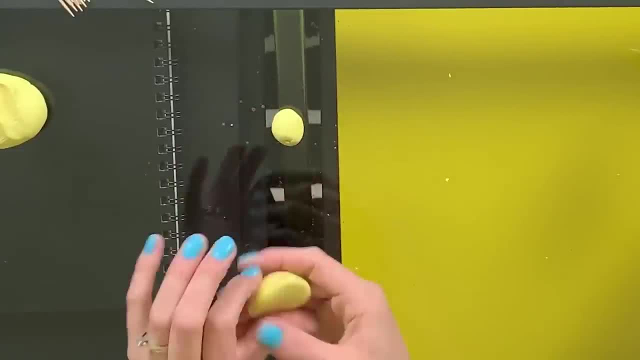 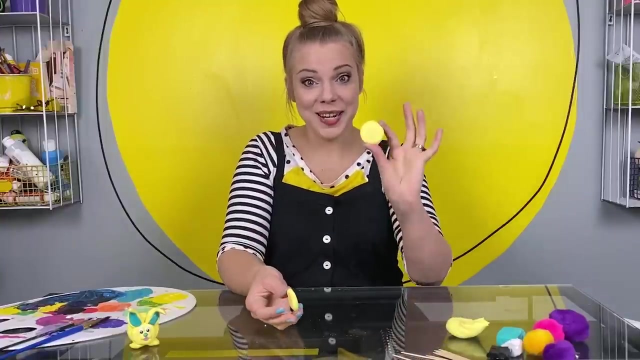 Roll them up. Now I'm going to take it in my hand and just flatten it a little bit. This will make the spheres, or the balls, into circles or discs Next Great. Now one is going to be the body and one is going to be the head. 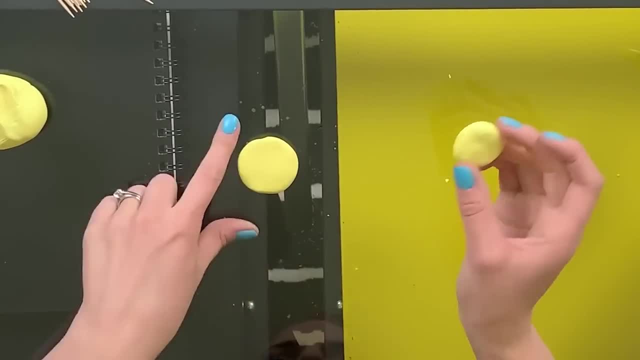 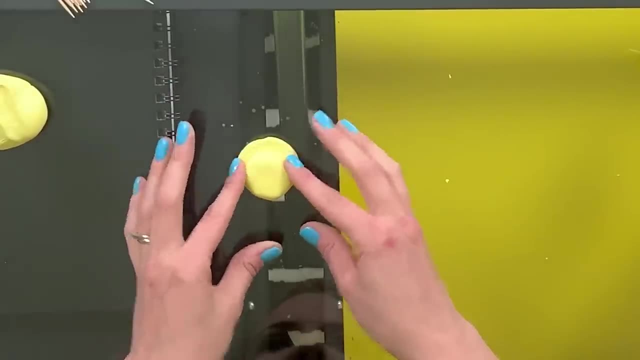 You can put this down flat to work on it. Put your body down first and then attach your head. Give it a little spin, Swoosh- You don't need to go super hard. Great. Next we're going to make the ears of the bunny. 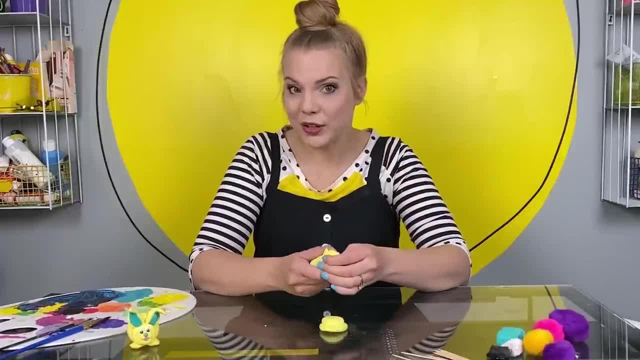 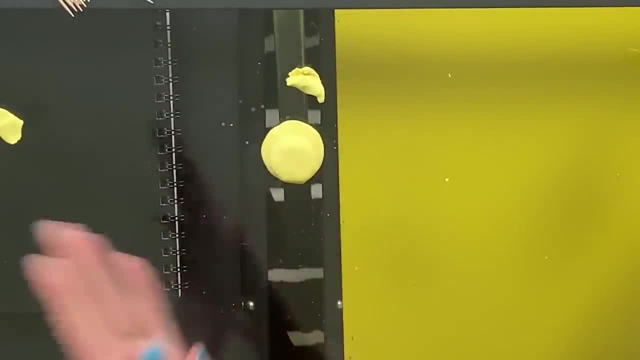 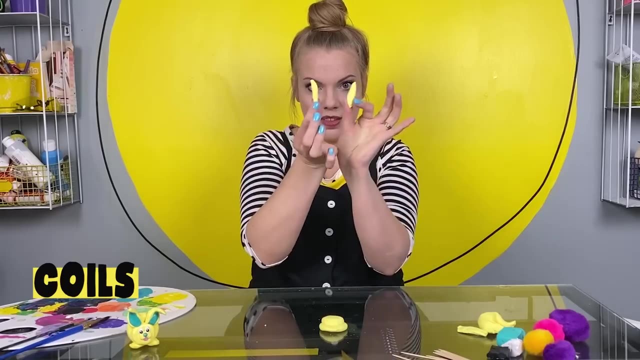 My favorite part: Take a little bit more of whatever color you want and break off two equal pieces. If you want your ears to be really big and really long, use more clay. I'm rolling these into coils, Then I'm going to slightly flatten them with my fingers. 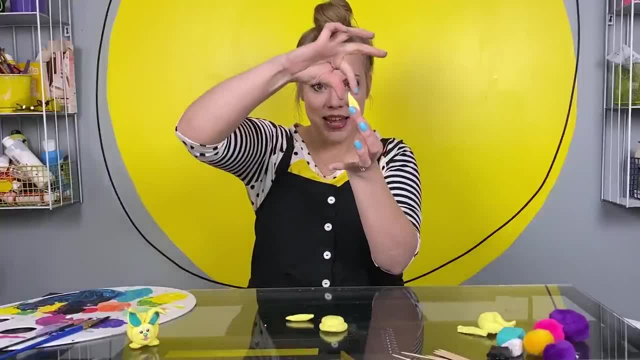 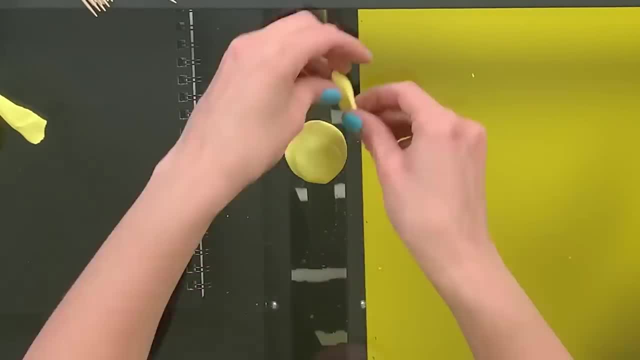 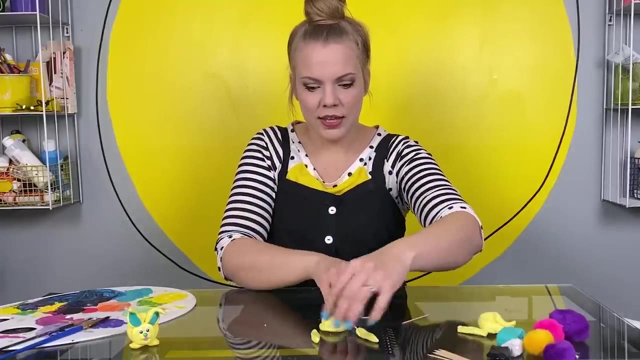 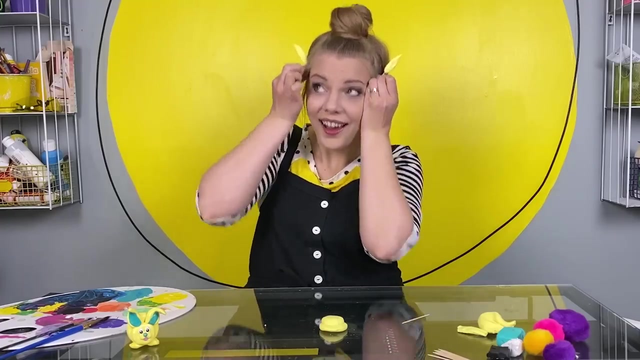 Just by pinching them And make the ends of each coil into a point Like that. I'm going to break a toothpick in half And I'm going to put each one in the end of each ear. Now I'm going to take my ears on toothpicks and put them into the coil. 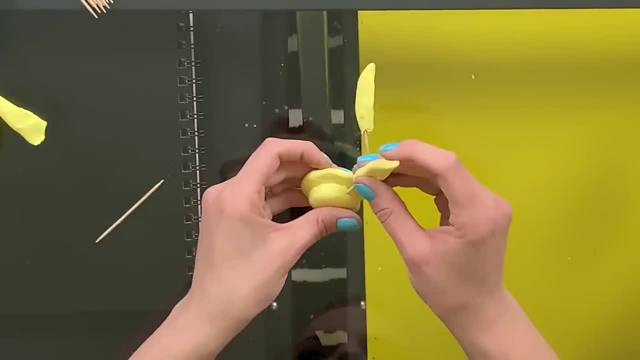 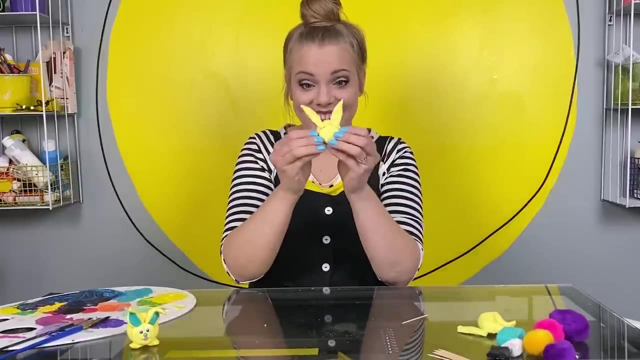 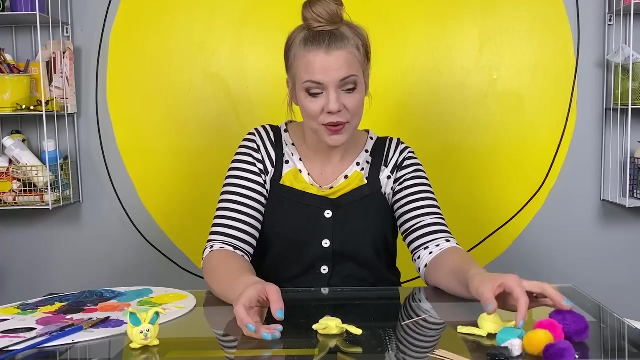 And put them into my bunny's head. This will make sure that they stick and stay up, Starting to look like a bunny right Now. if you want to put some color on the inside of your rabbit's ears, go ahead and do that. 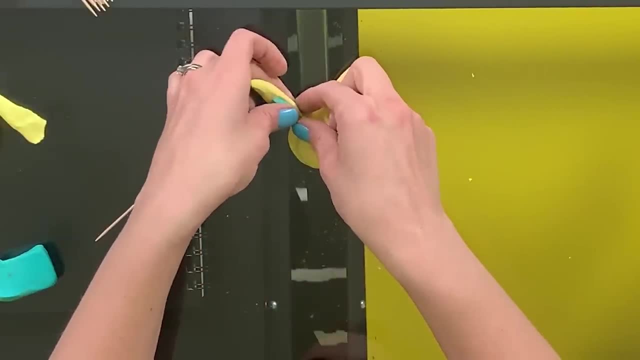 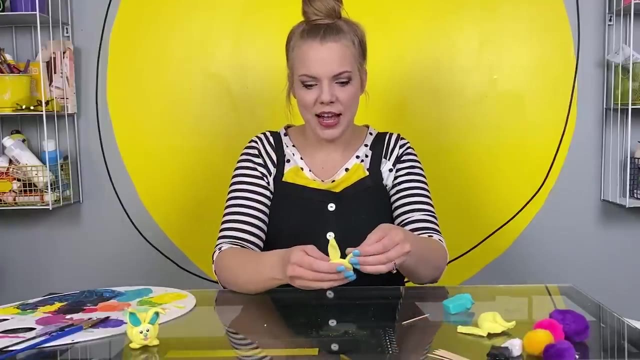 Then just stick it right inside your ear And you're just going to press that together lightly. You can bend your rabbit's ears to give it a little bit more personality. I think I'm going to flop one down a little bit Like that. 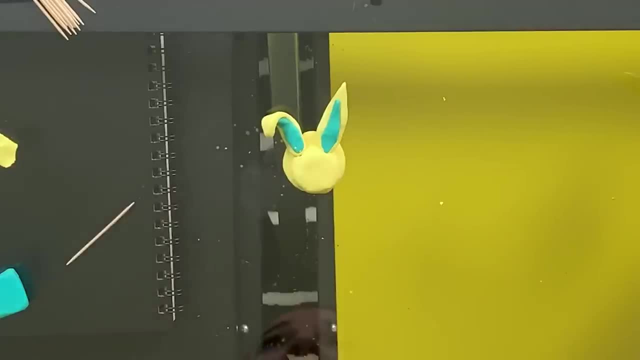 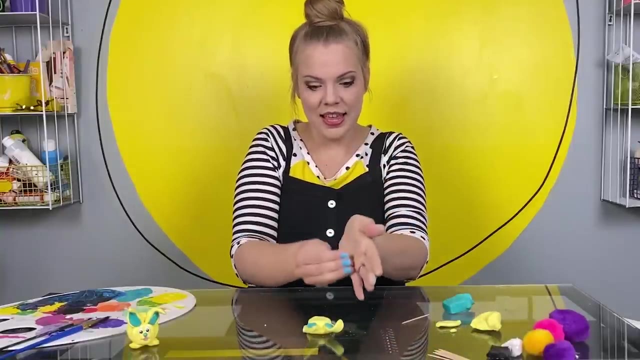 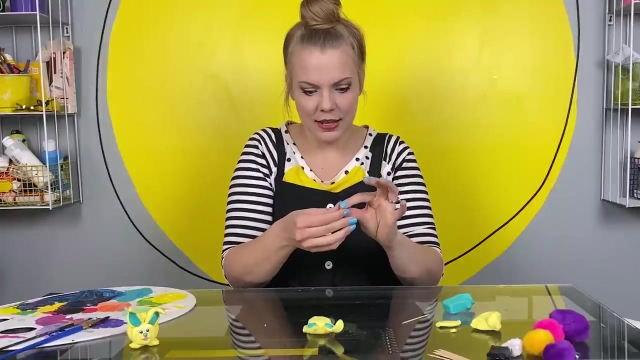 Just one, though Time to make the face. I'm going to take a very little bit of clay and roll it into a ball. Then I'm going to shape it into an oval and flatten it just a little bit. This will be the cheeks of our bunny. 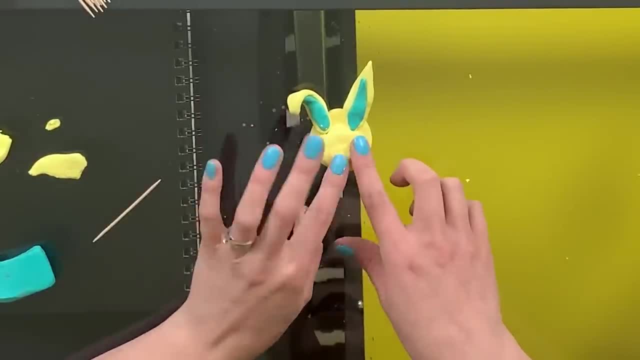 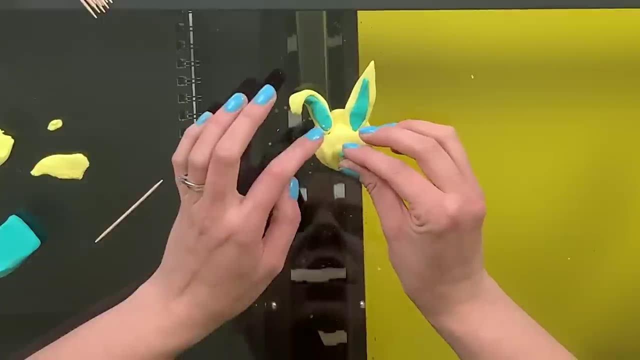 I'm going to put it right here And then I'm going to make a little nose to put it right on top. I'm going to use this teal color. You can use whatever color you want, Put it on top and give it a little smush. 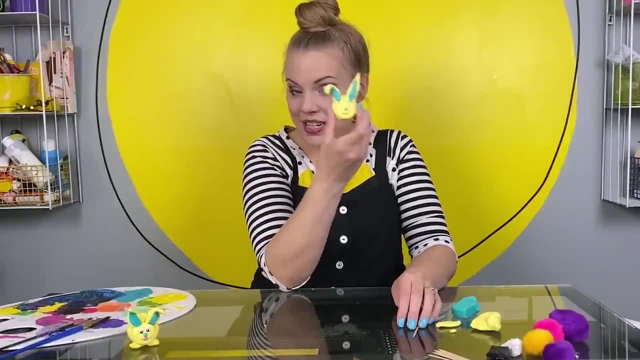 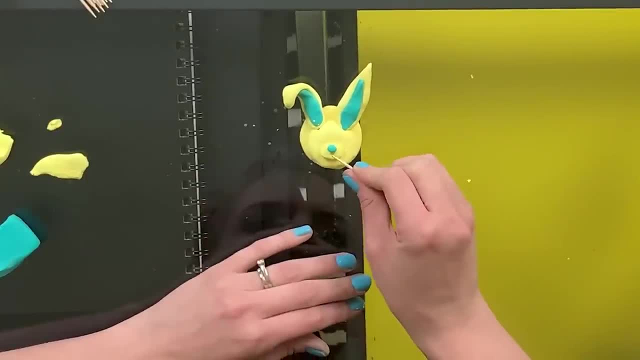 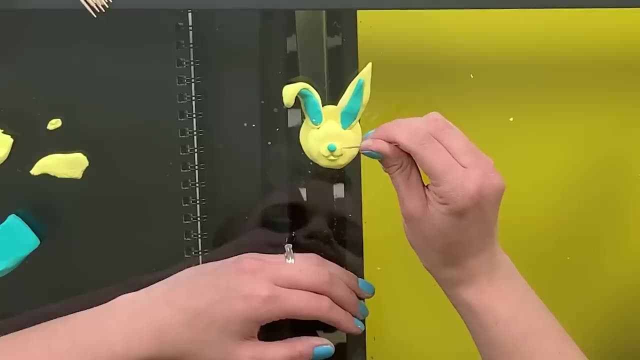 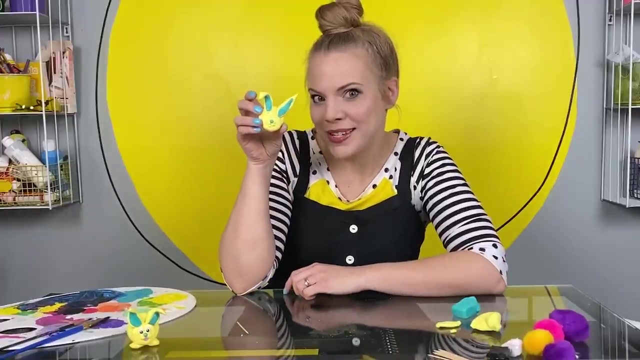 Now that you have your little cheeks and your nose of your rabbit attached, use a toothpick to make a mouth Great, And then I'm going to make some holes in this so it looks like places for whiskers. What is this rabbit missing? 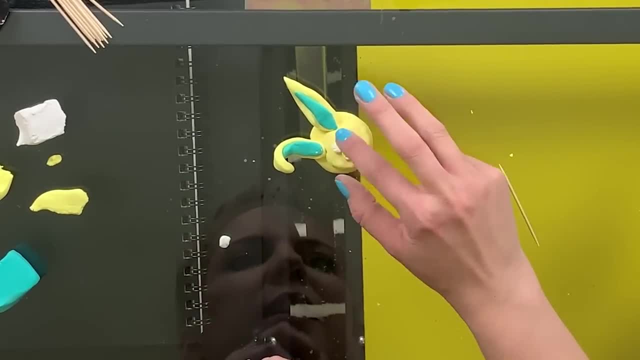 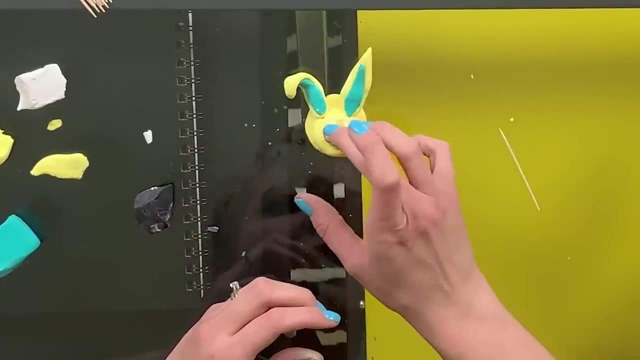 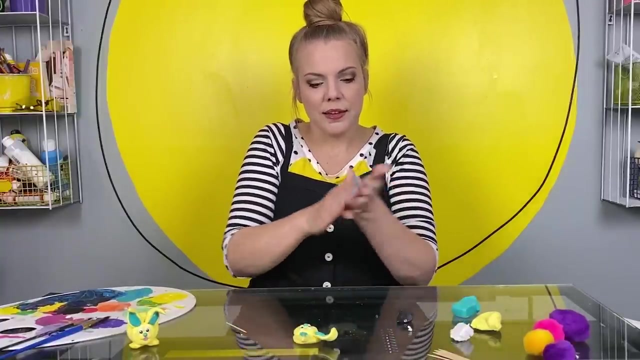 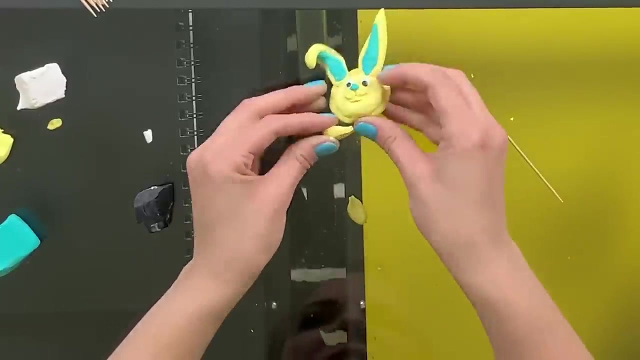 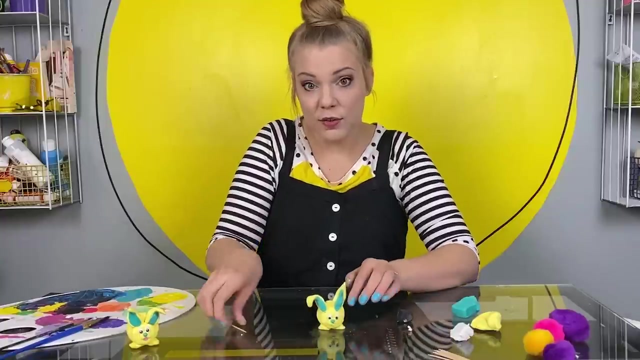 Eyes. The only thing left to make with clay is the bunny's feet. So take a coil, Break it in half And attach it right to the underside of your rabbit. Great, You can also use your toothpick to make little lines to make it look like your bunny has toes. 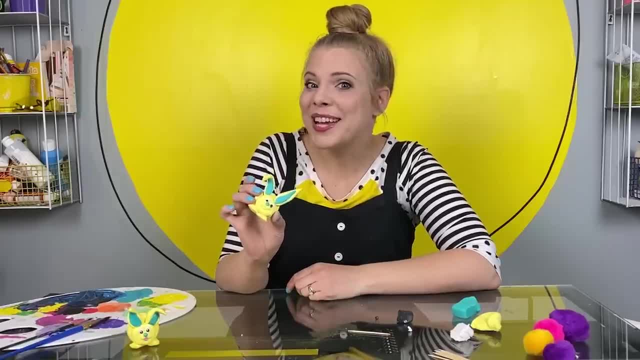 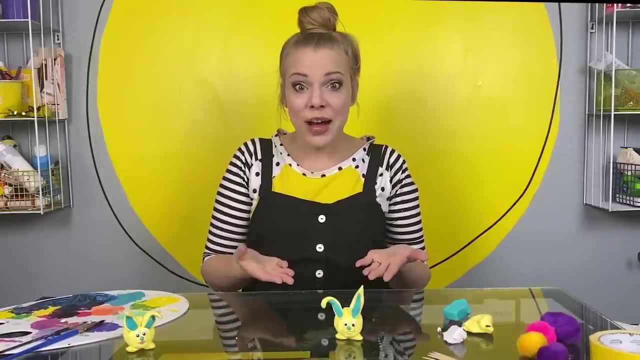 The kind of polymer clay that I used for this project needs to bake at 275 degrees for 15 minutes, So I'll see you in 15 minutes. The bunny is out of the oven, and now we can add a few more details with paint if you want to. 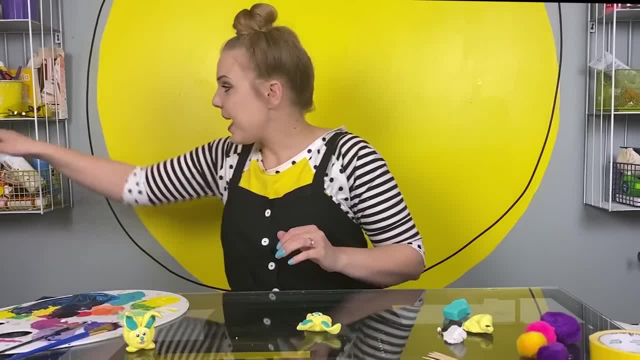 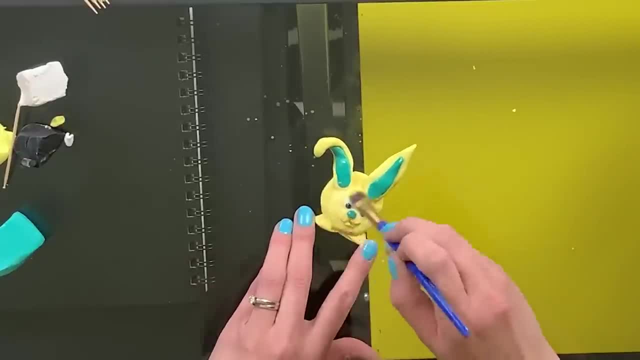 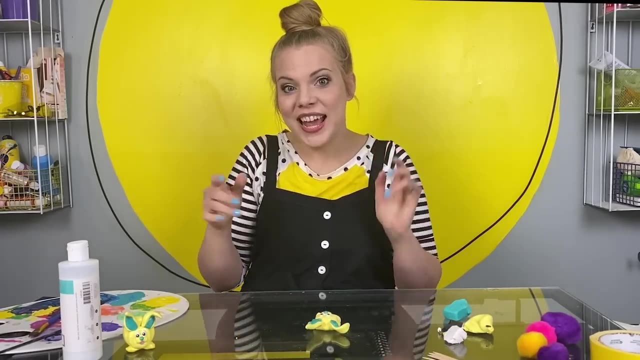 I'm going to flip mine upside down and add a little bit of a gloss finish. This just makes it look shiny. Add my gloss paint on And now I'm going to add some detail in the eye to make them look shiny, and a little tongue or mouth. 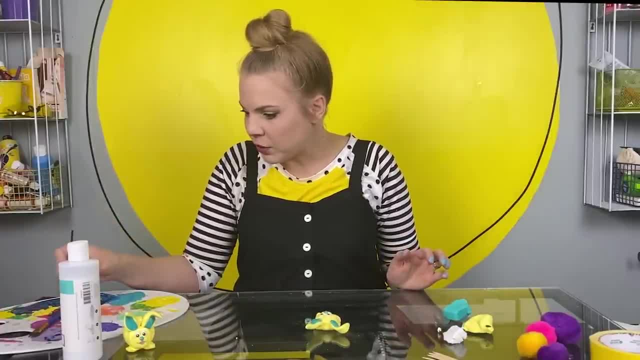 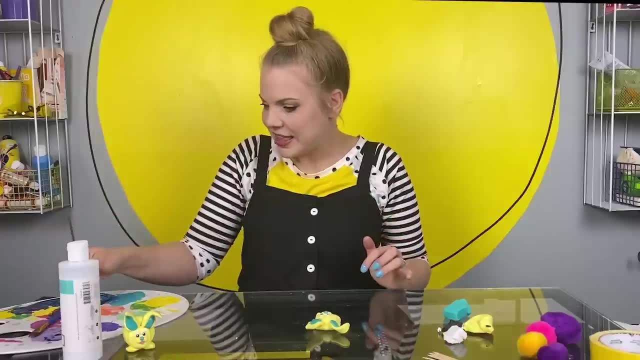 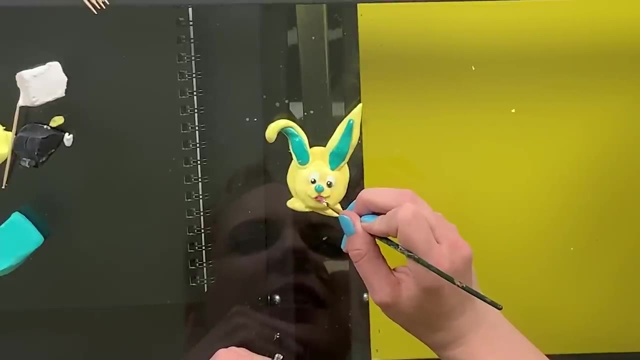 So I just have a little paint brush. I'm going to grab a little white paint, just the smallest dot And just boop boop. Then I'm going to take a little bit of pink paint and paint this little area right here by the mouth. 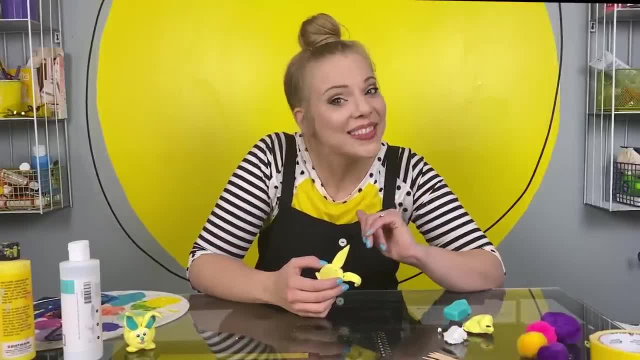 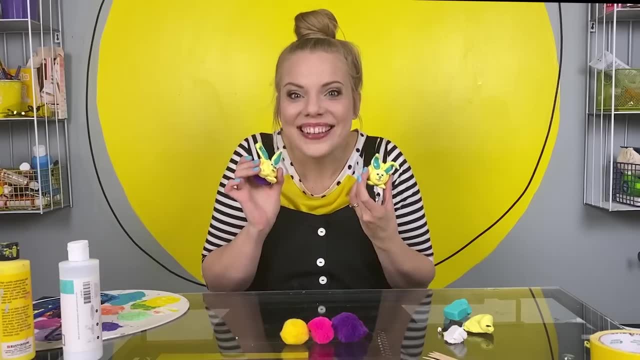 There we go, And now it's time for, I think, the most fun part: the big poopy tail. Now let's get back to our story. It's you, my long lost twin. Thank you for your help. 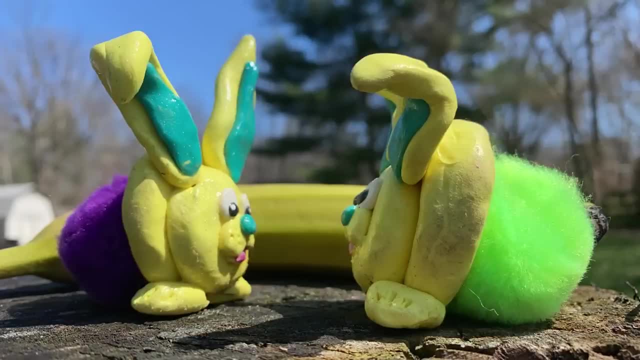 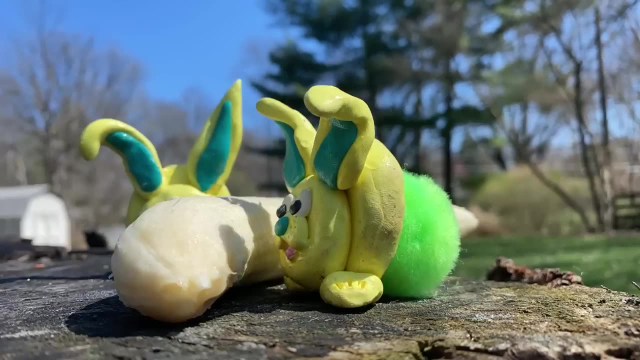 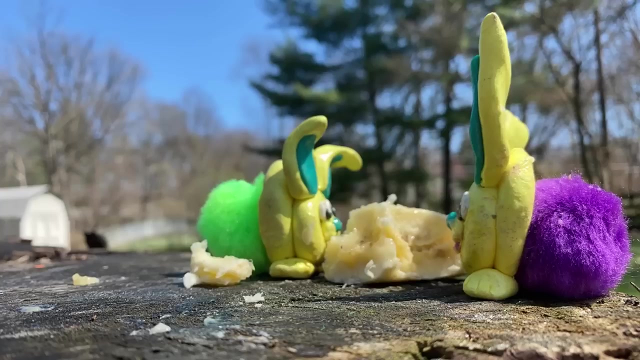 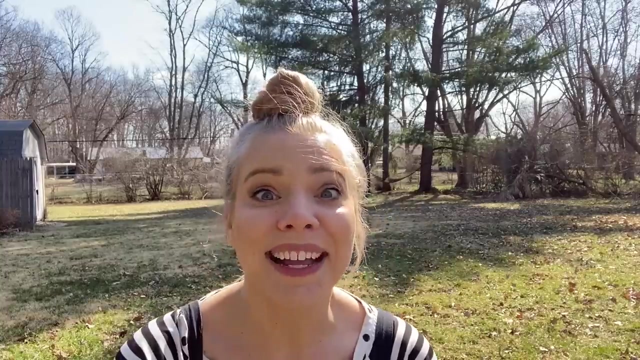 Now let's go get that carrot. Wow, This is a large and yellow and peely carrot. Nom, nom, nom, nom, nom, Delicious. Hi, it's me Kylie. Welcome to my backyard. It finally feels like spring out here. 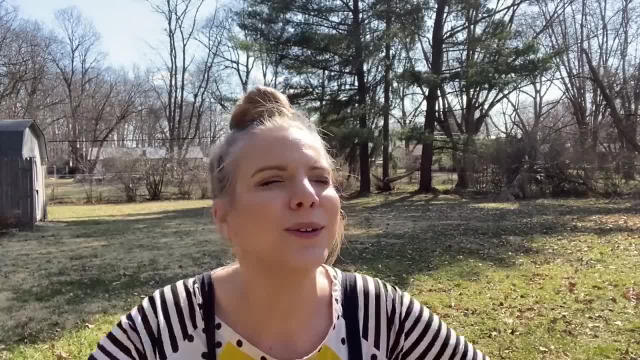 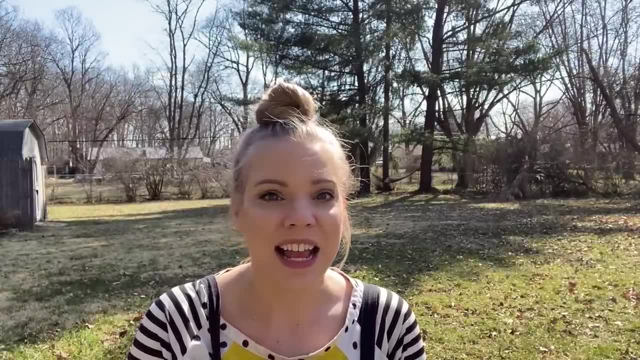 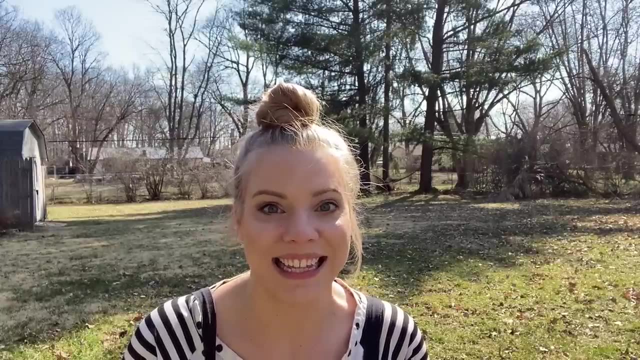 It's not technically spring yet, but, ooh, that sun feels so good on my face And I just found a sign of spring in my yard. It's the first thing every year that happens when I think spring is coming. Look at this. 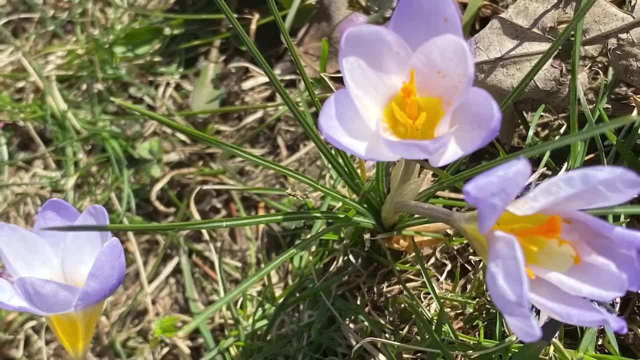 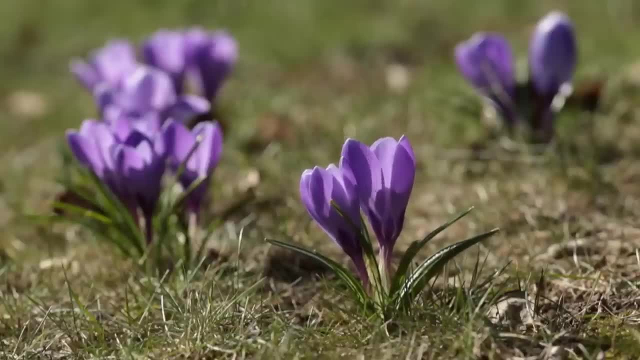 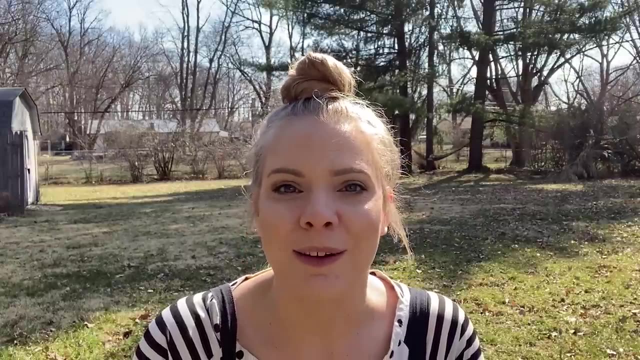 Little yellow flowers and purple flowers. I love them And every year they show up right here And it reminds me that spring and warmer days are ahead. I'm going to pick just one of these and bring it into my house, But these flowers are so special. 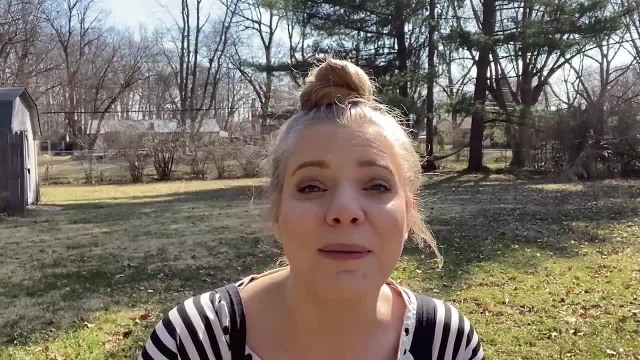 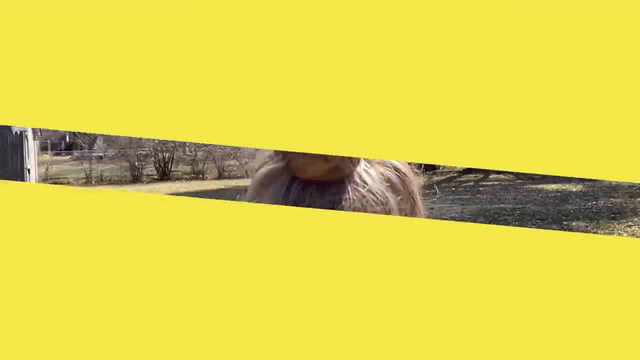 I think that you and I should make something special to carry them in once we pick the one that we choose. What do you think? All right To the studio. See you guys soon. Welcome to the studio. I am so excited to show you the craft that we're going to be making today. 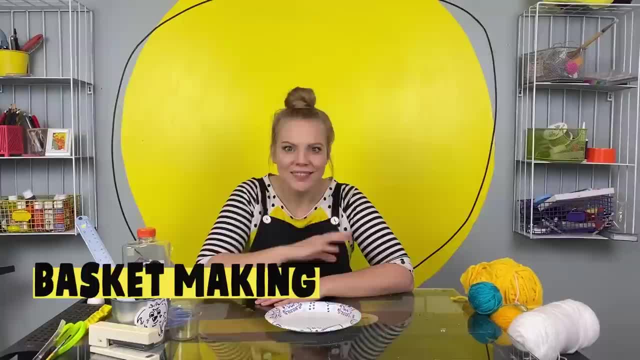 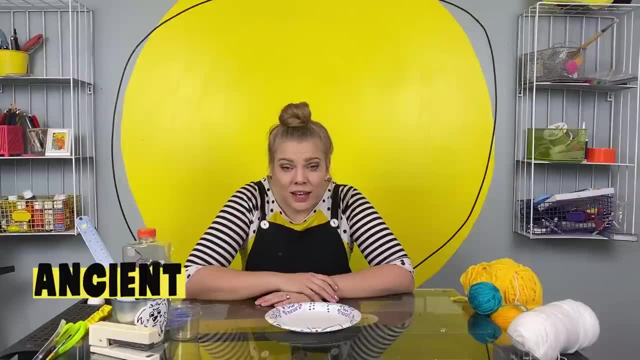 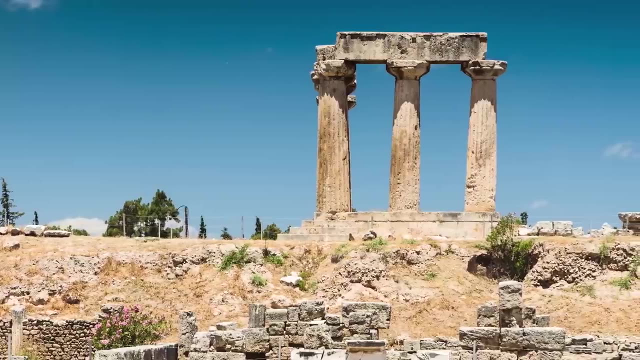 Because basket making or making a basket, is a craft that is ancient. Do you know what the word ancient means? It means super, super, super, super old, Like things that have been around for thousands and hundreds of thousands and sometimes millions of years. 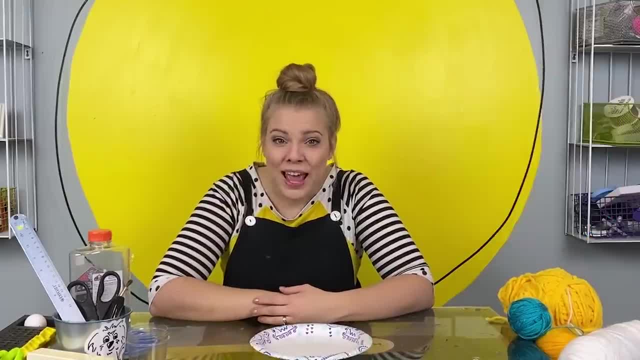 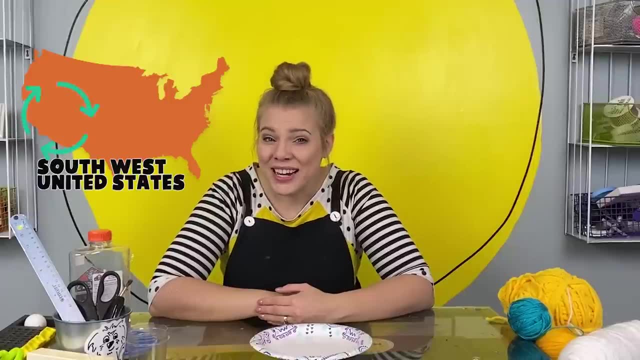 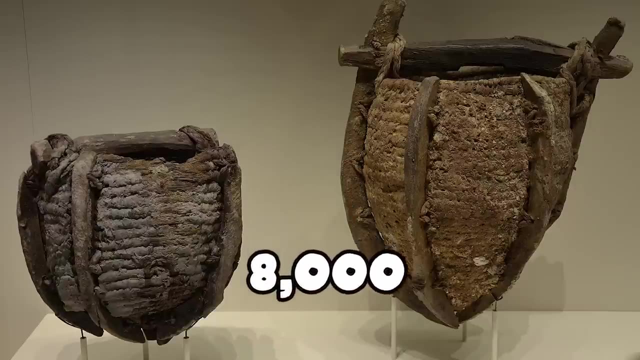 I live in North America And basket weaving has been an ancient craft and art form in North America For a long time. In the southwest United States they have found baskets that are over 8,000 years old. Here's the supplies that you need to make your basket. 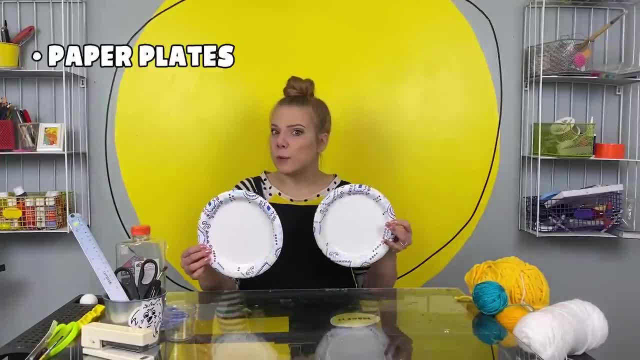 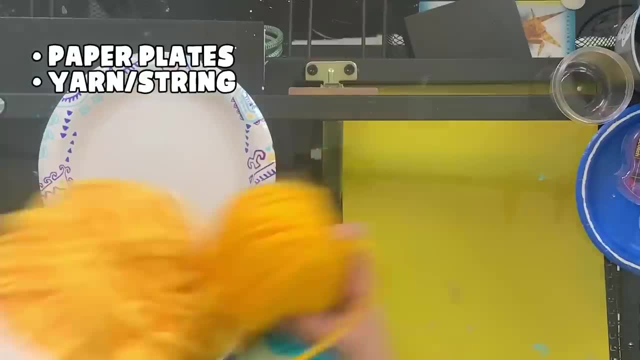 You're going to need one or two paper plates. Two, if you want to make a handle, Different kinds of yarn, string, ribbon, whatever kind of fibers you want to use. You're going to need some glue, A little bit of tape. 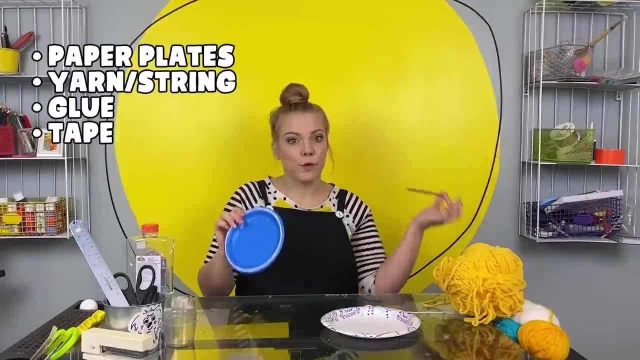 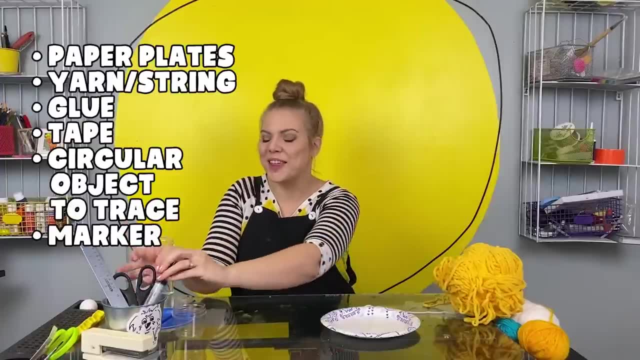 I'm using a plate and paint brush for my glue, But if you have glue in a bottle, that will work just fine. A circle shape: you can trace A marker or something to trace with Scissors. Ruler, Check, check, check. 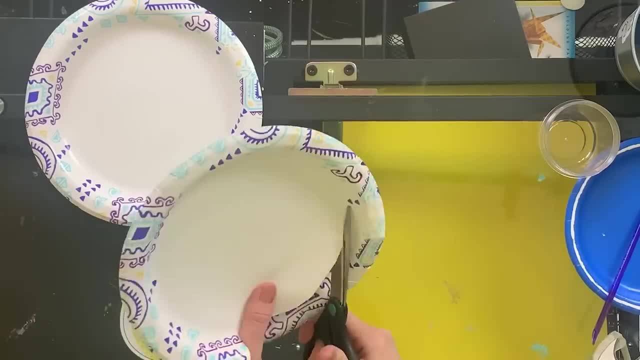 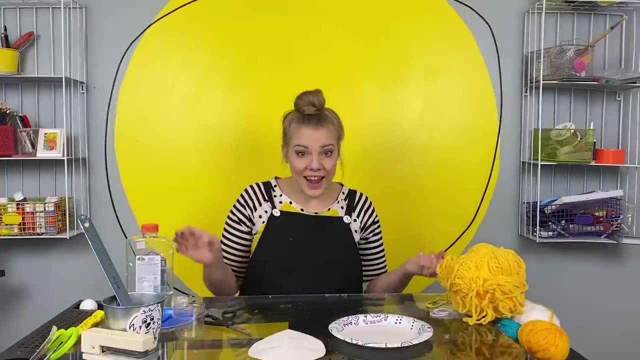 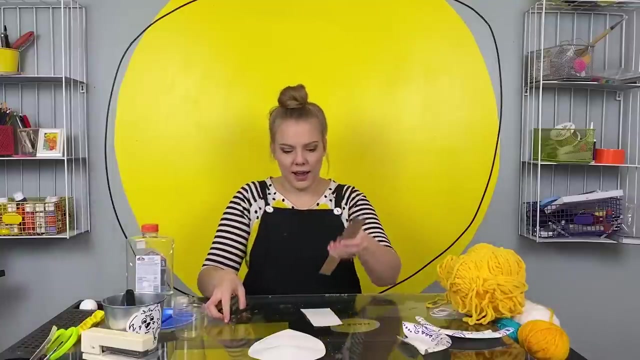 The first thing I'm going to do is to cut the rim of this paper plate off. There we go A nice round circle. Now I'm going to cut out the handle for my basket from my other plate. Now I'm going to use my ruler so that I can make these lines nice and precise. 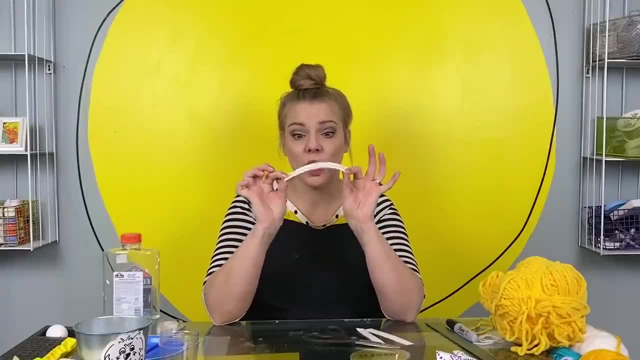 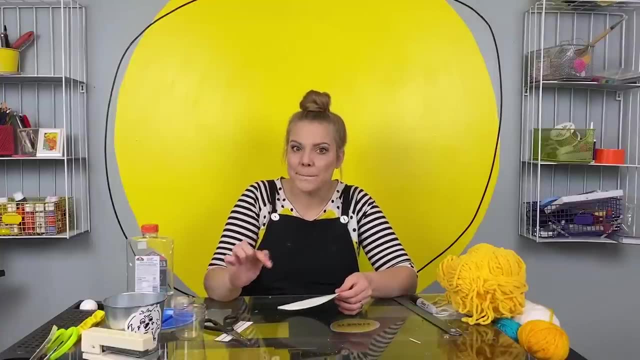 This will be the handle for our little basket. If you want a longer or bigger handle, you just need to use a longer piece of paper. Next, you need to choose the size of the bottom of your basket, So I picked this circle for the bottom. 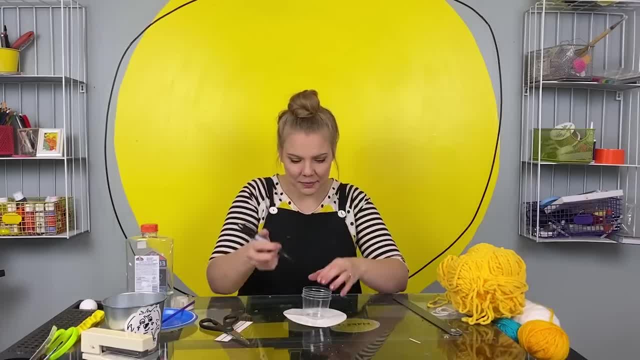 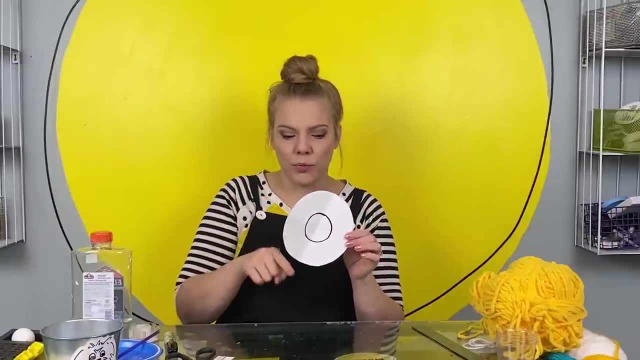 I'm going to put it right in the middle of my paper plate and trace it. Now that we have our middle traced, we're going to cut lines around the whole perimeter. That means the edge of our circle. This will create the walls of our basket. 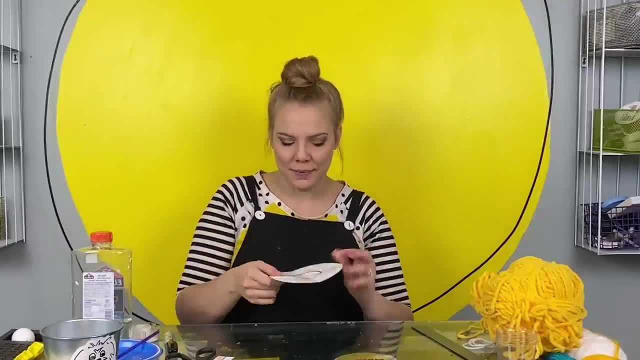 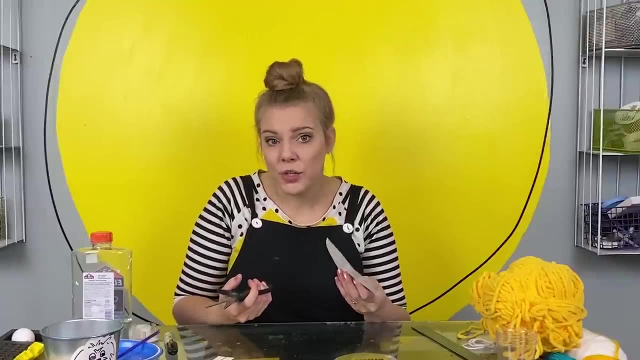 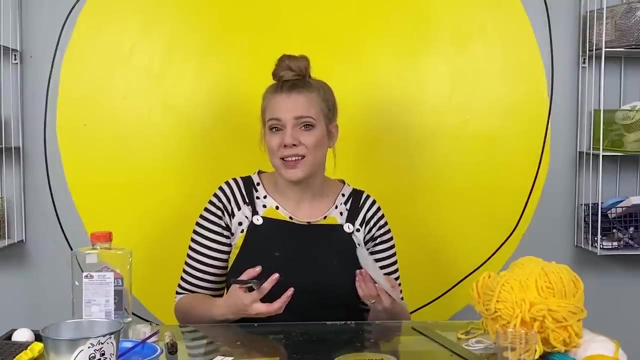 You might not be able to imagine this right away, but just stick with me. You can use a ruler to measure these out, but you also don't have to. They don't have to be the same width all the way around. If they're different widths, that might even look kind of cool, because you would get a different design of your basket. 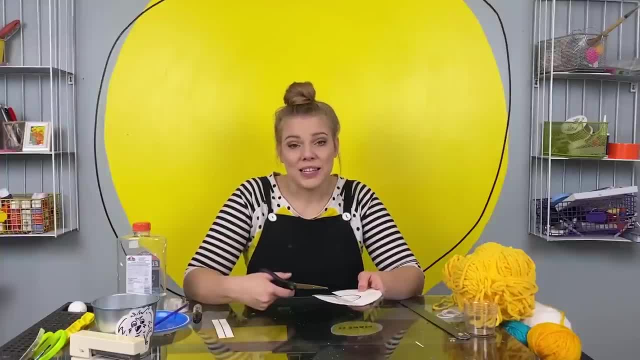 You get to pick. The only thing you need to think about as you make these cuts is that you make an odd number of sections. When I say odd number, I don't mean a number that's unusual, I mean a number that's not even. 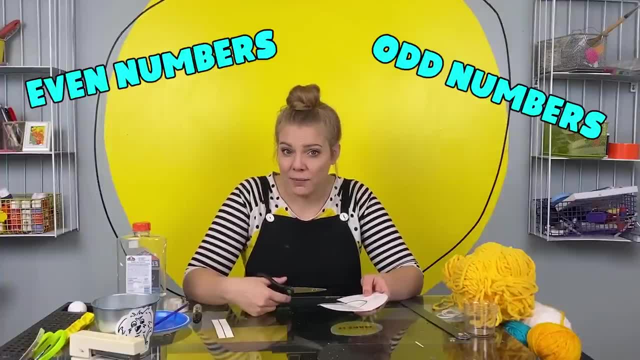 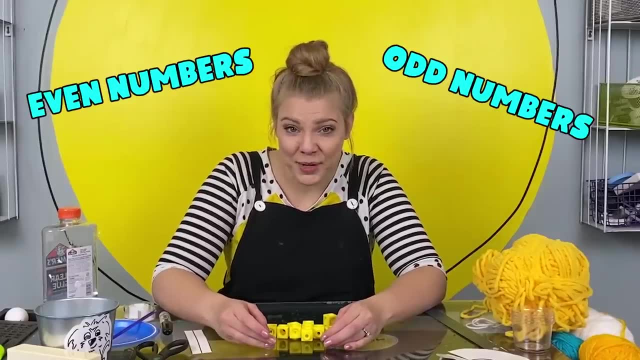 Do you know the difference between even numbers and odd numbers? Oh, Math break, Math break. Now I remember the difference between even and odd numbers If you stack them in a column of two, like everyone is holding hands with a friend, like this: 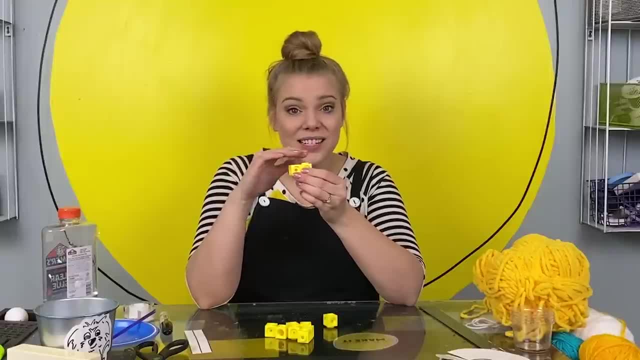 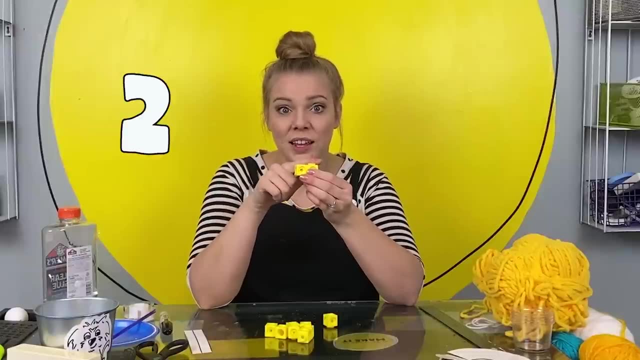 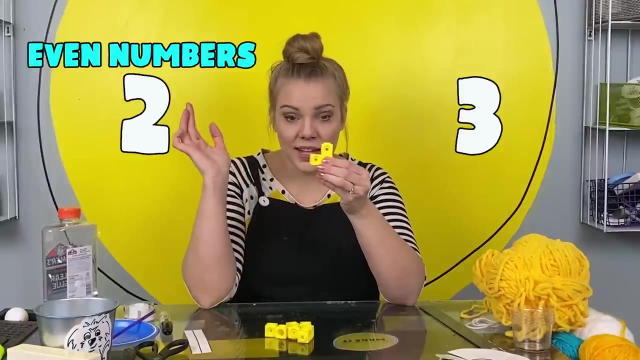 Is the top flat Or is the top even, Because even just means flat, smoothed out, totally level. Okay, so two, one, two is an even number, But three It's not. That's not even. That's a bumpy road. 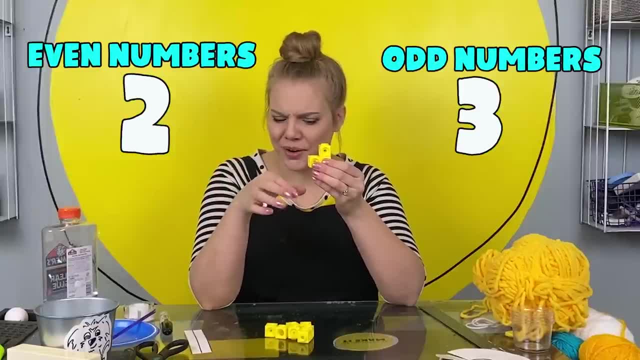 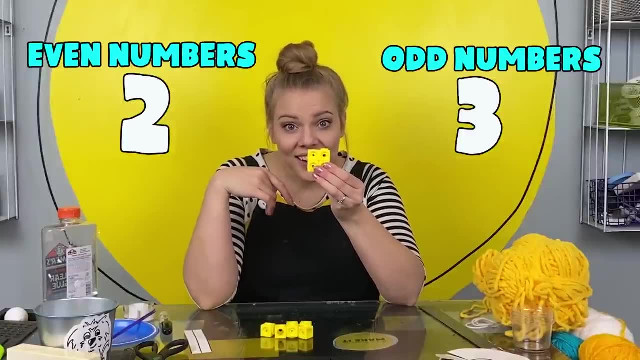 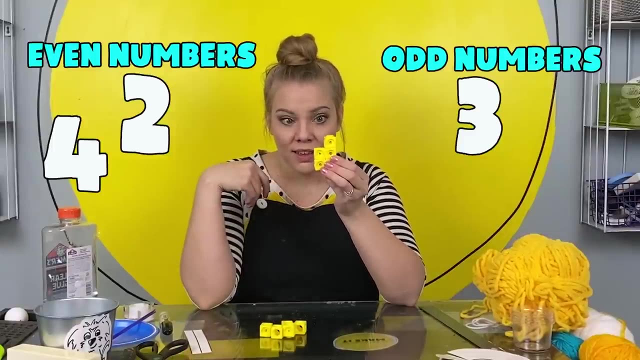 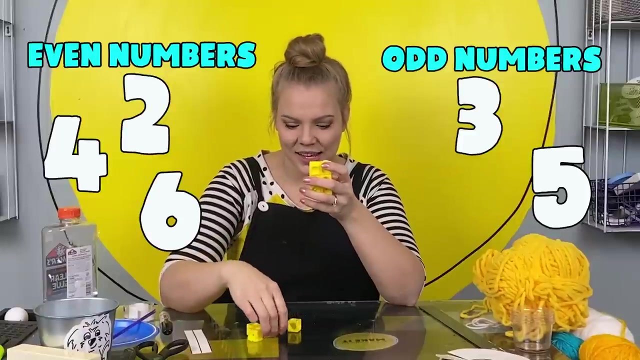 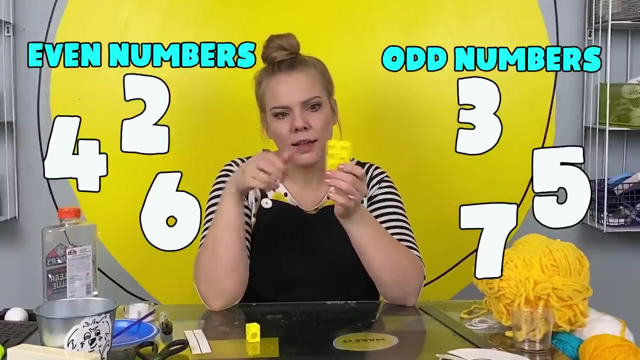 Three is an odd number, a unique number. How about four? Is the top flat or bumpy? It's flat. Four is an even number: Five Odd Six Even. Seven Odd, Eight, Even. Are you starting to get it? 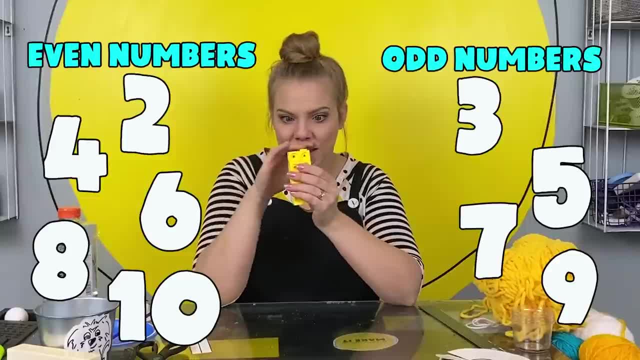 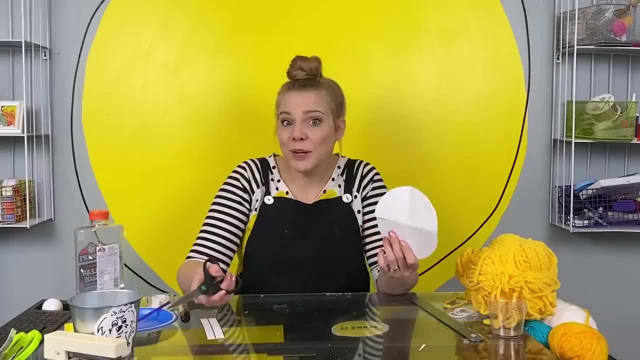 Nine Odd And ten Even. It just keeps going like that. Now you know the difference between odd and even numbers. The math break is over, So I'm going to cut an odd number of sections. When you get to the line we traced, stop cutting. 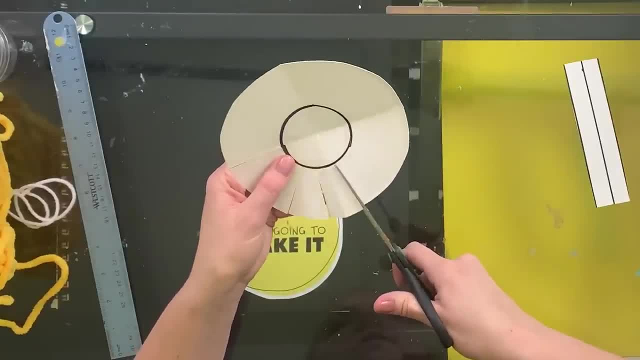 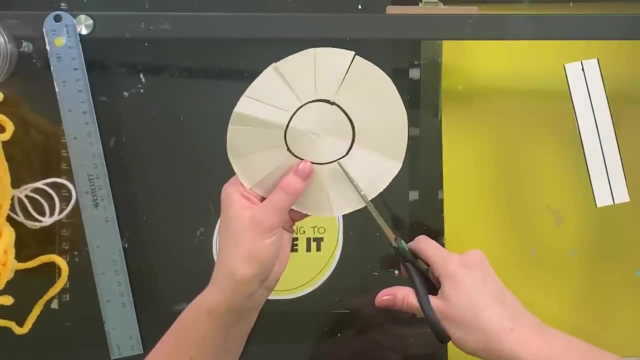 That area is protected by this line so that there's a bottom to our basket. You can use a ruler to measure these out, but you also don't have to. They don't have to be the same width all the way around. If they're different widths, that might even look kind of cool, because you would get a different design of your basket. 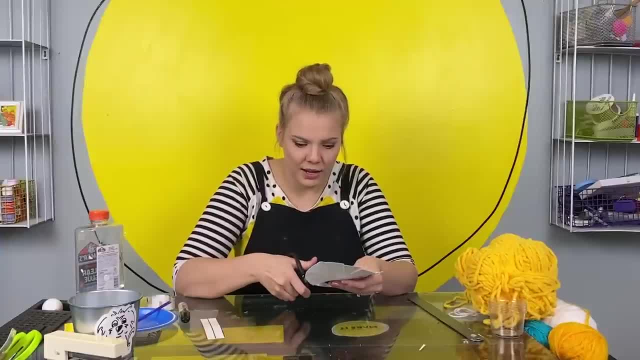 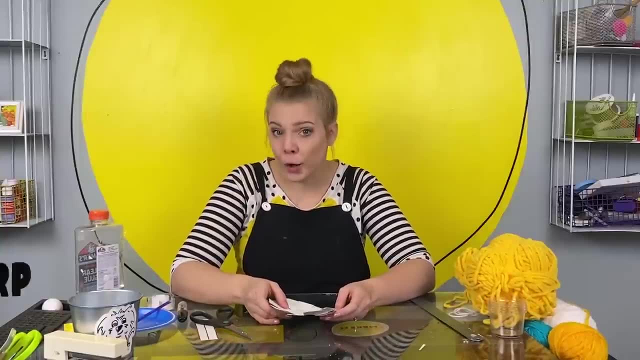 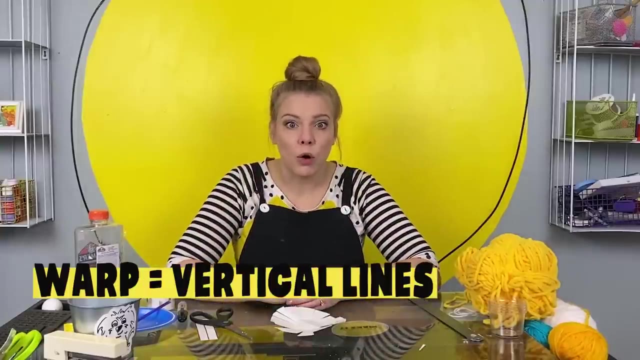 You get to pick Thirteen odd, So I need to make this one into two, So it's fourteen, fifteen. Those fifteen sections will end up being the wharf of the weave that we're making. The warp are the lines that go up and down or vertically in a woven thing. 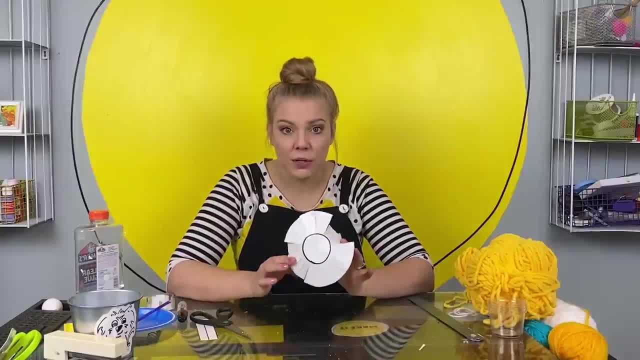 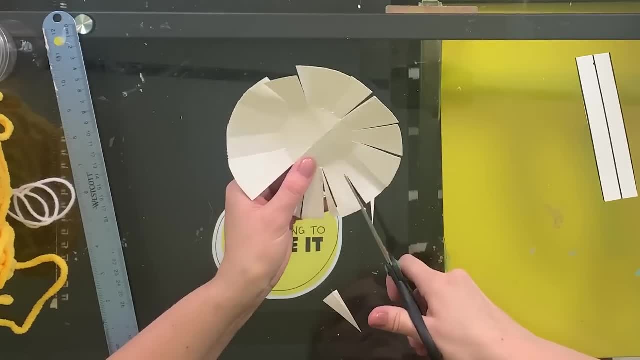 So we have fifteen warps for our basket. Our next step is to cut a little space between each section so that there's room for our yarn. I'm going to do that by cutting a little triangle, kind of like a pizza slice, between each section. 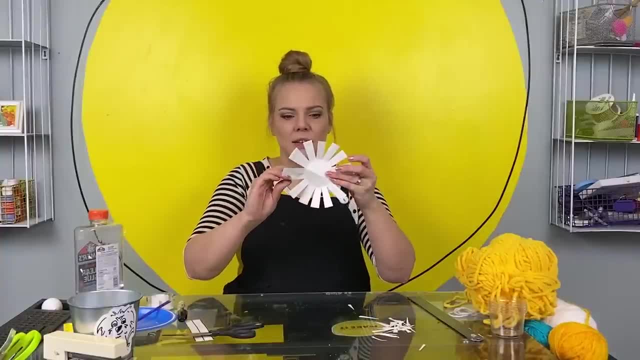 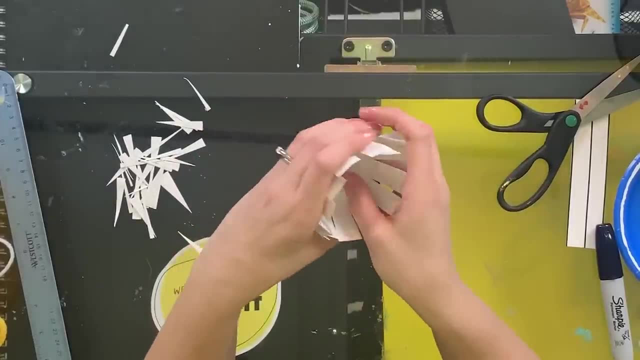 Wow, It kind of looks like a sun or a flower, doesn't it? Or, um, oh, a sunflower. Now you're going to be able to start to imagine the basket a little bit. The circle we traced is going to be the bottom. 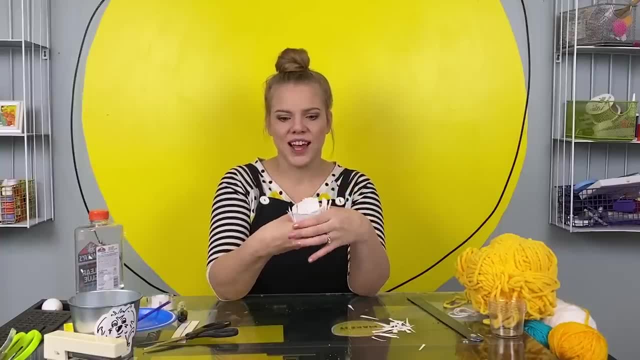 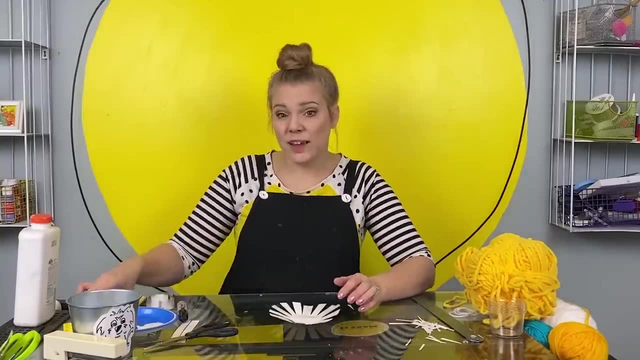 And these sections we cut, or the warps, are going to be the sides. See, Before we get weaving, I'm going to decorate the very bottom of my basket, which definitely can be woven, but that's not what we're doing here today. 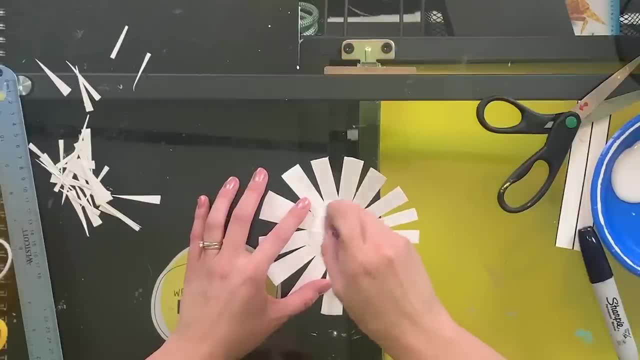 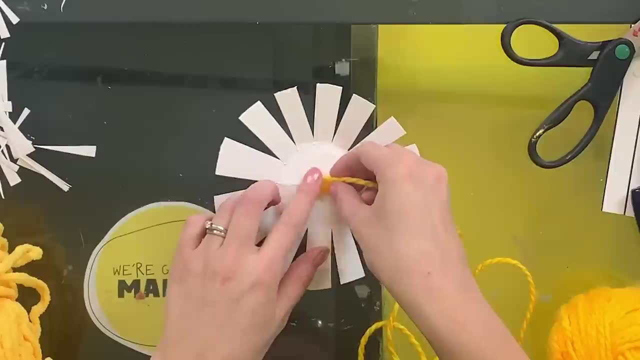 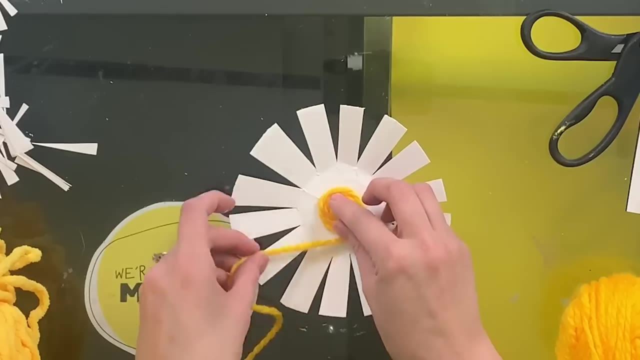 So I'm just going to add some yarn with glue. I'm going to start by making a little twirl And putting it in the very bottom Center. I already put my glue down so this sticks. Then I'm going to keep wrapping this in a coil, kind of like a snail. 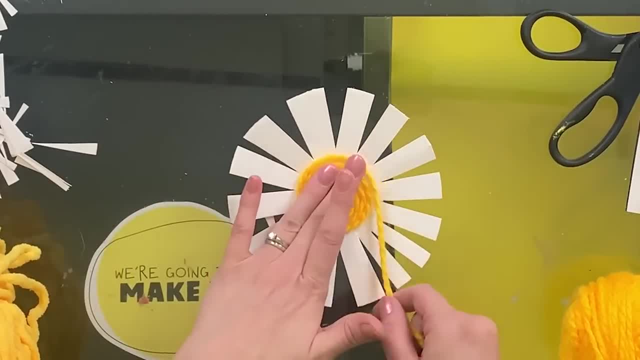 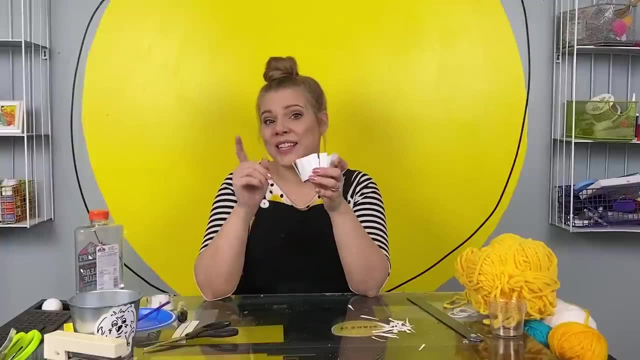 all the way until the bottom of my basket is covered. Once that's done, you just need to cut it. That glue will dry and hold it right in place. Now we're going to add some yarn. This is what's going to hold all of these sections together. 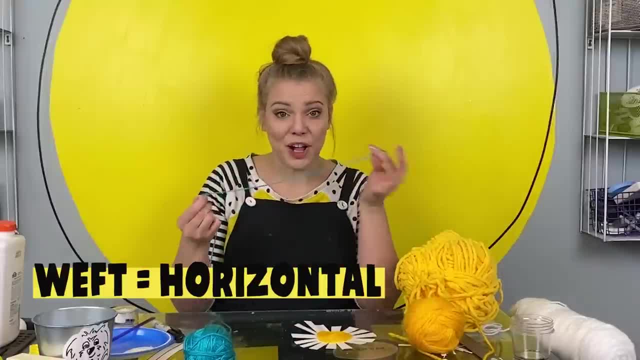 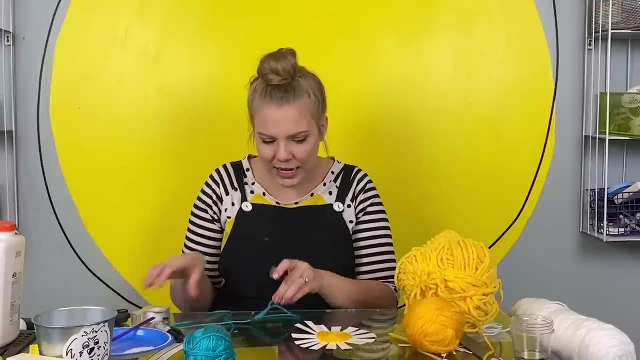 This is what's called the weft. Find whatever color, string, yarn, ribbon, whatever you're using you want to start with, And just to make it a little easier to hold, I'm going to tape this down. Then we're going to start weaving. 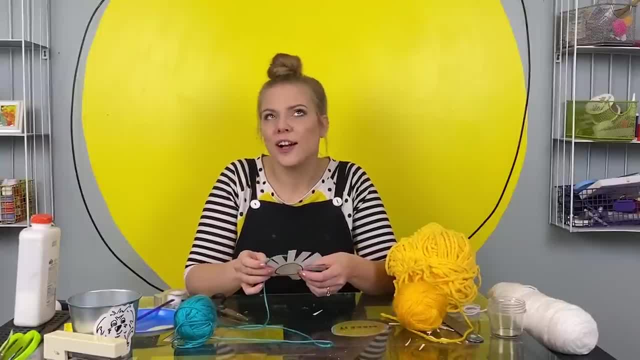 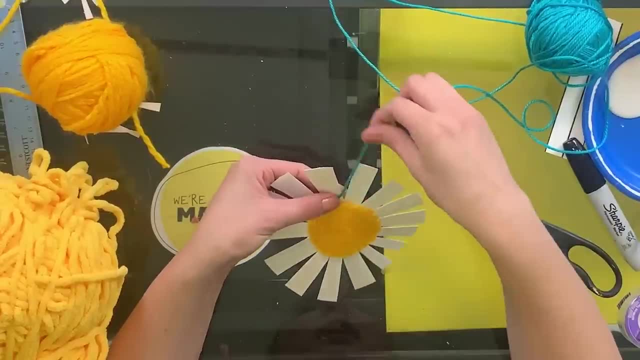 The pattern that we're going to be using today is just over under, over under, over under, Yes, Over Under. You get it This one's over, so for our next one, we're just going to go under. 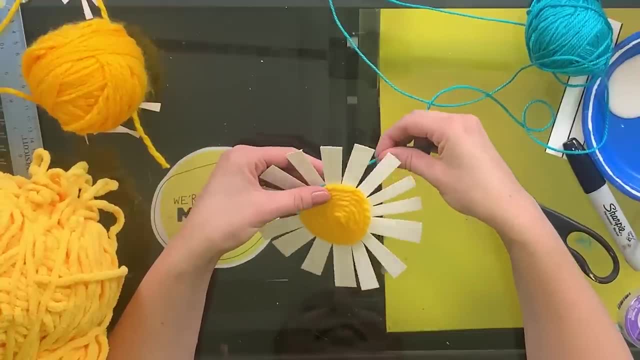 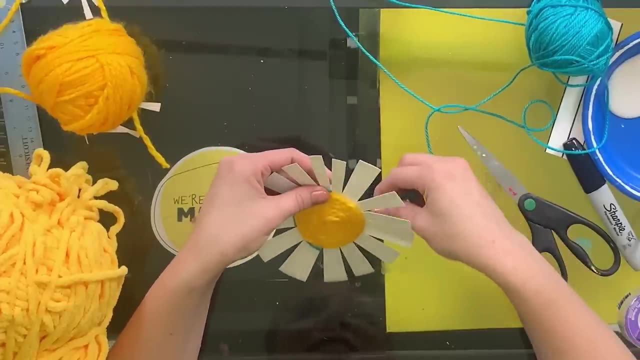 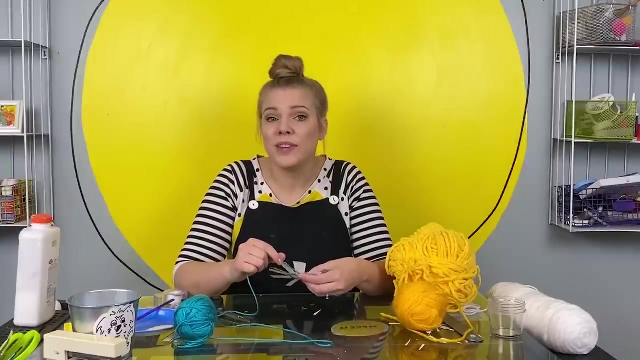 Over Under, Getting it Over, Under, Over Under. Now you get to decide if you want to keep going with that color or switch it up. You can make whatever kind of design you want. I'm going to do a couple more rounds with this teal color. 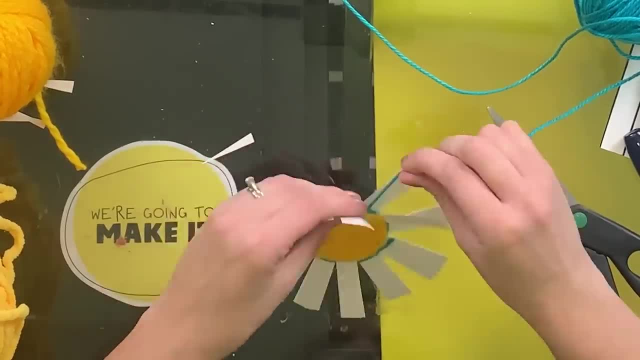 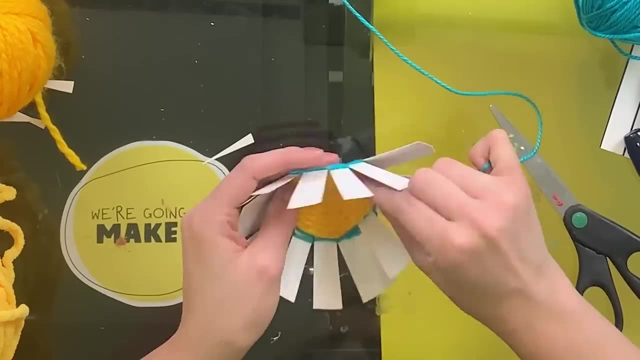 For the first couple rows it's okay to do this flat, But as you start getting closer you're going to start lifting those warps up so that your weft can start holding it up into a basket shape instead of just a flat plate shape or something. 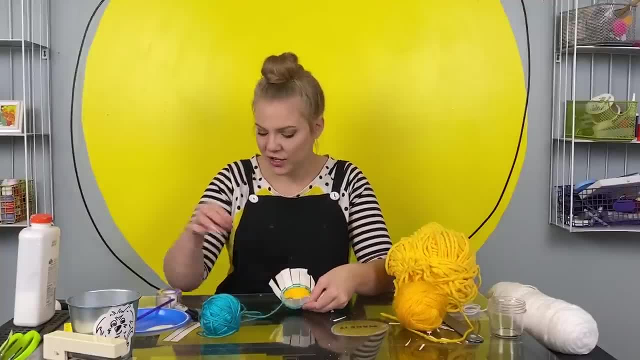 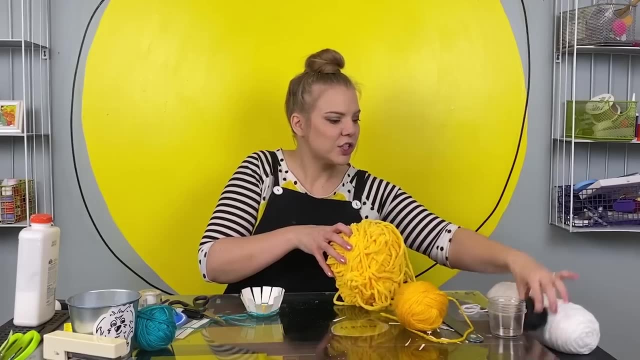 I love it And I think it's time for me to switch colors. To do that, I'm just going to cut my yarn off And I'm just going to secure the end with a little bit of tape again And then switch. 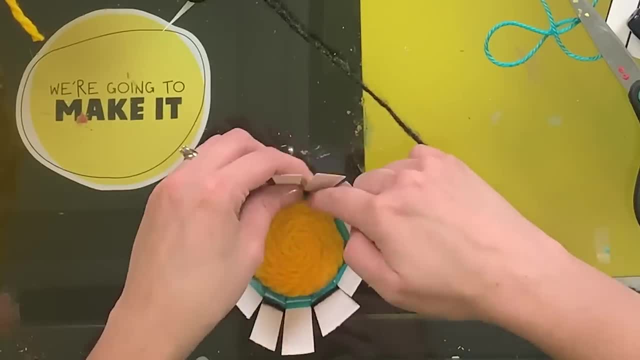 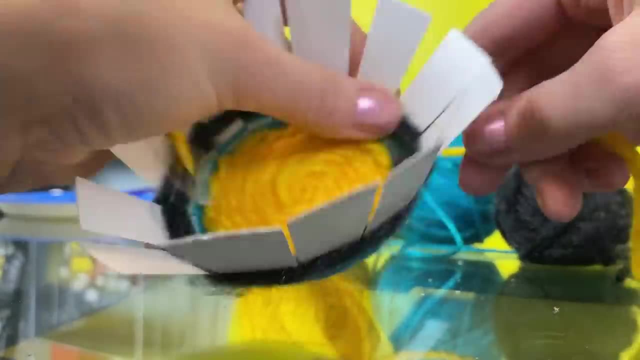 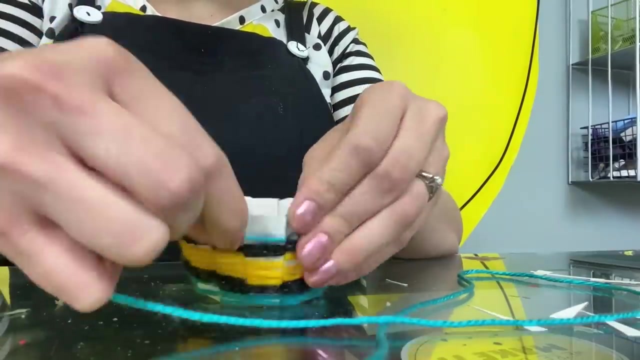 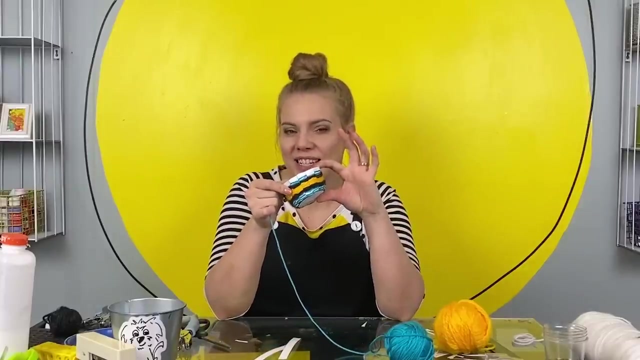 I'm going to try this dark gray Once you've filled up your warps almost all the way to the top. we're going to do something a little different. We're going to punch some holes in the top so we can make a decoration around the top edge. 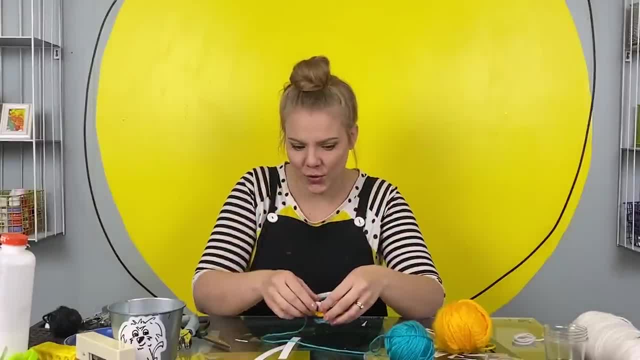 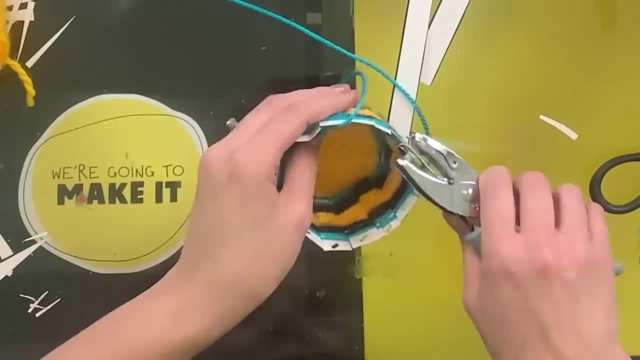 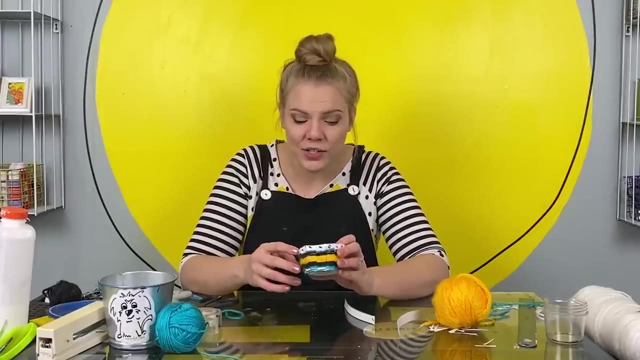 And we're going to add on our handles. So let's start with our hole punches. Now that our holes are punched, we're about to put our handles on, So the first thing I'm going to do is take care of these extra ends. 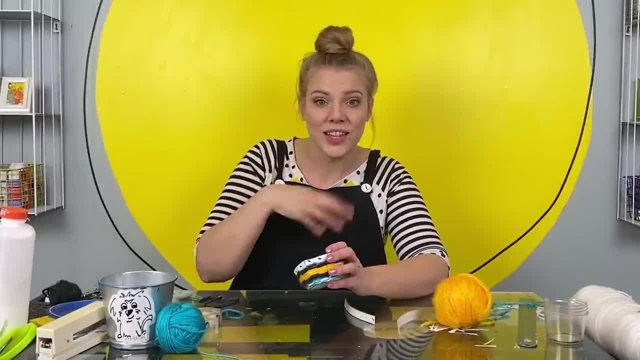 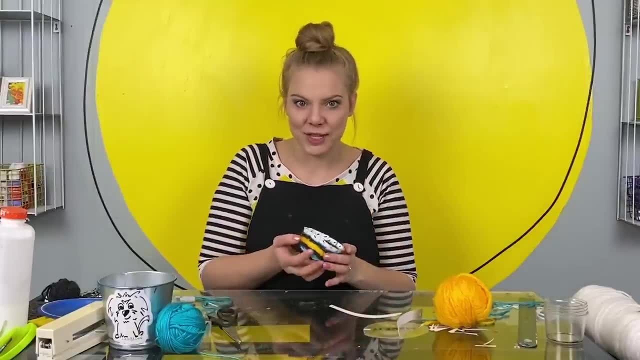 And how you're going to do that is, you're just going to tuck them under the weave so that they stay nice and hidden, and it looks really neat. There we go: Time to attach our handle and to make a cool design around the edge of this basket. 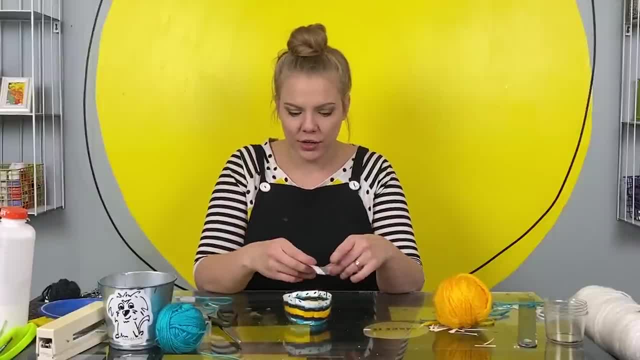 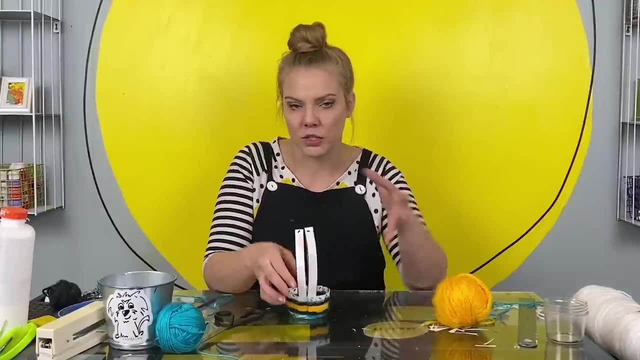 First thing you need to do is decide where you want your handle to go And then glue them down to the inside. We're going to use yarn to secure these two, but gluing them just helps you hold everything, so you're not all. 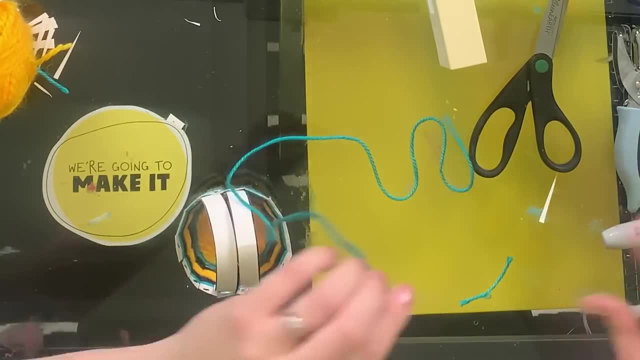 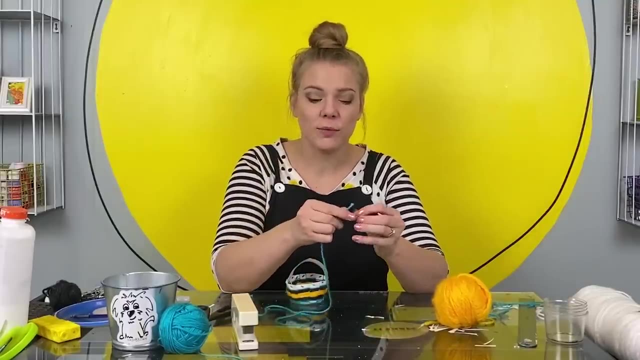 Now that your handles are attached, you just need some string. Now that your handles are attached, you're going to thread some yarn through the holes that we punched. Yarn gets really frayed on the ends. That means all the little pieces go everywhere. 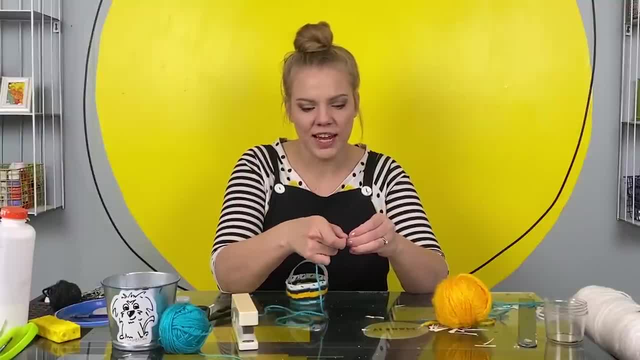 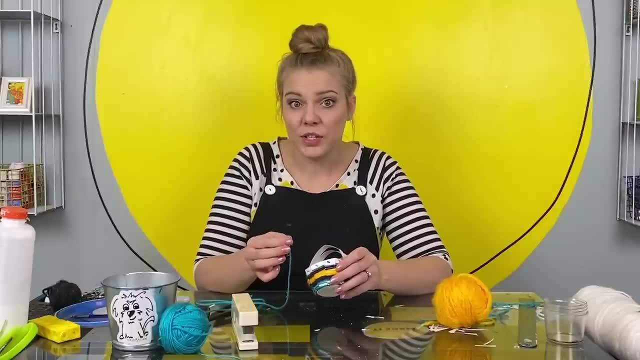 which can make it really hard to thread. So I'm going to put a little bit of tape around the end of my yarn. It's a temporary threading needle For every part of this design. I'm going to start from the inside and go out. 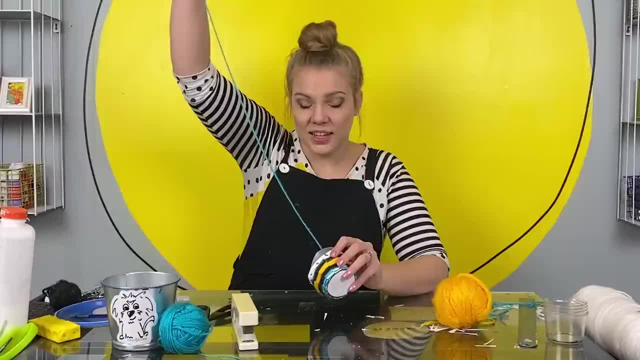 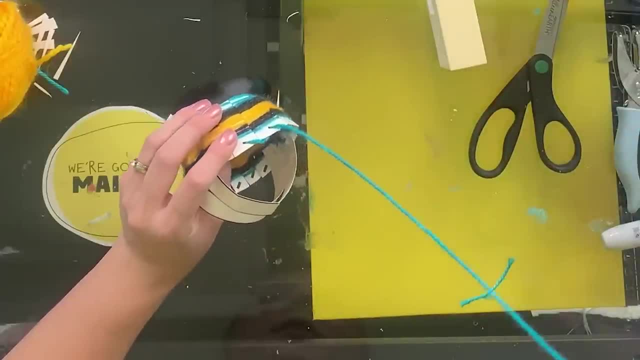 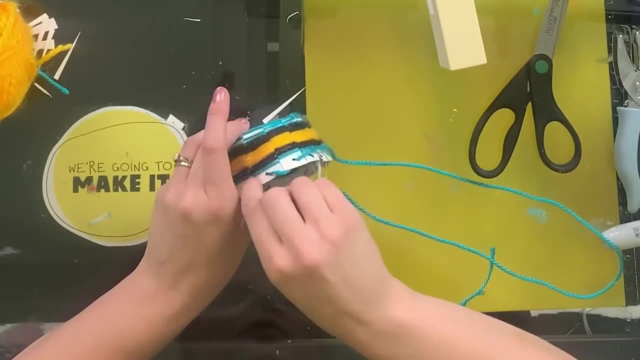 So inside out, Then I'm going to bring it up, go inside out. I'm not going to pull this really tight. I don't actually need it to hold anything. It's just a design. See that little twirly design it's making on top. 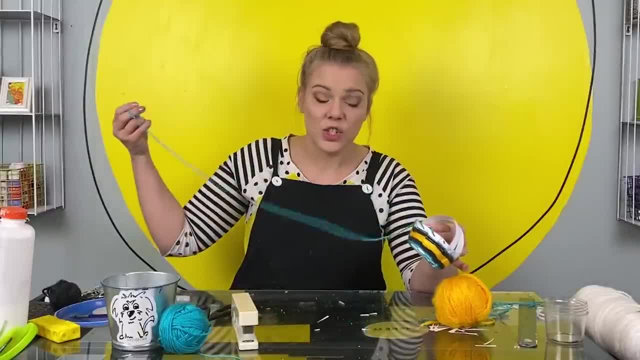 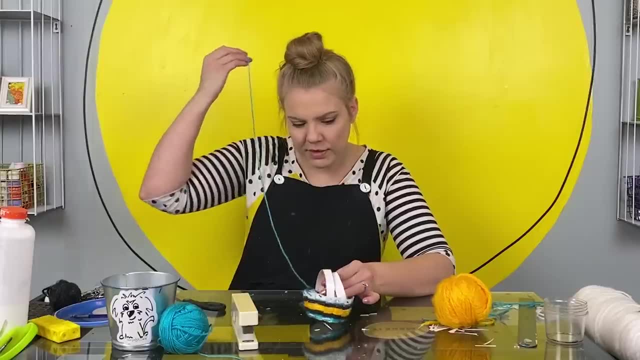 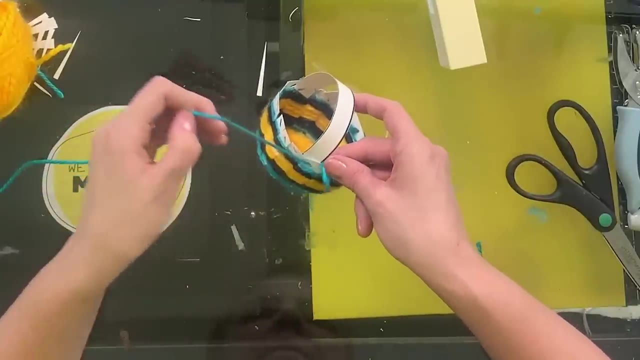 Cool, When you get to the handles, just do the same thing: Go through the hole that you punched in your handle, Then go between to go back in And then just right through that hole again. Keep going All the way around. 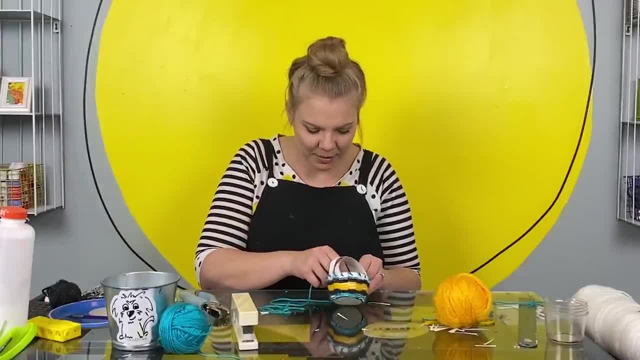 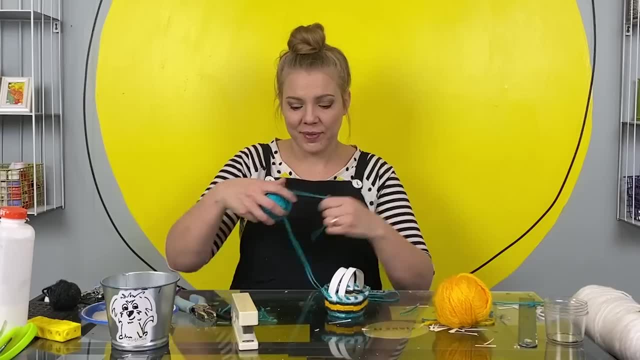 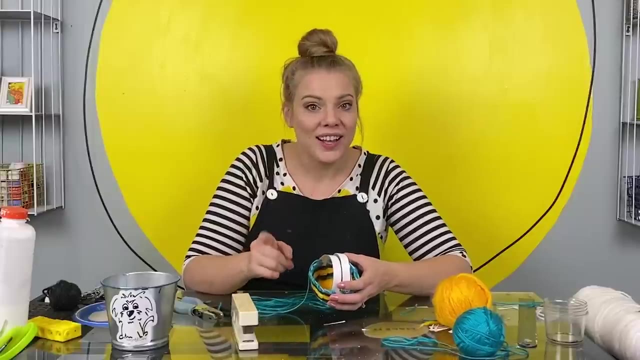 I decided to go around one more time on my top just because I want to double up that cool looking design. Our basket is looking awesome. Just one step left and it's to weave the handle. I'm going to use a pattern again. that's just over under, over under. 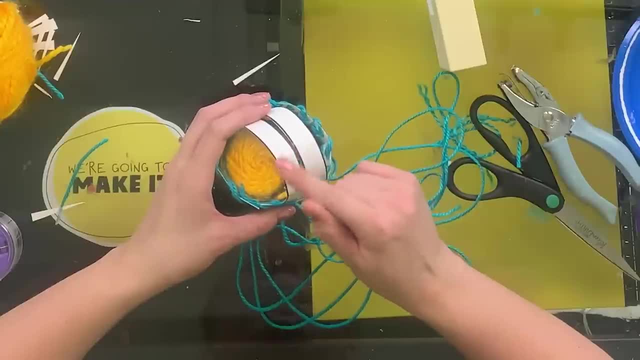 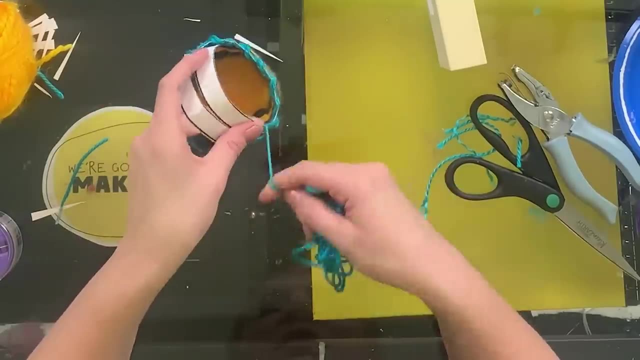 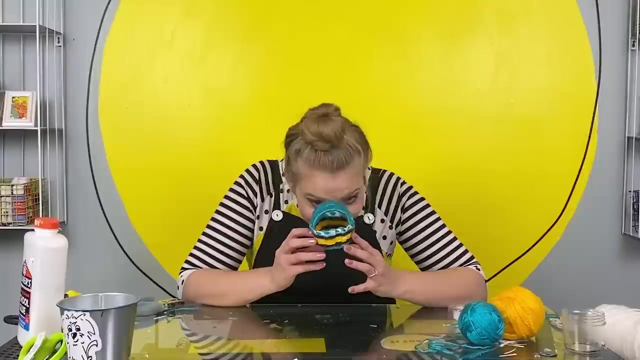 But there's only two, So I'm just going to be going back and forth, back and forth, back and forth until I reach the other side Over Under. Our basket is done. I love it. Is it perfect? No way. 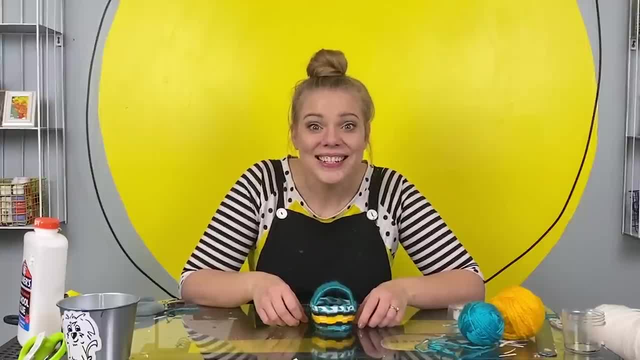 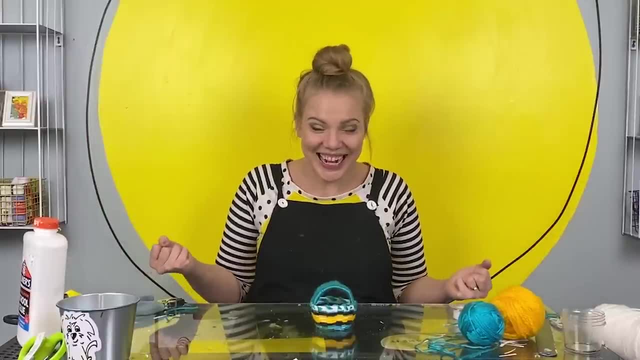 But that's what makes it special, And special enough to carry the first flower of spring. I'm so excited. Maybe you want to make a basket at home, but you don't have any flowers around, Or maybe when you're watching this, it's winter time. 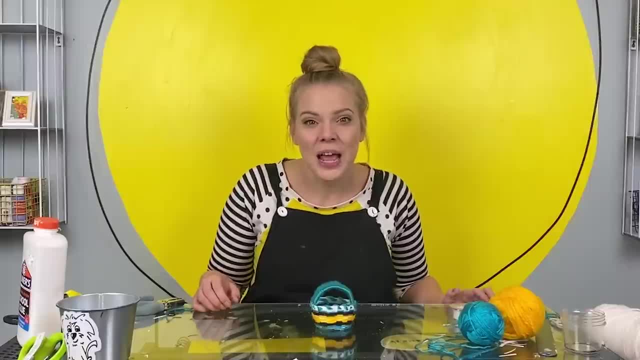 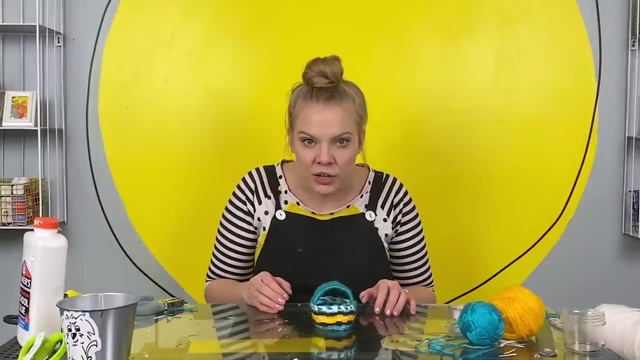 Where are you supposed to get a spring flower? Don't worry, A basket like this can have many purposes. Maybe you want to make your own. Maybe you put one of the coolest rocks from your rock collection in here, Or something very special that someone gave you. 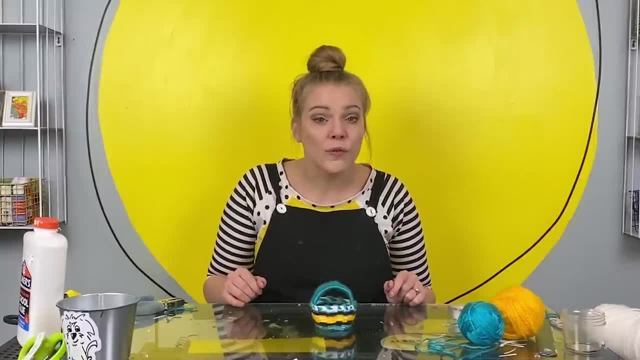 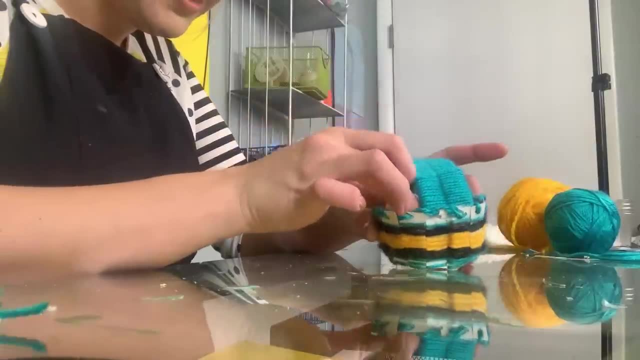 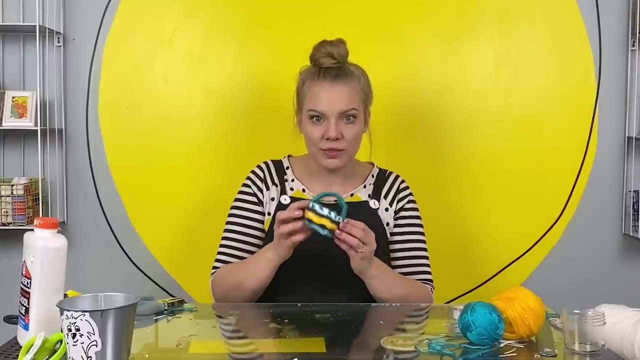 Maybe your favorite little toy. Or if your family celebrates Easter in the spring, maybe this would be the perfect place for an Easter egg. Oh yeah, That would totally work. But for us today this is a special flower carrier. Let's go. 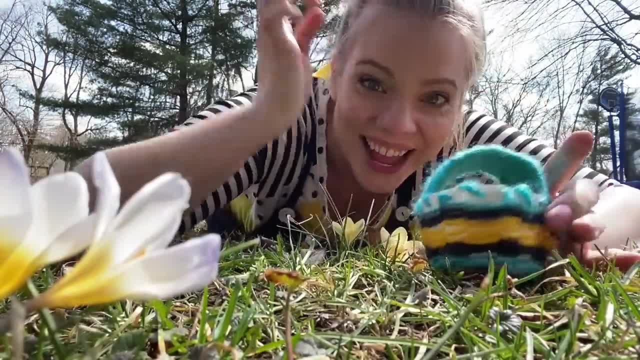 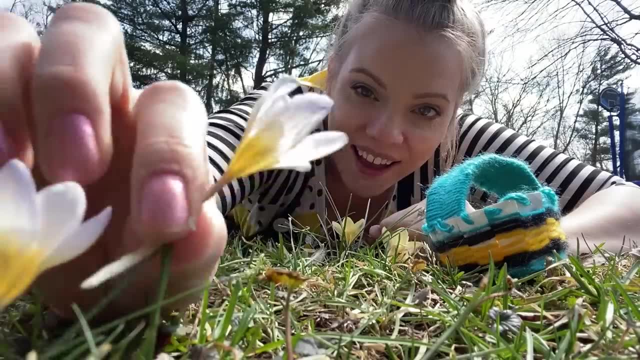 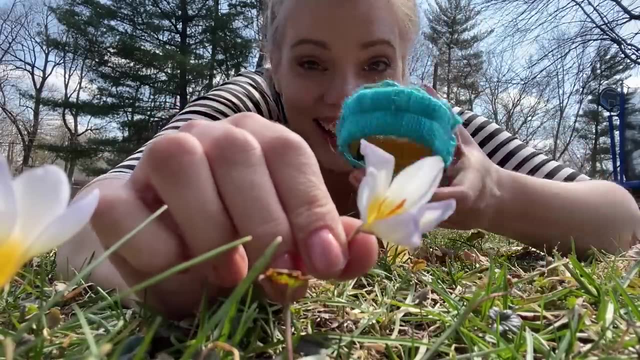 You beat me. Okay, Got my basket, Got our flowers Ready. Okay, Look, Isn't it beautiful? Yeah, Okay, Got our basket, Got our flower Perfect. I loved making this one. I love it. I love it. 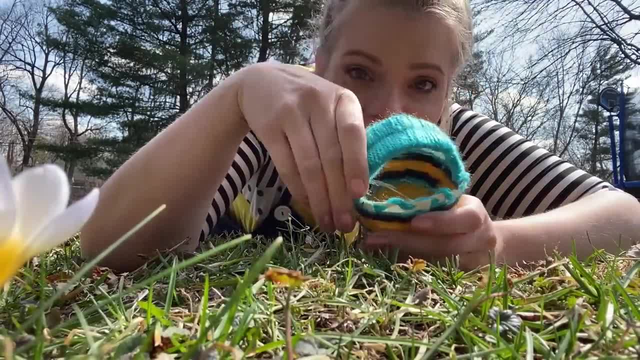 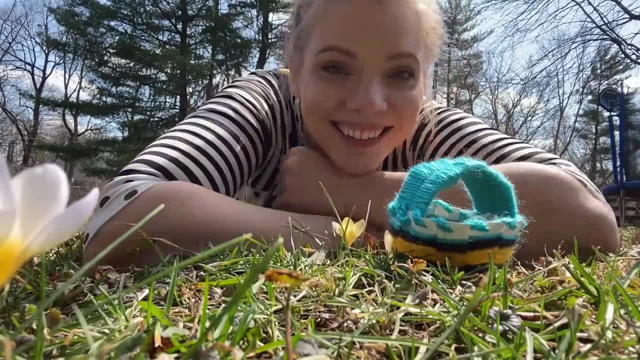 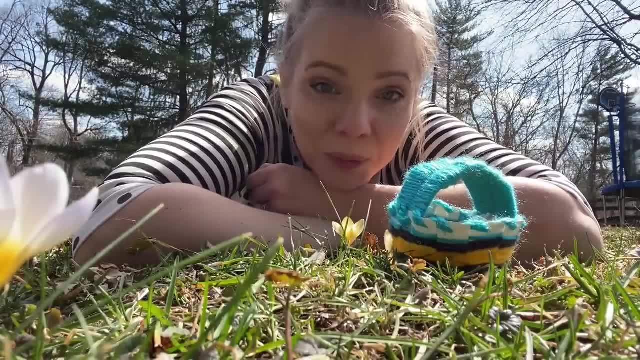 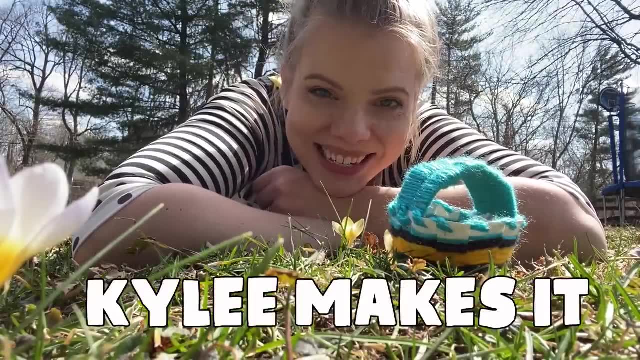 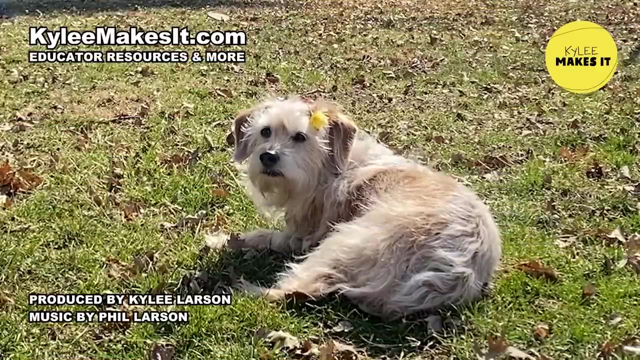 I loved our basket. I love spring And I love when we get to hang out. If you want to make more of it art with me, just search for Kylie Makes It K-Y-L-E-E. That's me. See you next time.